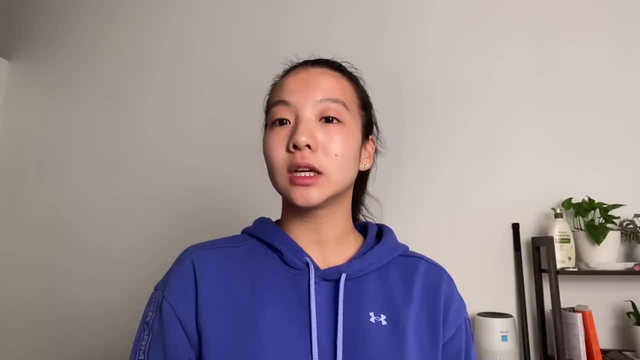 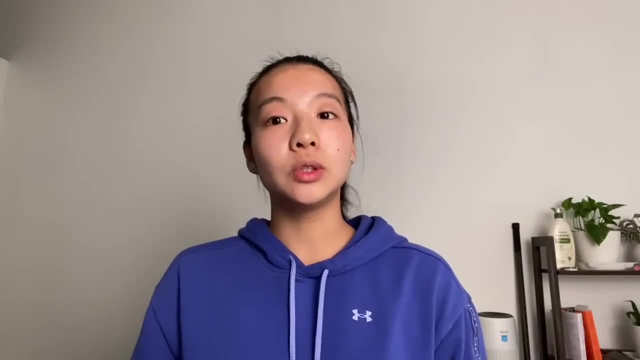 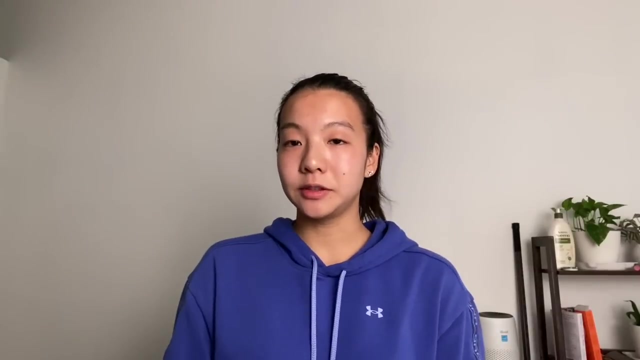 parts about finding a job as a software engineer is the technical interview. During these programming related interviews, the interviewer will expect you to work to a solution, optimize it and write code or pseudocode on the spot. The reasoning behind these interviews is that they will help. 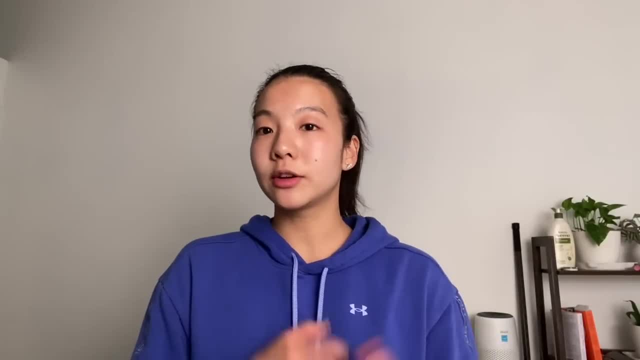 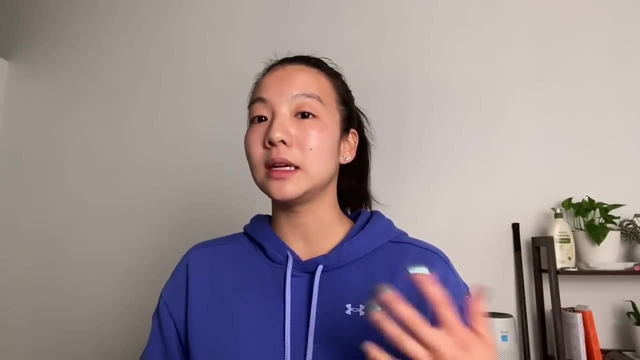 the interviewer. understand your ability to understand the problem, ask questions, go deeper and optimize the solution. How much do you understand data structures and how much do you need to know to solve a problem? How much do you need to know to solve a problem? 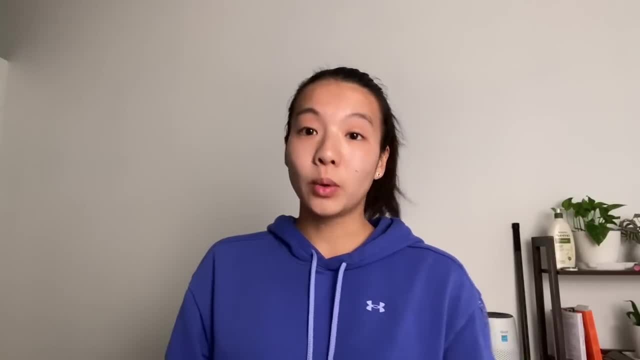 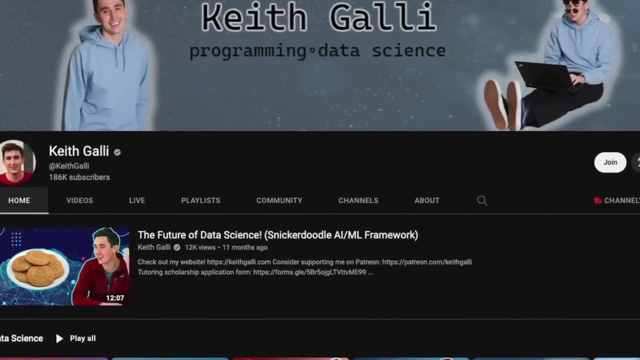 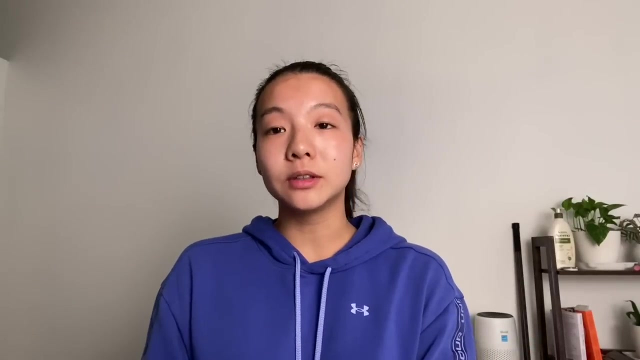 and algorithms and, ultimately, what is your coding level and what is your coding ability. today i paired up with a good friend of mine, keith galley, who has a data science focused youtube channel, and he is going to be mock interviewing me, so this interview might look like what a real software. 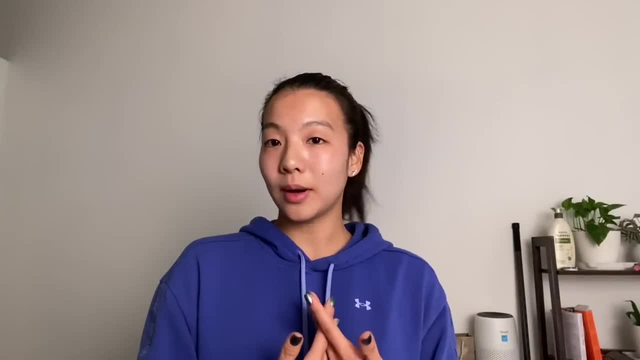 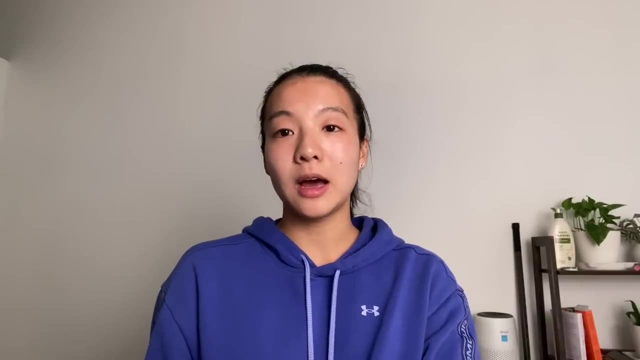 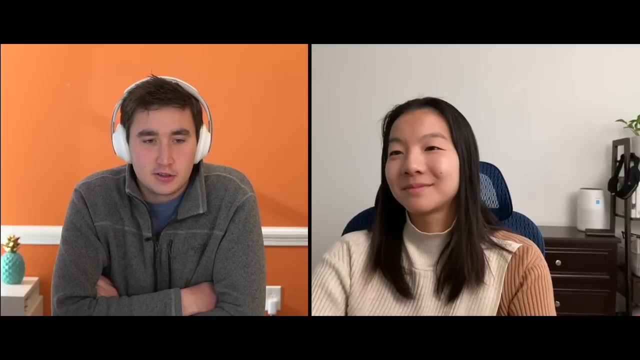 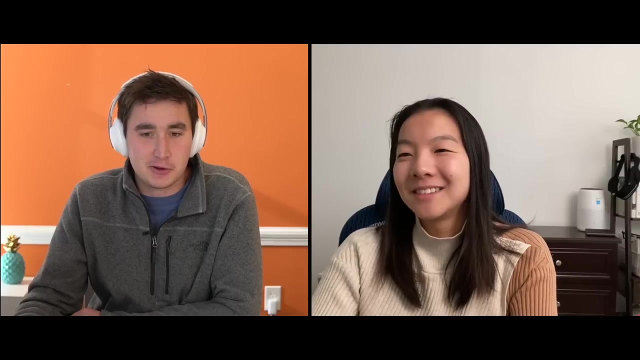 engineering interview looks like i don't know what question he's going to ask, so it's going to be as much of a surprise to me as it is to you, and i will be coding on the spot. so here we go. welcome, uh, welcome to the interview. how are you doing, uh, today? i'm good. how are you? i'm doing? 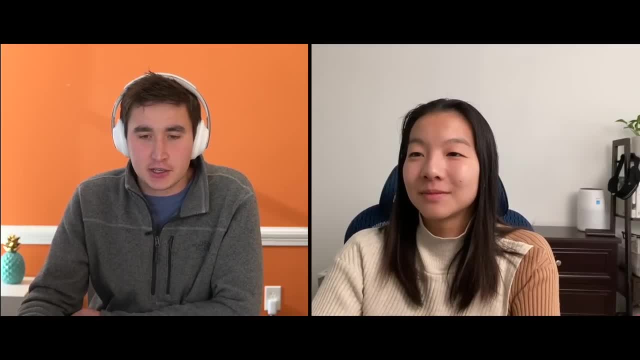 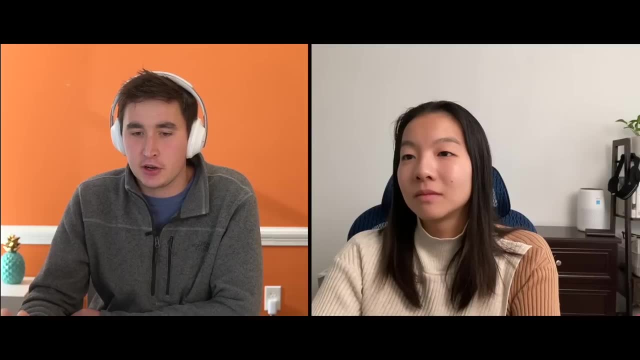 pretty well. um, we're gonna probably just jump right into this interview. i'm just curious: are you familiar with coder pad? because that's what we're gonna be using throughout. i think it might be easiest to kind of share code. yeah, cool, all right, so we're gonna kind of just jump. 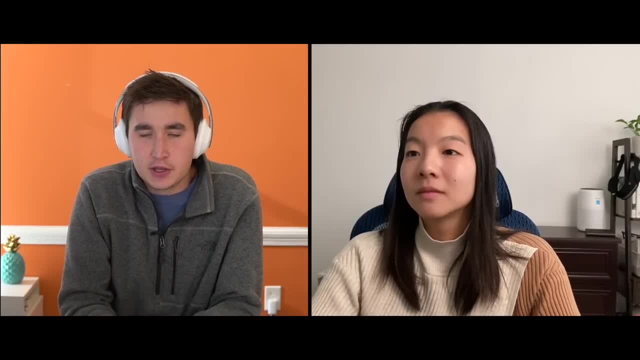 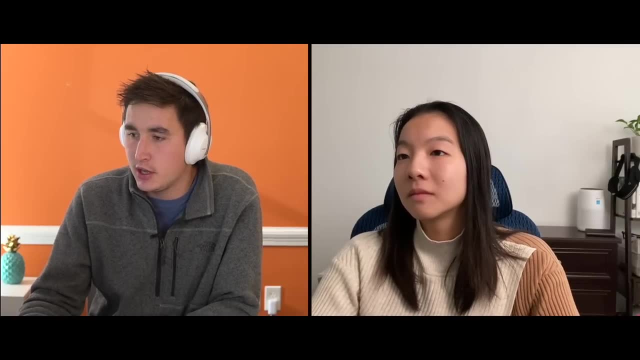 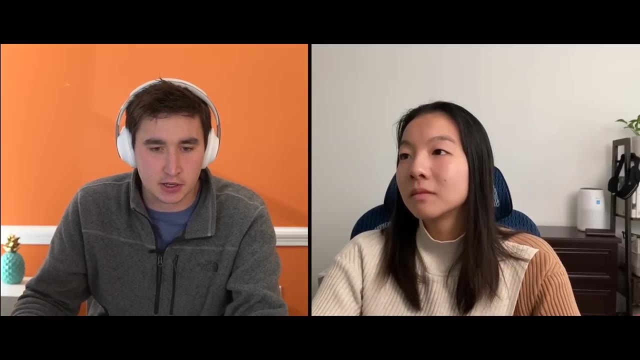 right into the the problem. so for the purpose of this problem and let me share, i just want to make sure you can access this coder link. so i'm going to share this and i recommend maybe sharing your screen- or i guess we also can just work off of this- so i should be able to see here what you 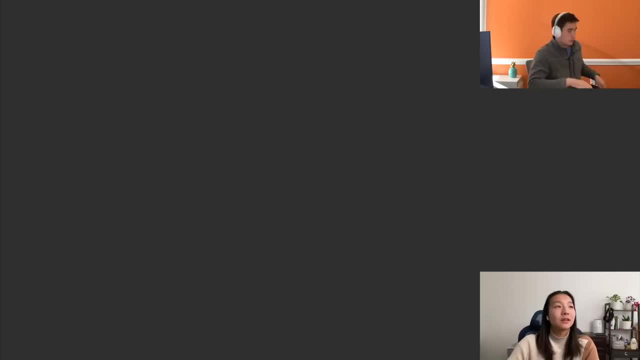 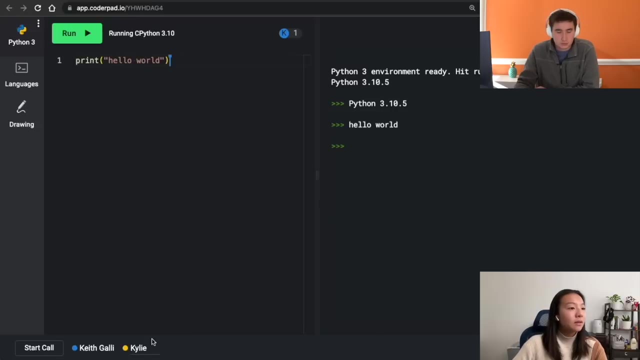 type in si open the chat. i can click on this link and it will take me to the coder pad. i name is kylie and i will enter, and so so i can see that you're going to enter an apt cue. you're at the top of the bar. you can get us back to it, so i'm going to go and share and it might be just a very 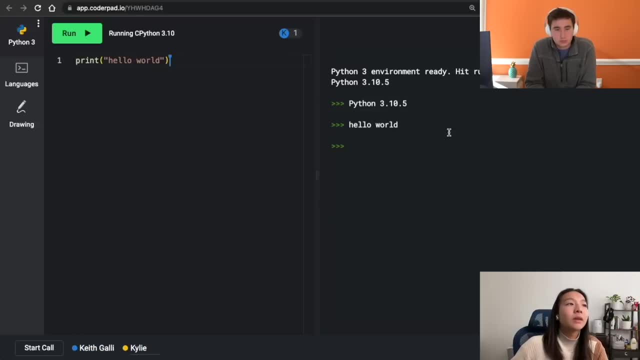 you're in this coder pad as well, and then here i am. yep, and just to make sure that you're comfortable here, you want to just run like a couple simple lines of code. you can try just running this: print: hello world, if you want. yeah, so if i run this, it'll say that i ran a line of python. it prints: 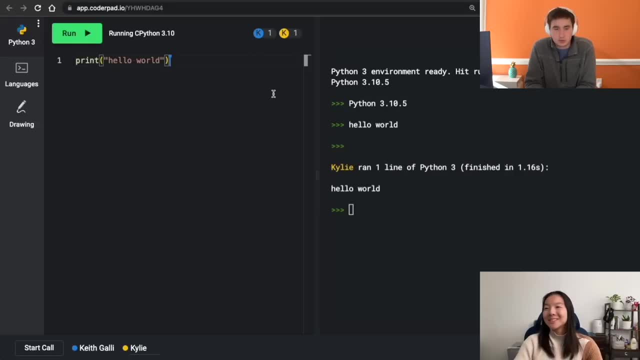 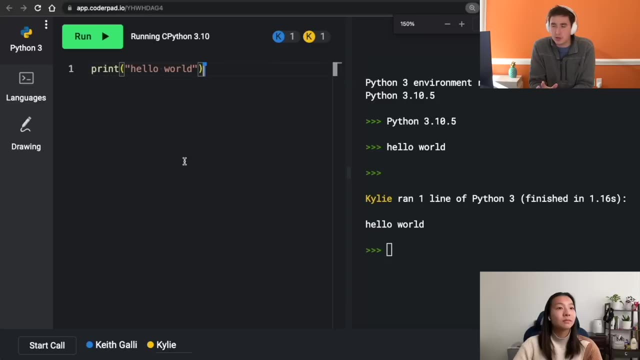 out hello world, so i think it works perfect. okay, so let's uh kind of jump into the problem. so, just to give you some context, we're going to start with about 20 minutes of design- object oriented design, however you want to design this code- and then we'll spend probably the last 20. 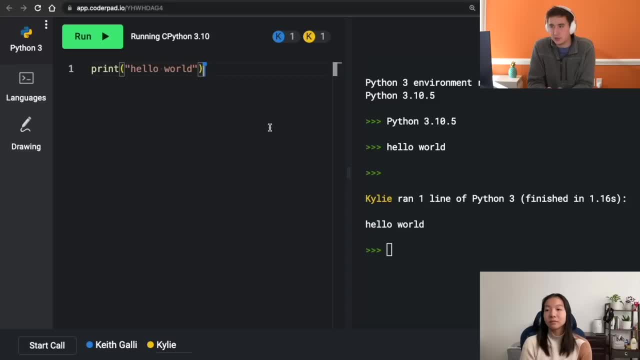 minutes working on more of an algorithms question. so that gives you just a little bit of a scope. you don't necessarily have to accomplish everything, you know. i know that we have limited time, but to kind of give you the context of the problem, imagine that we're designing a. 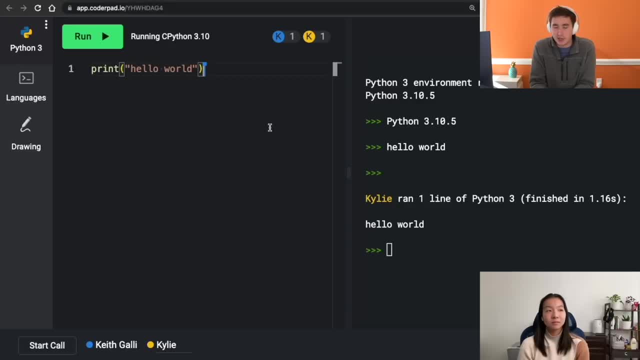 book system, so an online cloud reading application, and you can pretty much imagine that we're building a product that is similar to an amazon kindle, but specifically for short stories. so we're kind of in our own niche. they might be indie stories, they might not be, you know, found anywhere. 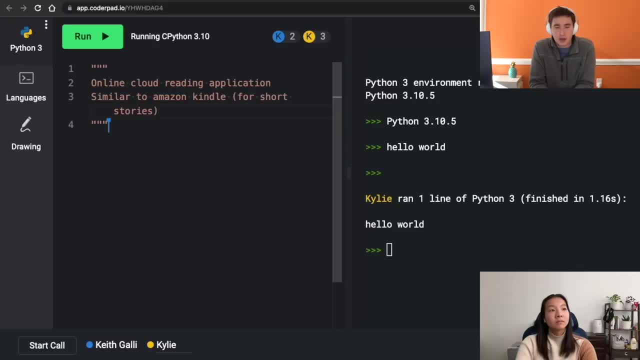 else people could add their own stories and basically, what we want to do to start this problem off is that we need help designing the actual application, we need to help designing the code that could implement an online cloud reading application, and there's a couple things that we're looking for, and this is very open-ended. 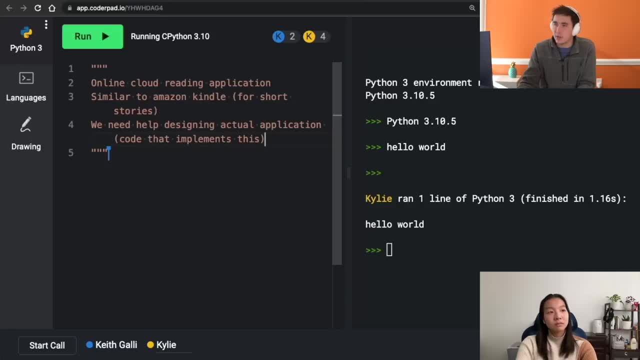 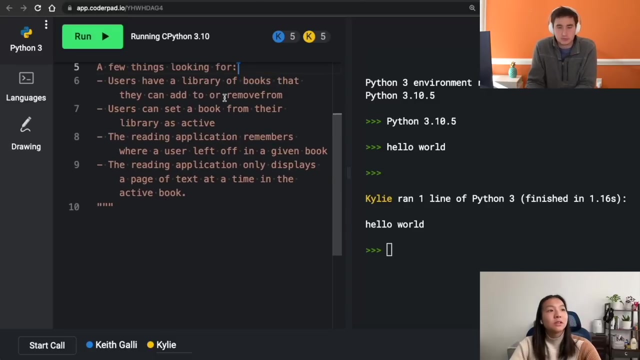 you can implement this how you want. but a few things, and i'll paste these into the coder pad that we're looking for. i'll just paste it below: um, oh yeah, okay, you can fix this up and i'll delete it, that top line, okay. so a few things that you're looking for. users have a library of books that 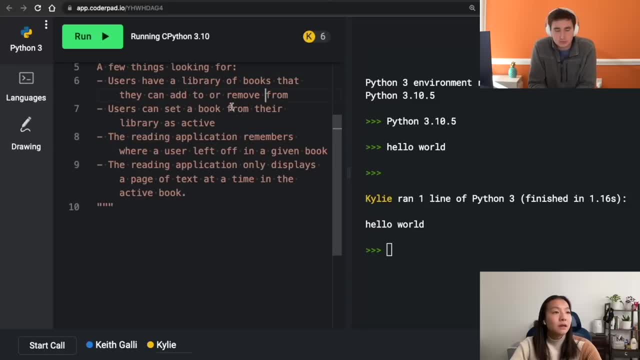 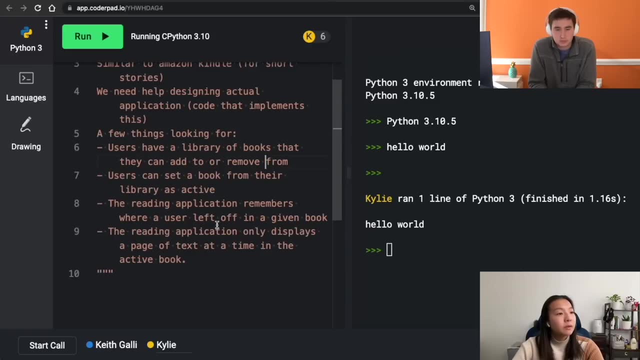 they can add to or remove from. users can set a book from their library as active. the reading application remembers where a user left off in a given book and the reading application only displays a page of text at a time in the app, in the active book. exactly, awesome, um so. 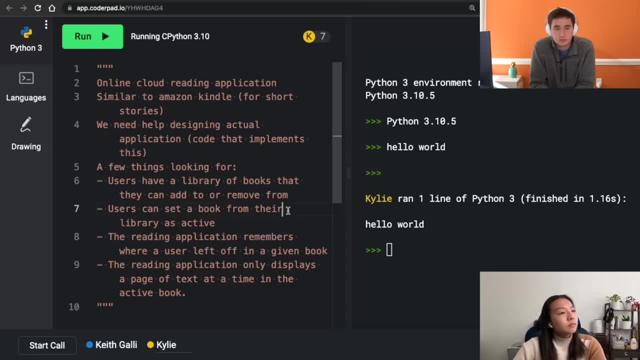 so let's see, essentially what we want to do is create a library where users can interact with this library. they can look at a book and set it as active and then, um, this application will also just remember where they left off and display whatever page that they're currently looking at in the active book. 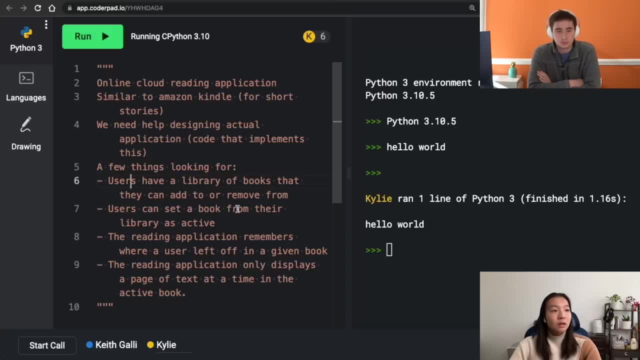 exactly, correct, correct, correct, okay. and then, more specifically, do you want me to kind of give like a high level implementation or um, how do you want me to start this? so i really want to just think about you know what components would it be important? this is, i would say, an object-oriented 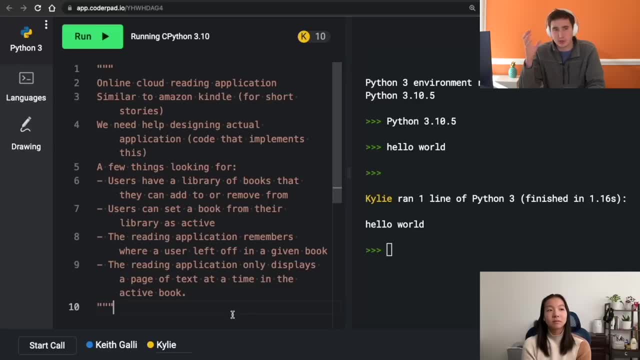 design question. so i'm just thinking about how you would think about structuring, uh, i guess, the base of a program like this. so obviously we're not going to build this full application, but i'm really curious about how you're structuring that kind of that core structure, that core um foundation, right? so let me 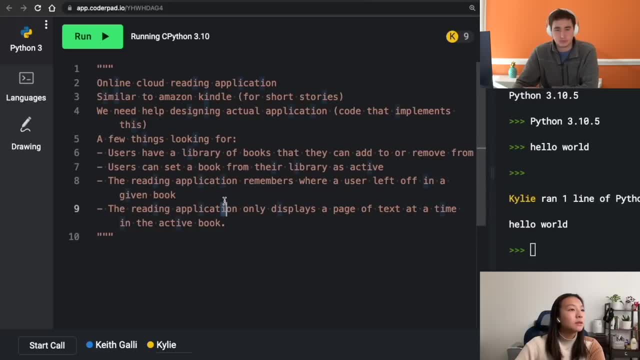 make this, uh, smaller over on this end, so people can see all of this and let's type up some more notes. so, uh, the things that jump out to me are that you need to be able to remember all books. so if i type this, we need to have all books in the library and we need to 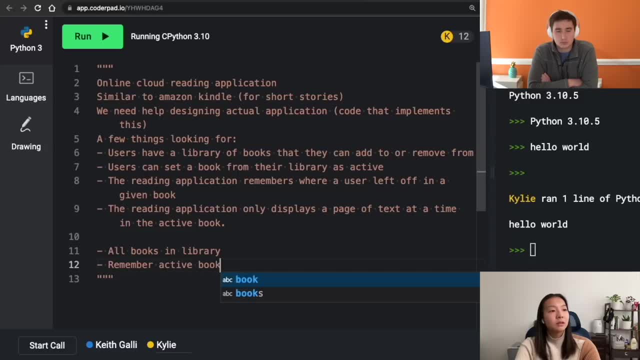 um, remember active book. and then we want to remember page. uh, remember page, i guess last pages in all books. and then we want to uh, display a page in active book. okay, so, um, by this, all books in the library. is that more so, i guess? how are we representing these books? are we? are they just like strings do? 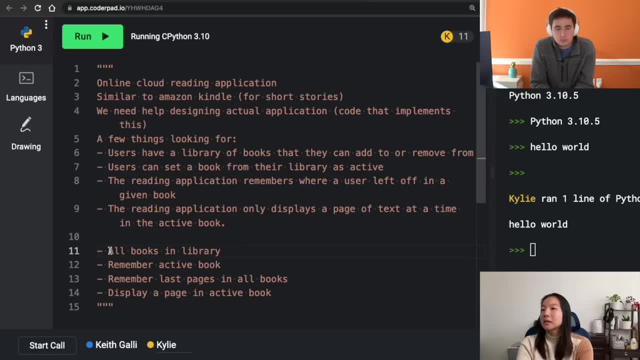 they have a page number and then the string of text. how is that formatted? is it like html? i think it's up to you how you want to um store the books within, like this programming structure, so you can kind of decide what makes sense. um, for that i think the important things is the actual. 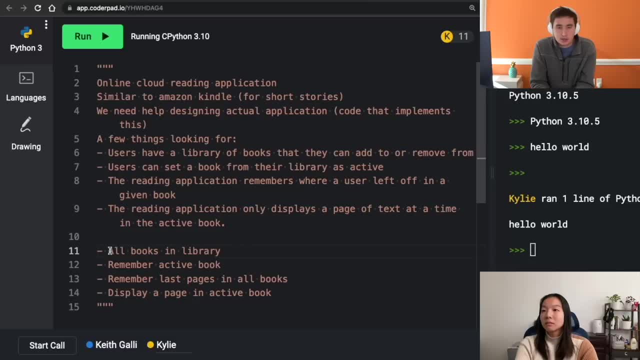 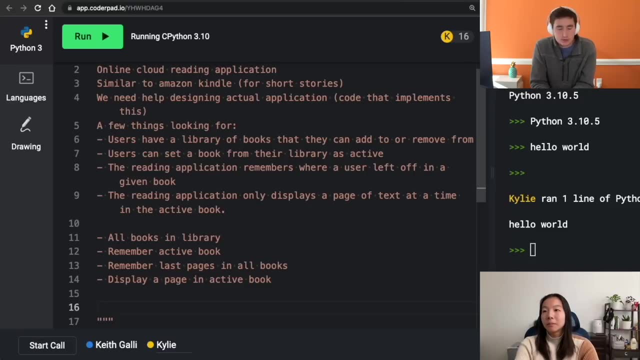 text of the book, as well as the title of the book, uh, okay, and, and you can implement the- uh, the details of, like the pages and all of that, yeah, yeah, okay. so i think that there's two things that jump out to me here. right, it's, we need one class. we want one class representing 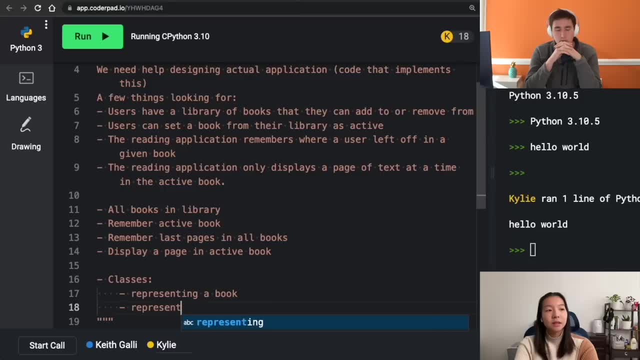 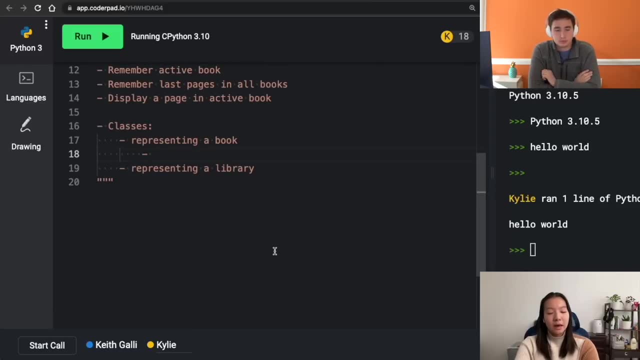 a book, and then we want another class, perhaps representing a library, so a collection of books, books, and so in this book specifically, you just mentioned that we want the title as well as the like pages in the book, yep, or like I could rename that, the content, yep, exactly in the book. and then for the library, we have a collection of 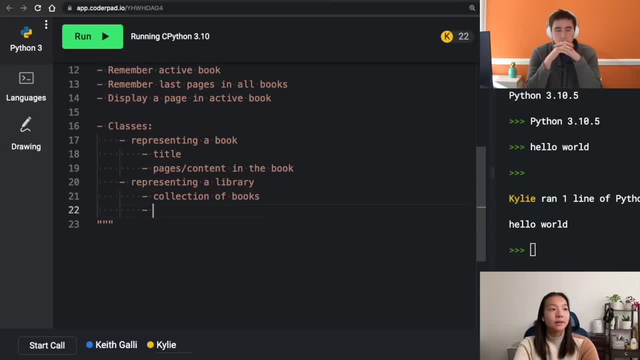 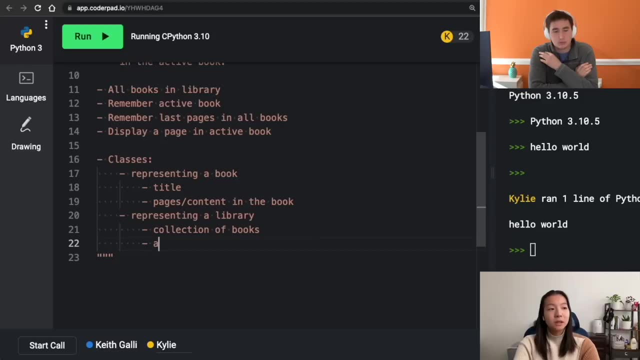 books. and then I would also argue that this page, or sorry, that whatever the active book is would would be at the library level, because, because we just want to toggle which one is active amongst this entire group, right, yep, and then actually. so this last page in the book, what I want, I think I'm gonna put. 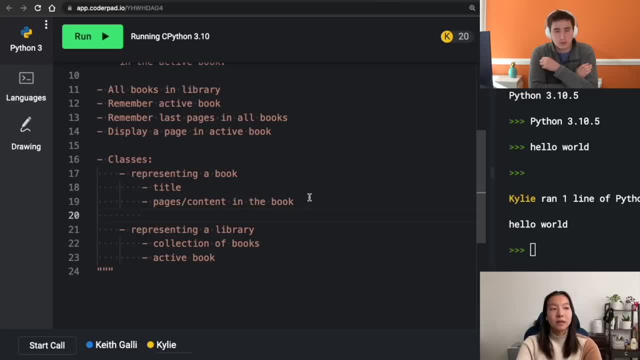 that under the book, because it's book specific. so I think it would make sense for every single book to just remember the last page, so okay. so I like how this is represented and then I think, kind of diving more so into the implementation, I think for the title, a string would make sense here. 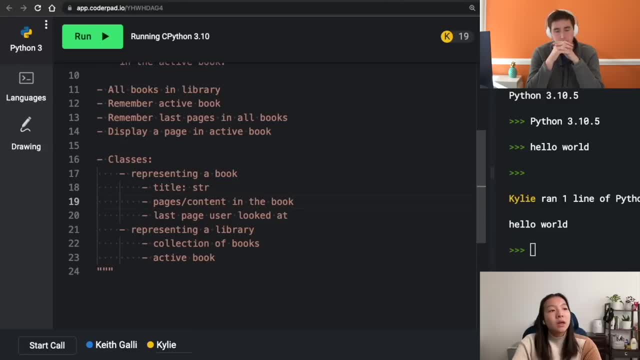 because I mean, a title is just a string, yep the pages and the content in the book. so the things here are: the pages are ordered right. when you go through a book they're ordered and there's a specific amount of content per page, and so I think something that would make sense for this is just 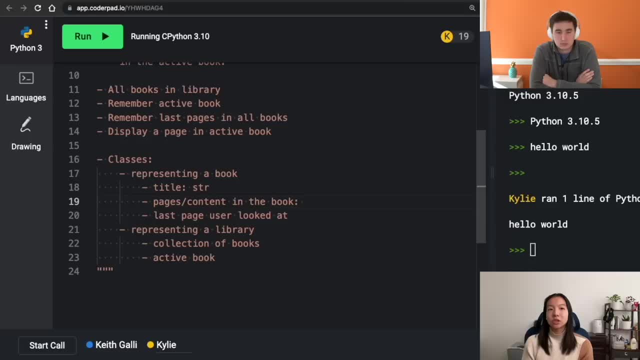 a list, because I think a list is ordered, it's a collection of items and um, and we can't, I mean I think, like a set, you would lose the ordering. a dictionary, you would lose the ordering and you would also over complicate things a little bit. you could have the page numbers as the keys, but then um, but then. 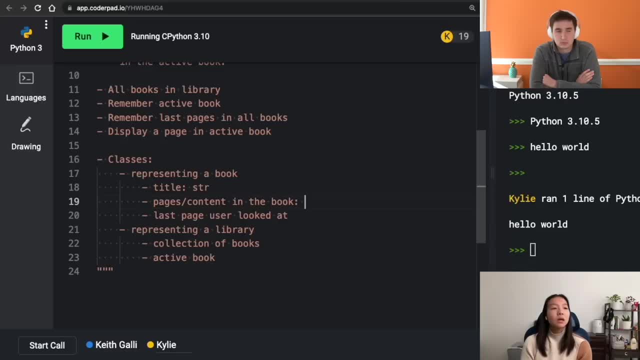 a list would also do the same thing, but kind of in a more elegant manner. and then finally, uh, a tuple. okay, you could also have a tuple, but, um, I don't think there's a reason to use like a tuple over a list in this specific example. yep, or like vice versa. 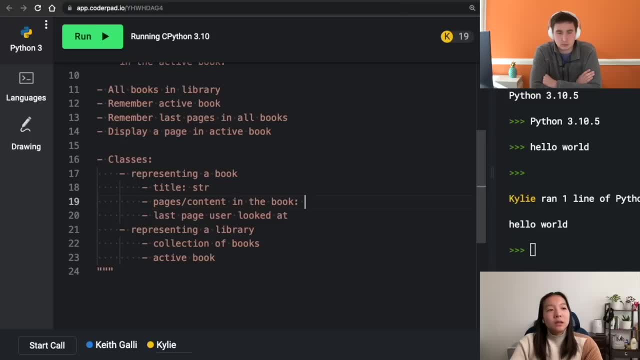 like I, I think that you could choose from either one. so I think here I'm just gonna use a list- of um, I guess, strings which represent per page. so, like each string represents whatever is on an entire page and then the last page that the user looked at, this would just be some integer and this: 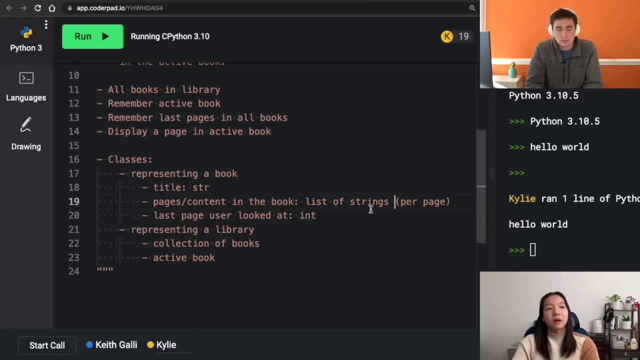 would be an index into this list of strings. so I would have to remember that this. you know there might be an off by one error here. um, because in Python we start at zero, but, like naturally when we're reading a book, we might start at one. yep. 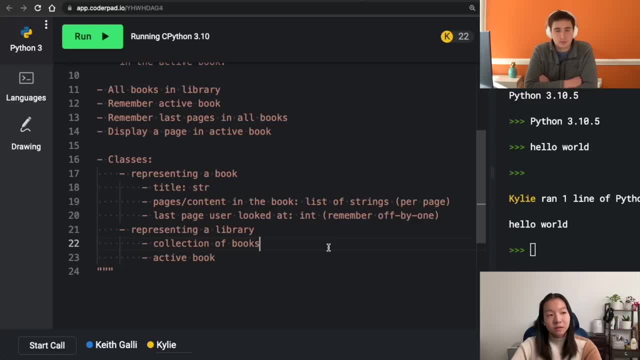 now for this library, for this collection of books, okay, well, so for this active book, um, I think you could either use a Boolean where you set one book to active and the rest to inactive, but I think that that would be kind of excessive, because every single time we toggle a book as active, we have to toggle everything else as 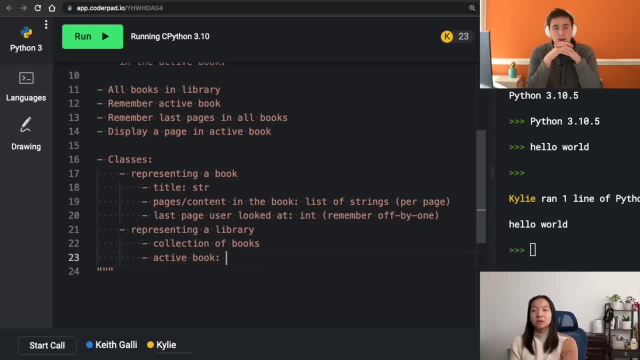 inactive. right, you can't have two active books. yeah, yeah, okay, yeah, that makes sense, okay, so then I think, in that case, instead, what I would rather do is have some sort of um, um, a string or some sort of like an ID matching system where we have like one. 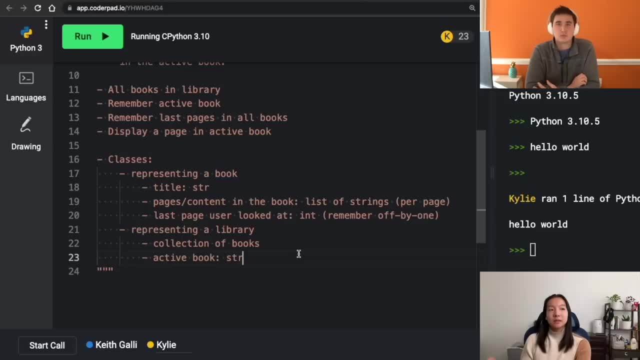 um variable that's set to the active book and that might be the title or the ID of a certain book in the library. so maybe, maybe we can just add ID here, um, and maybe I can make that also a string or an integer or something. yep, and I'm gonna add a question mark to kind of just say: 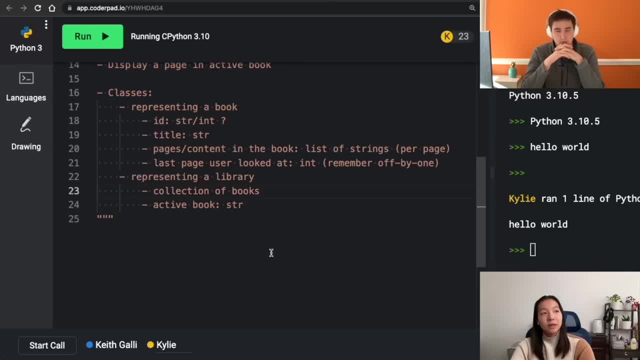 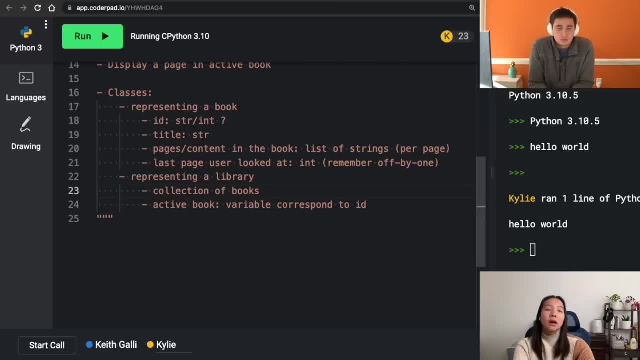 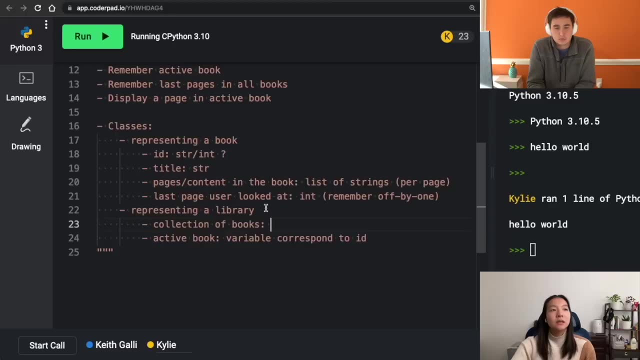 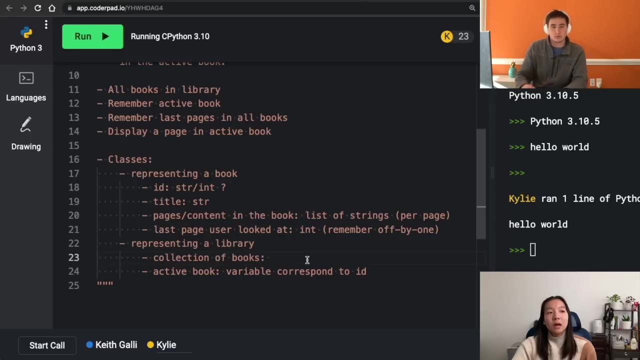 this would just be some variable. and then this collection of books. so I guess, like when we display this page in an active book, um, I actually. so I think that this, we, this might have an advantage being like some sort of a look up table, because we have a certain sense of an ID right, and I think what could make sense here. 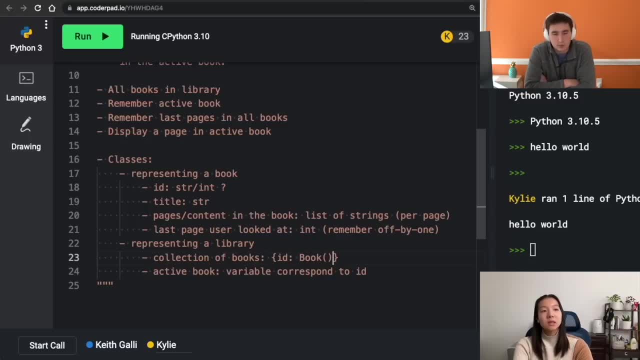 is having the ID correspond to the book object that we define up here. so, yeah, this could be a book object, right, and so, um, we don't really need this ID. I think that if all the titles are unique- mm-hmm, then- then we don't need this ID. we can just, we can just use the titles as the IDs. uh, but in some cases, in 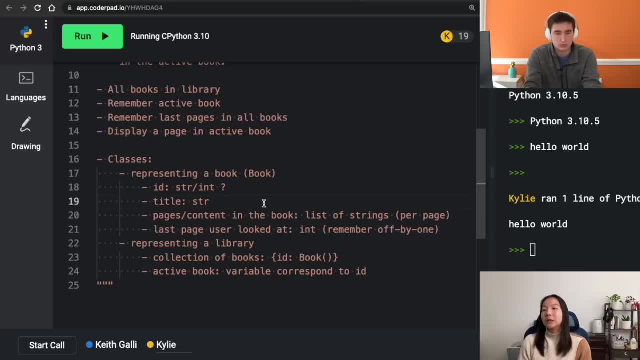 the real world, not all titles are unique, and so that's when an ID might might come in handy. um, and so I'll leave that like. what are our assumptions here? can we assume that the titles are unique, or should I be using this ID structure? I think I like the ID structure because, yeah, we're. 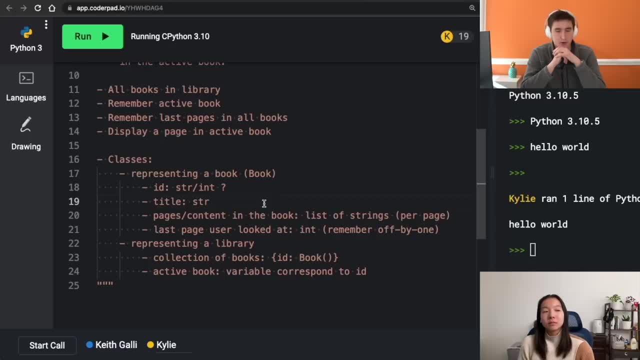 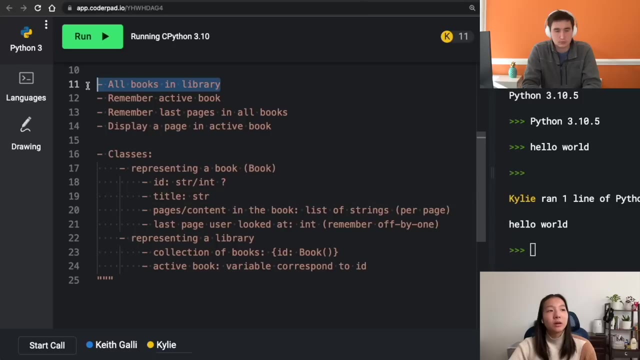 not necessarily going to know that everything's unique, so I think this is a little bit more robust. okay, okay, awesome. so I think, um, this representation looks good to me. so I'm just going to go through, uh, the requirements again, just to make sure that I've covered all my bases. so here I want all books. 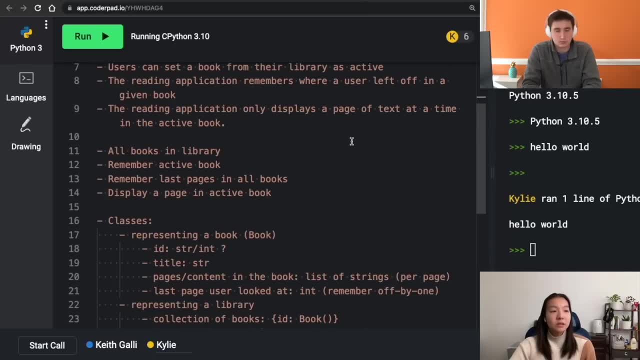 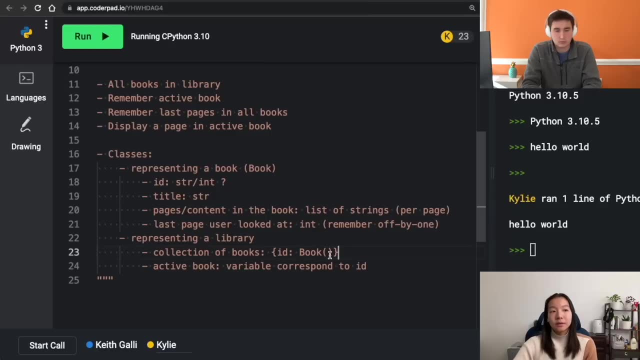 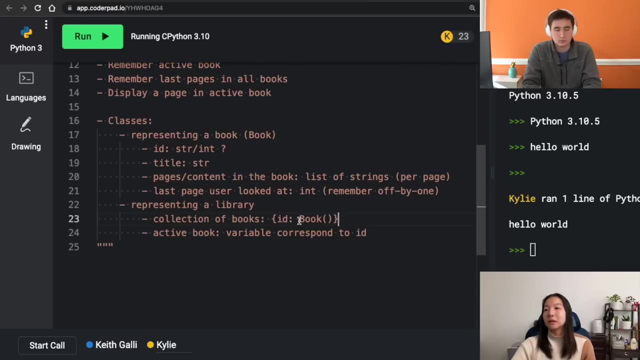 um okay. so I want a library books that I can add to or remove from, and so here I have a library and anytime I want to add to this library I can just add an ID. I can add the book. if I want to remove um from the, from the library, then I can just simply delete the key item pair. 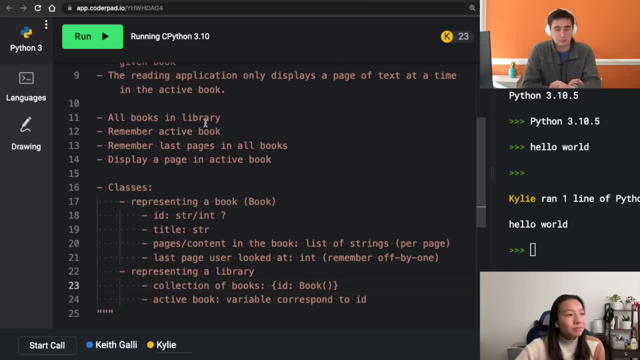 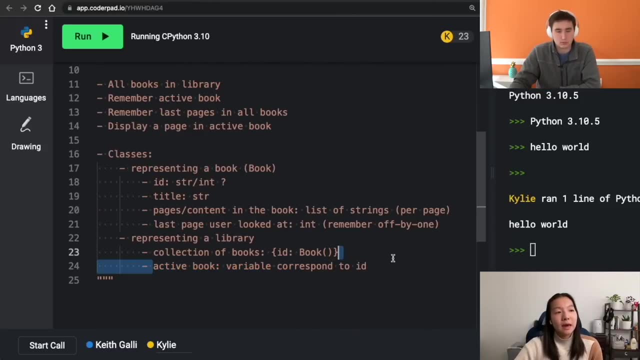 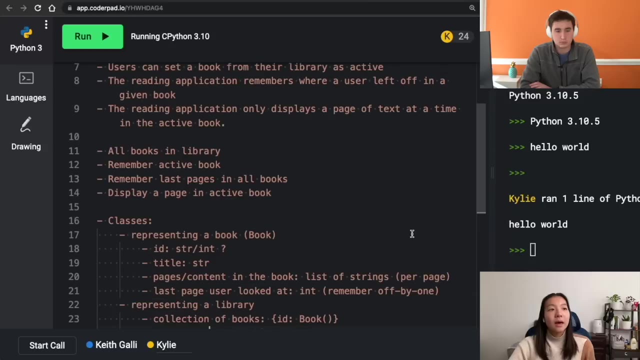 or the key, whatever pair, key value pair. Um, I can set a book from their library as active, And so here I have this active book and we could always say, like, if there is no active book, then we set this to none, or something like that. Um, the reading application remembers where a 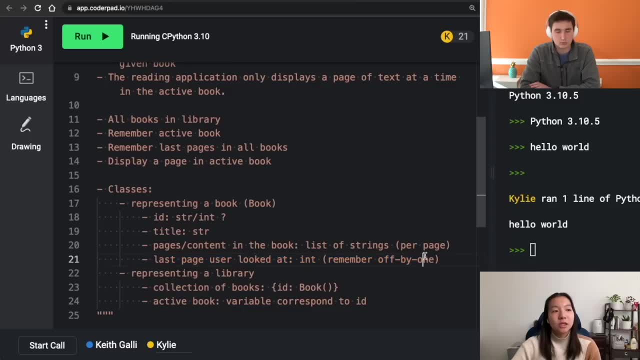 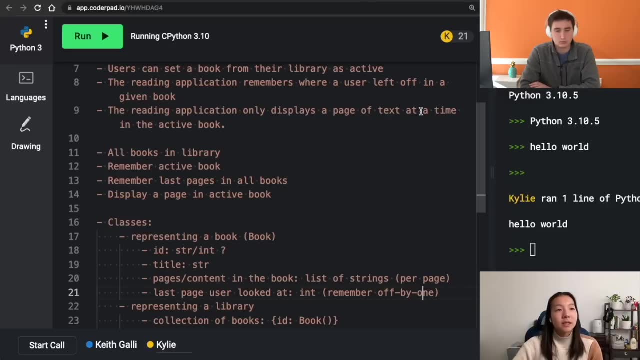 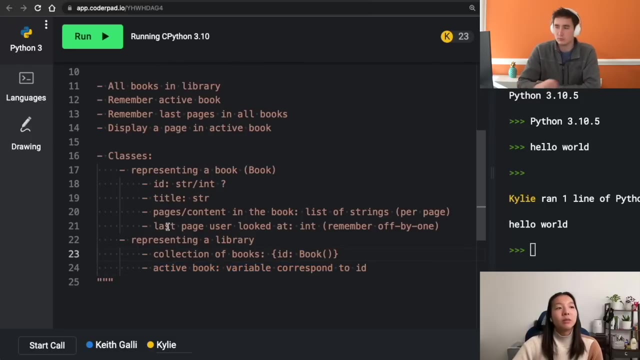 user left off. So we have that here right, The last page that the user looked at and not just in the active book, And then um displaying one page of text at a time in the active book. So we have the active book, We can get the book object from that And then we can go to the page. 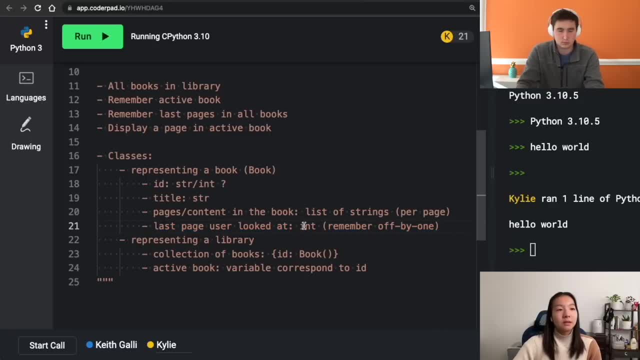 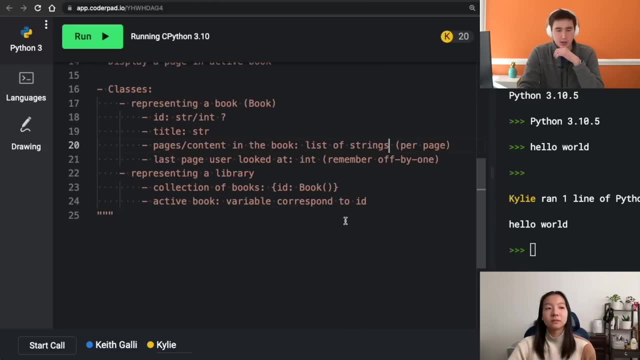 that the user last looked at by indexing this value into this list. So I think we've covered all the bases here, Cool, Um, let's do a a couple of questions here. Um, let's do a couple of questions here. Um, let's do a couple. 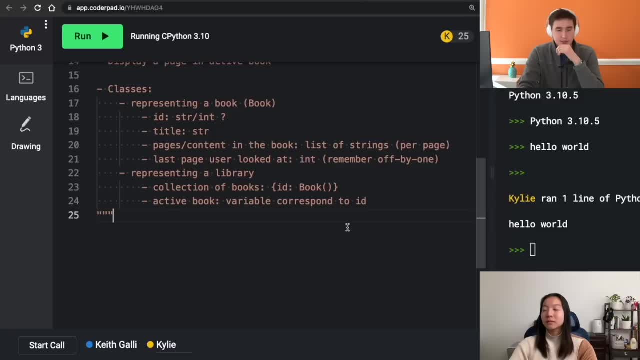 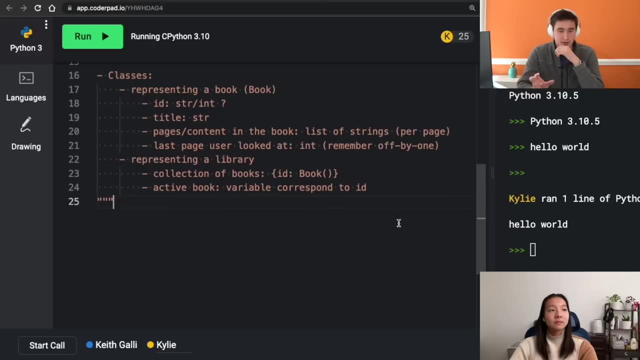 of things. I guess, I think, as a starting point, uh, and this doesn't have to get too crazy, but I would love to just see some, you know, Python pseudocode or even some Python kind of code, just to like, maybe flesh out one of these classes. I just want to, uh, you know, look at. 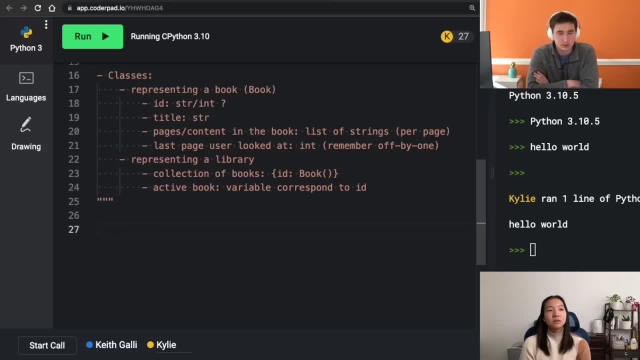 that a little bit and how you would actually start writing this code. Yeah, sure, So. so for example, here I let's start with the book Um, and when we define a class, let's initialize this. So when we initialize a book, we definitely should pass in the title and then um, the content. 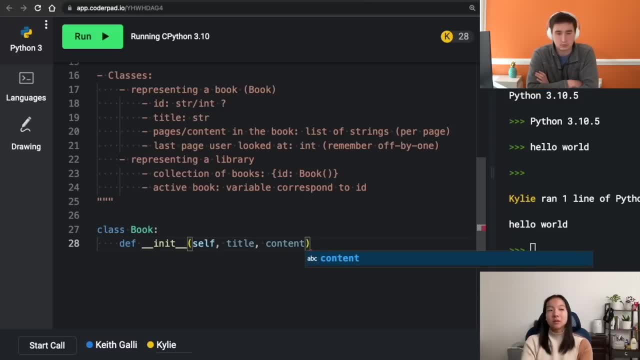 right, I'm assuming that when we add a book, these things have to be given to us, And then I'm assuming that when we add a book, we don't have a last page that the user has looked at. Is that an okay assumption? Yeah, I like that assumption. Okay, So we can set the title of. 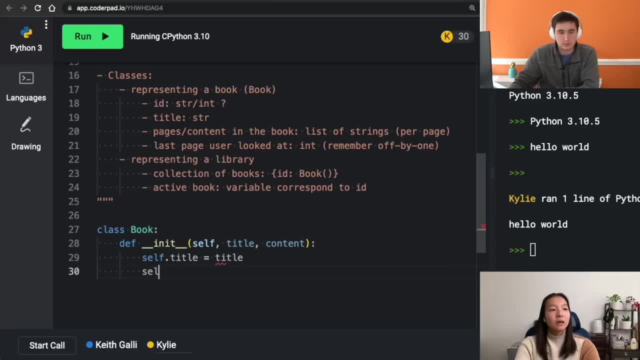 this book just equal to whatever the title is. Uh, the content of this book, and I'm going to assume that these are given to us in the formatting that we want. So the title is a string and the content is a list of strings. that 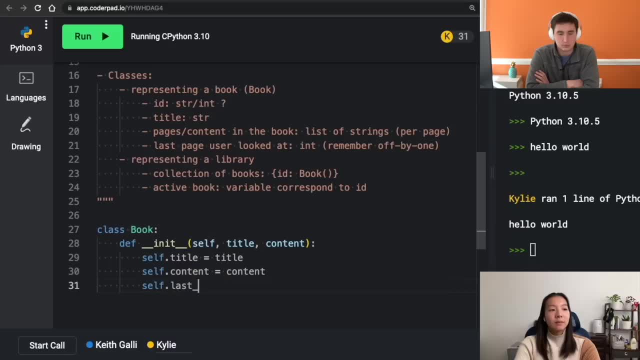 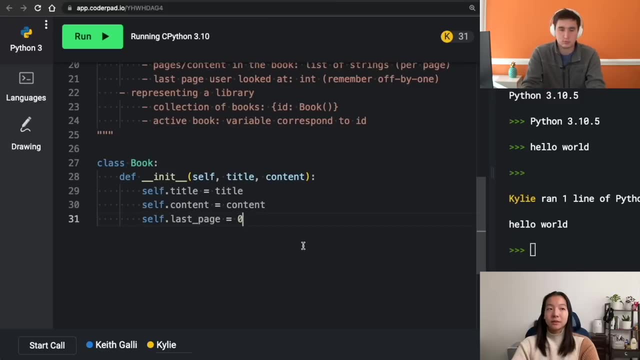 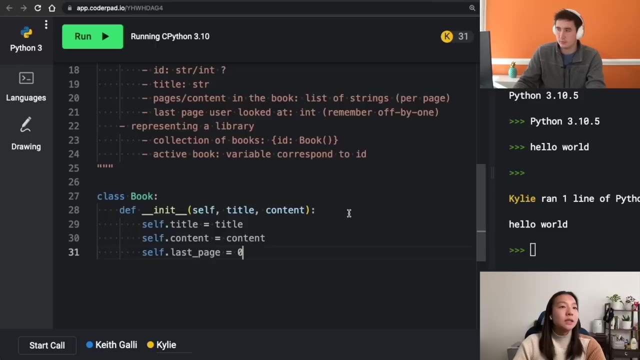 correspond to the pages Um, and I'm going to create a variable last page and I'm going to set that equal to just zero. I could also probably set it equal to negative one or something, but I think zero makes sense because that would be the beginning, right? Yep And um. 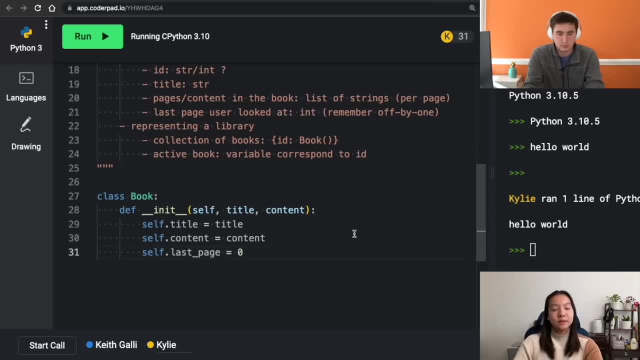 and then we need to come up with some sort of an ID. So typically, maybe we would have some sort of function that takes in the title and the content, or maybe the author or something and like returns a unique ID. Um, but I think maybe something that we can do here just very simply is, uh, have some. 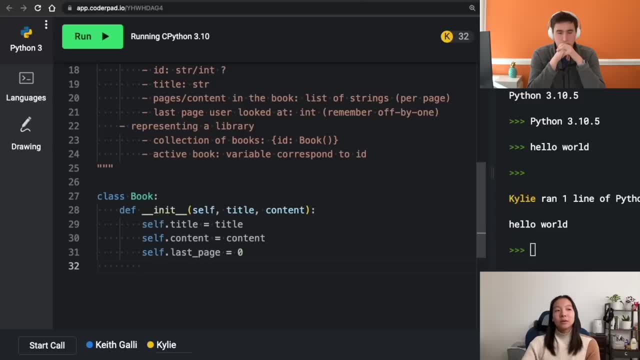 sort of counter in the library And then every single time we like add, add a new book, we can create that counter with that book, And so then we know that they're all unique and um, and they all have their own IDs. Would that make sense? Yeah, that that makes sense. Okay, So then I would. 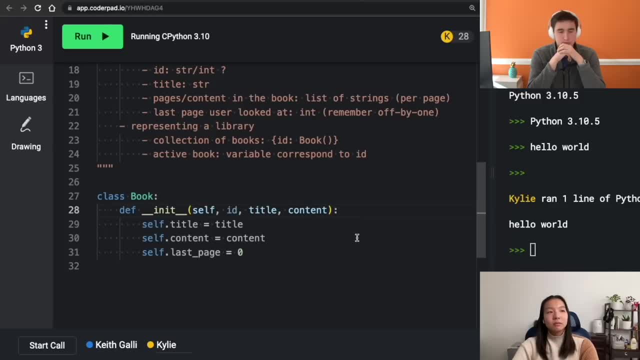 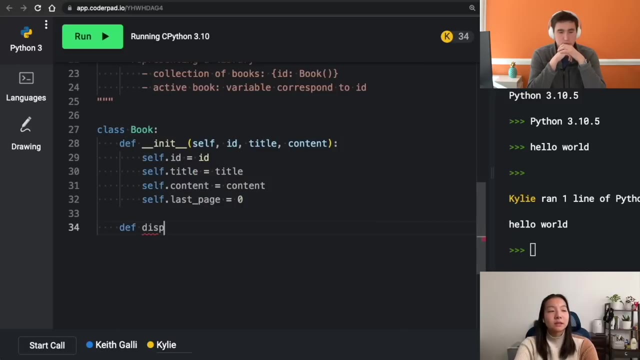 have to pass in the ID. Um, yeah, And so what I'm actually going to do is self dot ID equals ID. Uh, and then yeah, And so, then, uh, for example, we might want like a display page right In this. 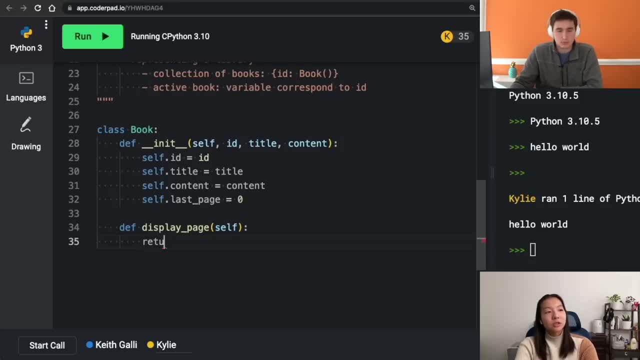 book And so for that. then we just want to return, um, whatever's at the last page of the content And I guess let's build on this a little bit. Uh, another useful function. you know, obviously you want to start at the last page, but let's say we're starting to. 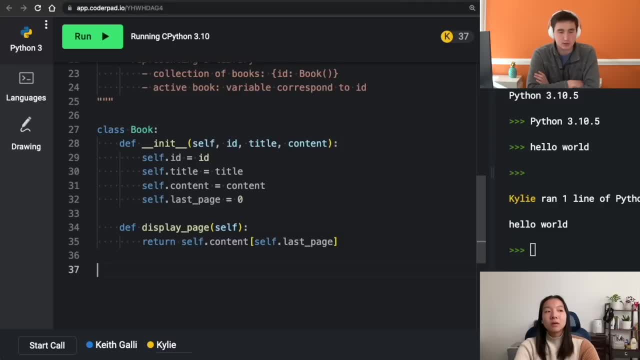 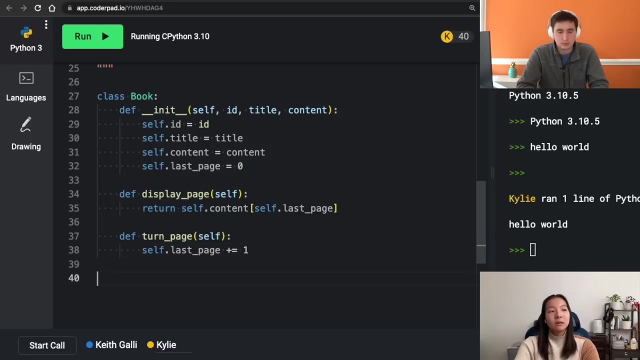 turn the page. What might that look like? Right? And so if we're turning the page, then all we want to do is increment the last page, Right, And so we might do self dot last page and we just increment that by one Um, and then we could call display page after that. Uh, if we 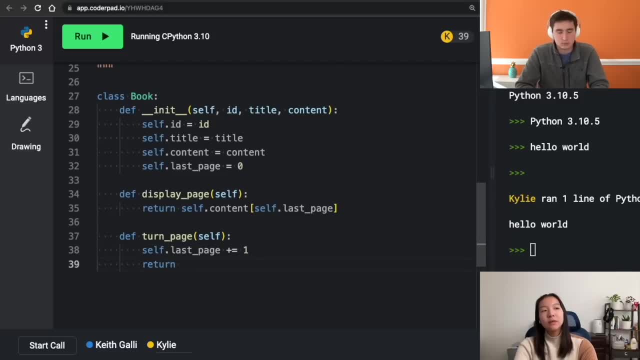 assume that, like we could, Yeah, Yeah, If we, if we assume that these two go together, So if we assume that when we turn the page we want to display that page, then I would just return display page. Yep, Like that, Um. 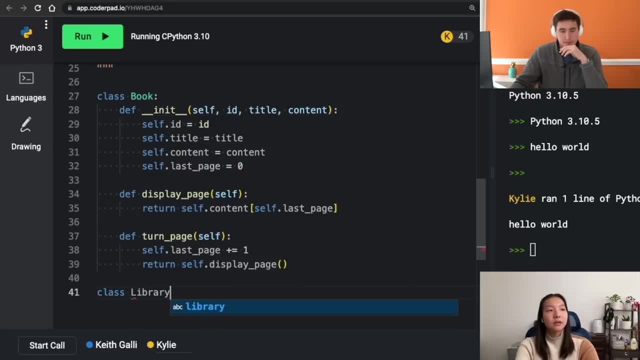 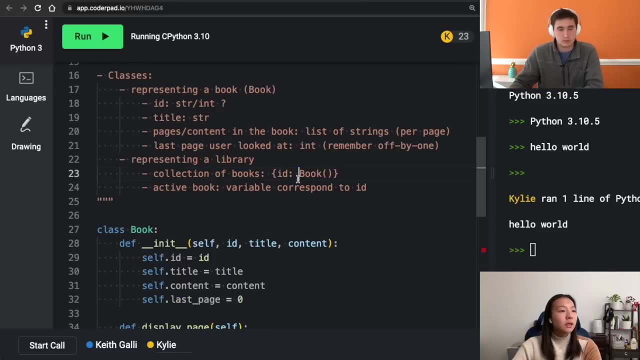 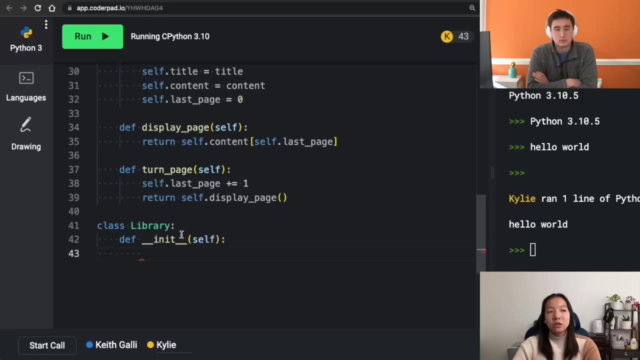 and then actually, I'm just going to go ahead and code up this library as well. So, this library, we have this collection of books and then also the active book. So it's literally just going S and F, um rather than uh, initializing the library. 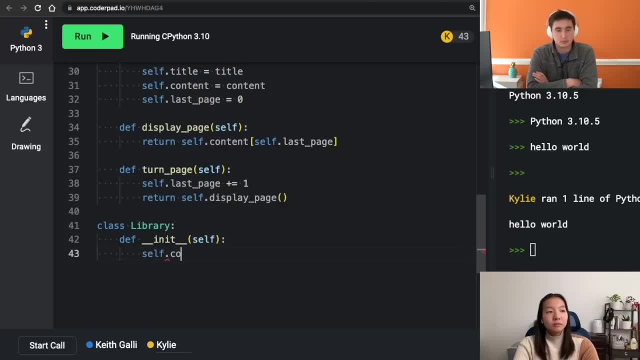 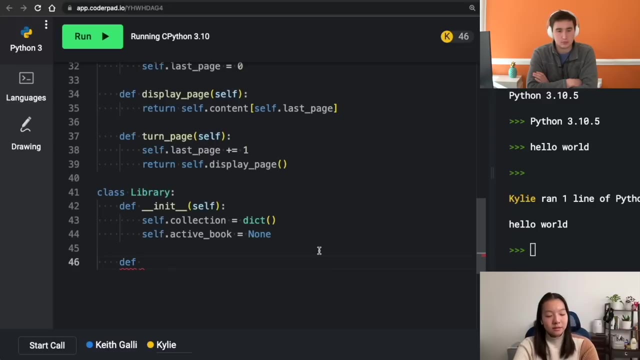 with books, I think let's just add them, um, to this. So initially this collection might just be an empty dictionary and then the active book might be done, Right? So then, um, when we want to add stuff, Yeah, 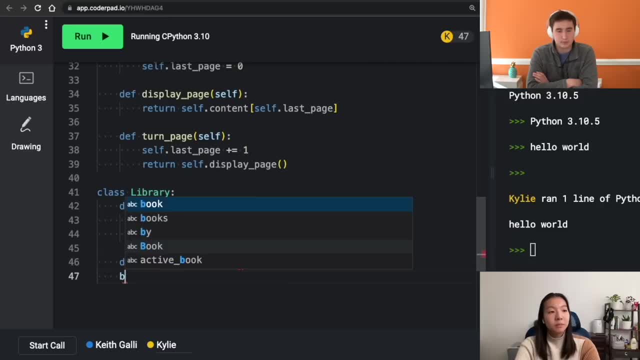 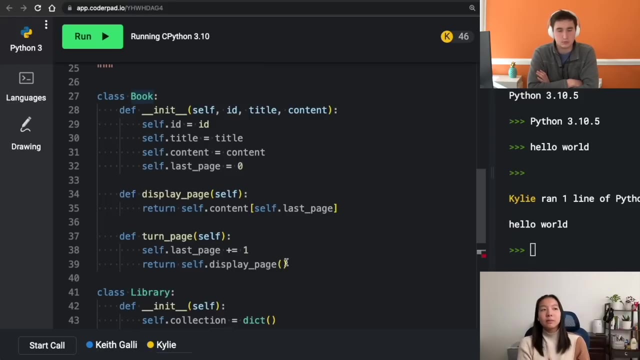 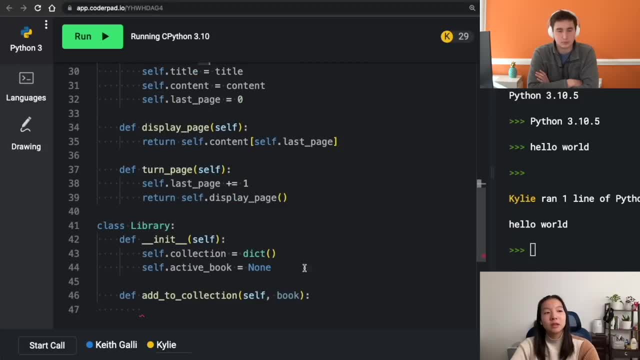 we're. we said that we would pass the ID through like the library, because we might have like a counter, like some sort of ID counter. I mean, this is not the best way to do it, but I think this is like a fine hack for right now, just to. 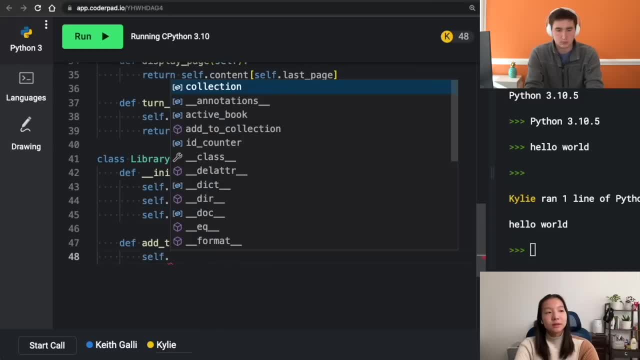 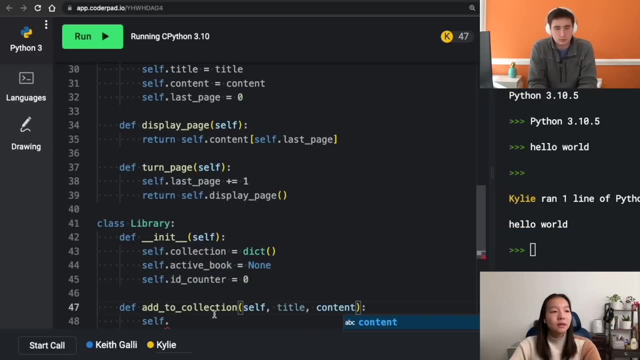 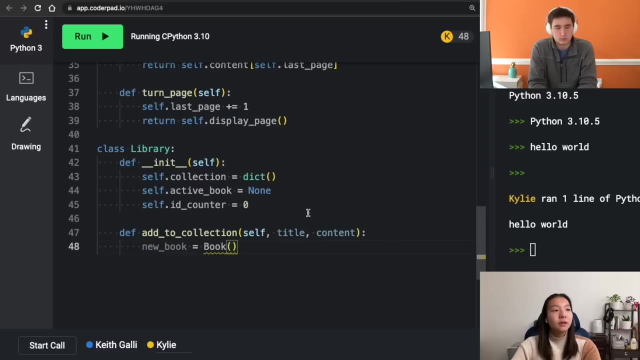 make all the IDs unique. what we can do here is we can also, when we want to add a book, just pass in the title and the content, and so then our new book is going to be a book as we've defined above, with the ID and the title and the content, and then we can add the book and then we can add the. 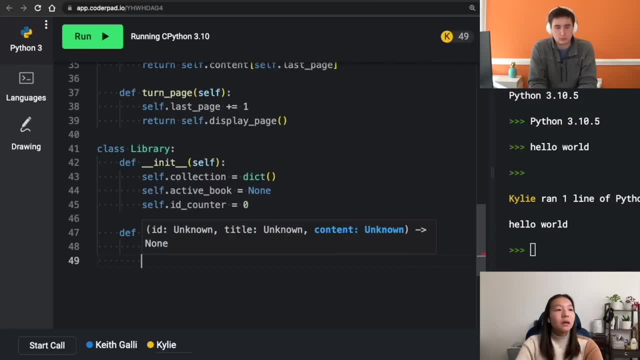 title and the count or the content, and then, after we create this new book, we want to increment the ID counter, uh, and then we also want to add this new book into the collection, right, so I'm going to add selfcollection, um, and I'm going to make the ID whatever the ID of the book is. so actually, I'm just going to. 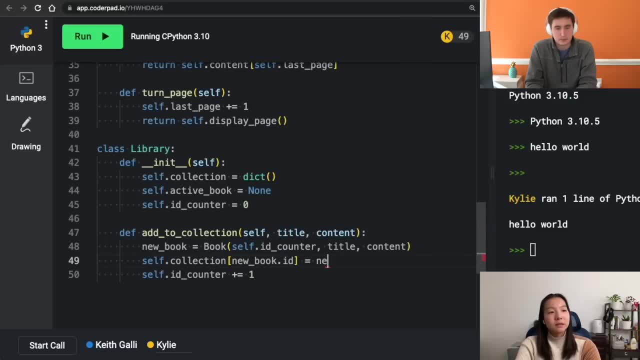 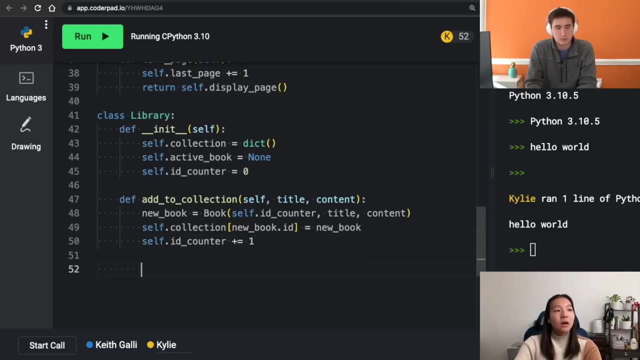 call newbookid, because I think that's a big one to get cleaner and this is going to be the new book. and then we increment the counter by one. so this is us adding to the collection. um, so of course we want to remove from the collection and so we want. we said that we wanted to remove. 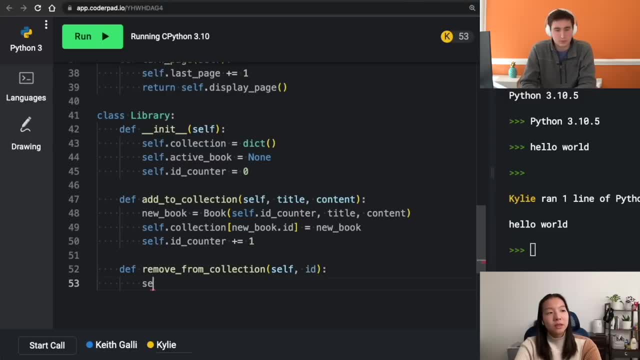 based on the ID. so all we have to do is: I think there's this delete in python. I'm not sure if there is. do you know, Keith? okay, is there a remove? let's, I think that there's. I mean it should autocomplete here in the coder pad. oh, isn't it Dell? isn't there a Dell? um, I mean, I think. 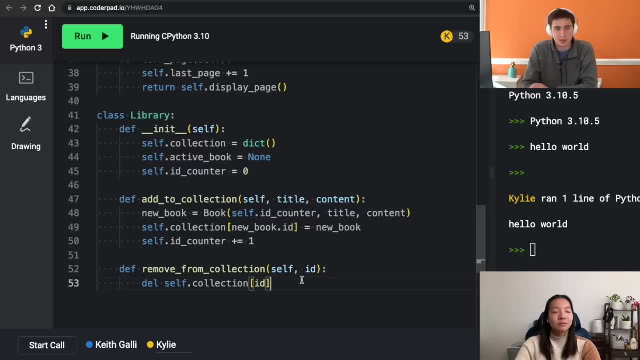 the biggest thing is: is it going to be happening in place or is it going to be happening in creating a copy? um, I, I understand, yeah, so we want it in place from the collection. I understand what you're trying to do, so the exact details is: yeah, is not super, super important to me, okay, yeah, so, anyways, this is removing from the collection. 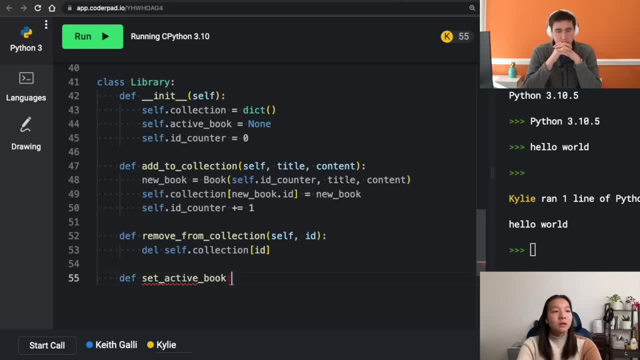 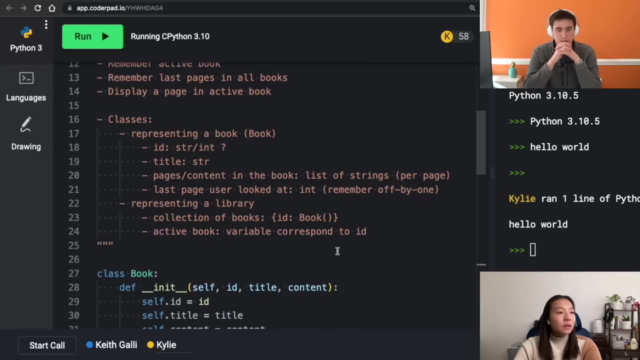 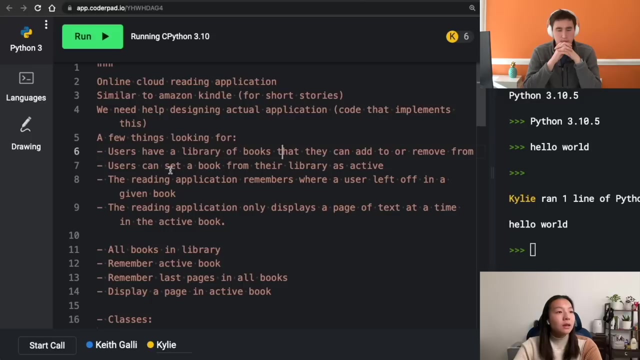 um, and when we set active book, again, we want to do this based on the ID. so I'm going to make self dot active book equal to whatever that ID is. uh, and let's see, so the user has a library books they can add or remove from. we did that, setting a book as active. okay, and then remembering 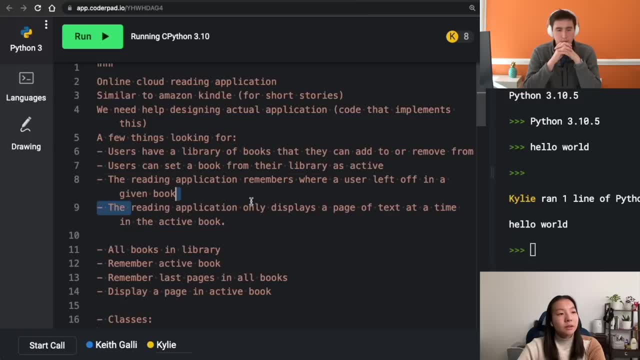 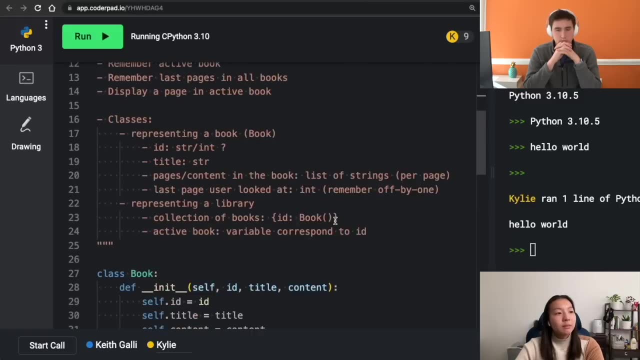 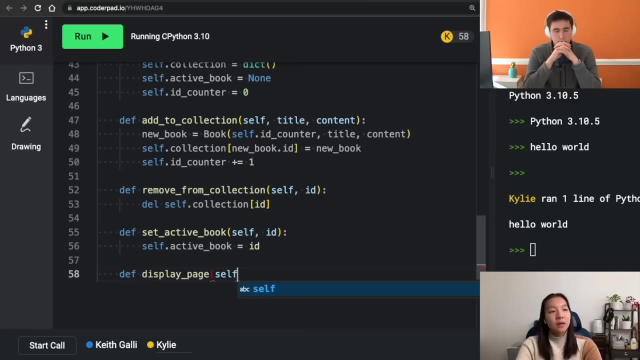 where a user left off. so we've actually taken care of that already implicitly in our um book, uh class. and then the reading application only displays a page of text at a time. all right, so then here we can say: define display page, and actually we don't even need the. the ID of the 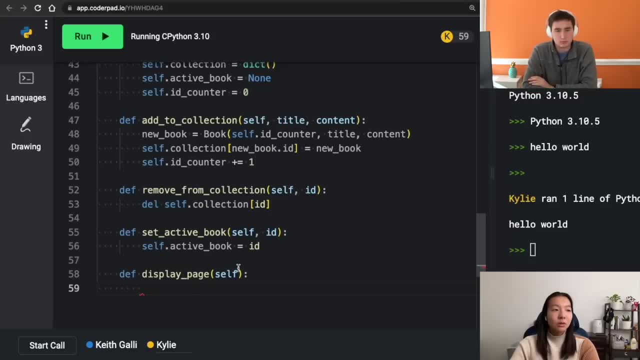 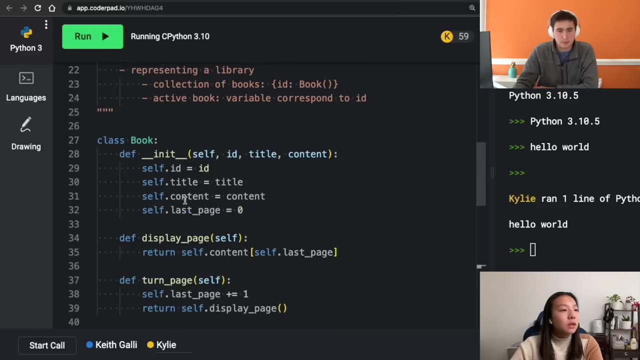 book, because we already have the active book ID, all right, and so what I'm going to do is I'm going to go into my collection, um, and I'm going to get the active book like this: so, yep, blah, blah, and I'm going to click or I'm going to do dot display page. 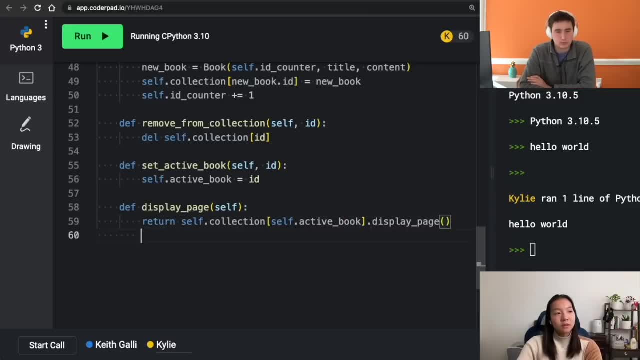 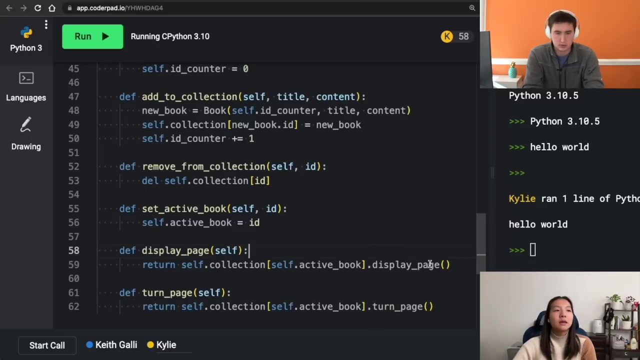 and then, of course, we also have this turn page that I could, um, just put up as well. so you get the idea, but so we want to, oops, turn that page. um, I do think that some like drawbacks here or that, uh, okay, so one thing that we could have done: 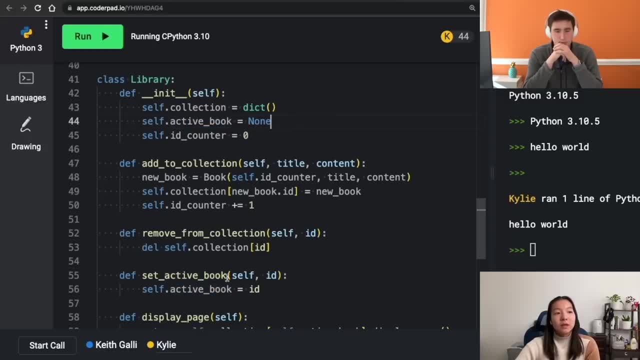 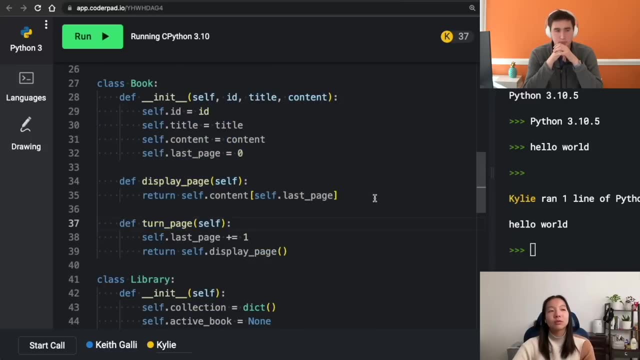 is instead of this active book. instead of saving the ID, we could have saved the book itself, and i think from a pythonic standpoint that might make sense. but then in the future, if we're using some sort of database or something, an id would make more sense because that's easier. 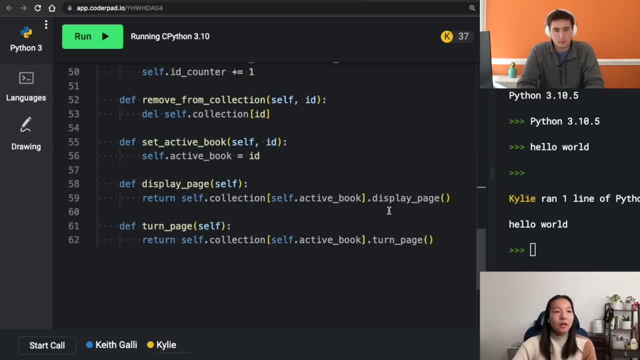 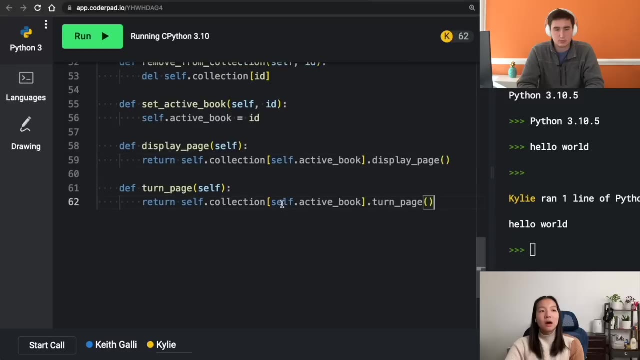 to store in like a table, um and if, uh, and okay, also for this display page. you might see that we've called this display page and turn page up here in the book and the reason why i did that, rather than um, rather than just call like selfbookcontent, last page, like booklastpage. 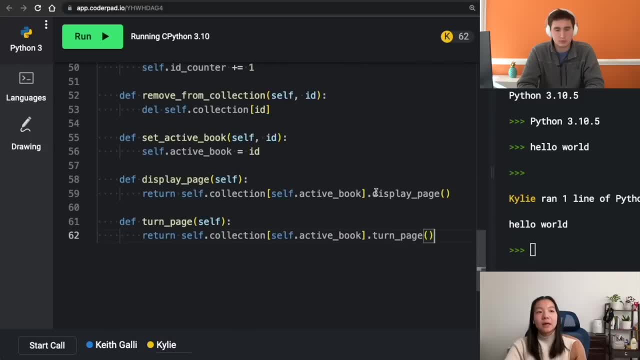 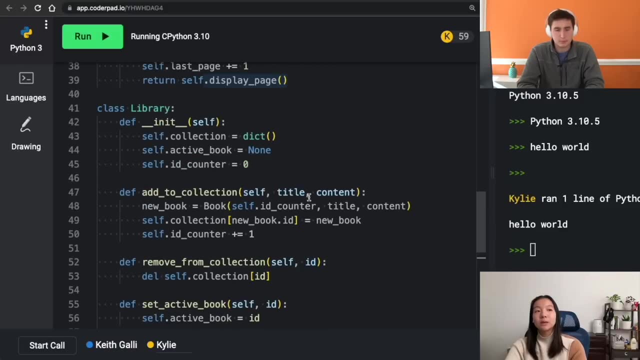 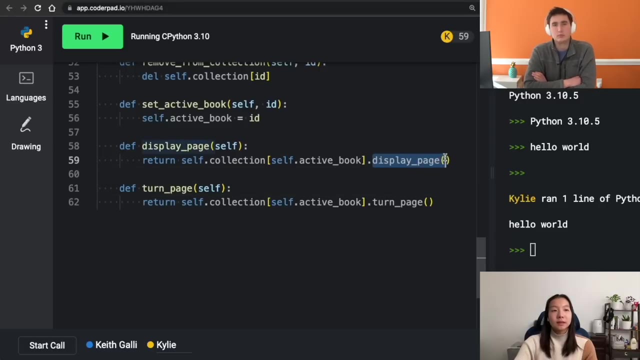 or something, was because i think that, like, for example, this should be independent of how we implement the book right, so we want to keep those as kind of block, like separate blocks as possible. and so here, what this allows me to do is when i go back to my book, like, if i decide to, 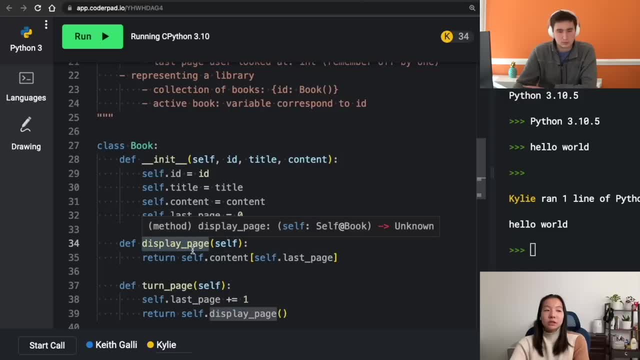 scrap it. i'm just going to keep it as a separate block and then i'm going to keep it as a separate book. i'm just going to keep it as a separate block and then i'm going to keep it as a separate book. this implementation: implement something else. i know that i would just have to implement the 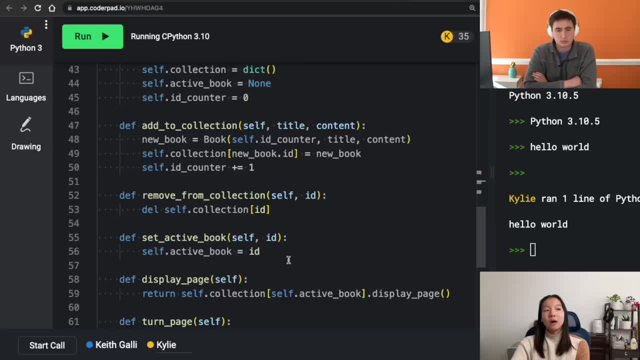 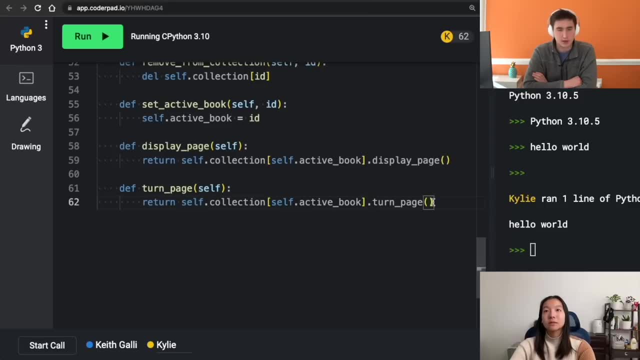 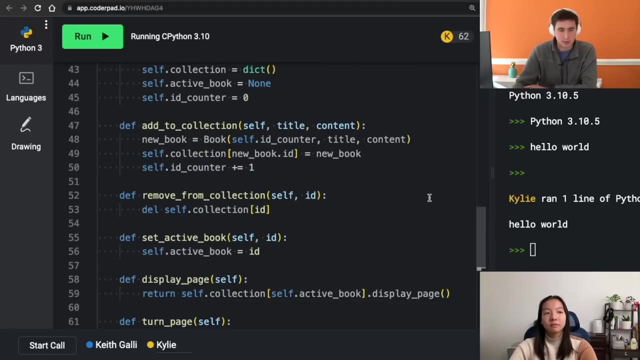 methods: display page and turn page for that to work. um, and like these functions, cool this. this looks good to me. i like the start. i think that this uh definitely lays out the foundation of what i was uh looking for with the requirements of this application. so nice work with this. a couple. 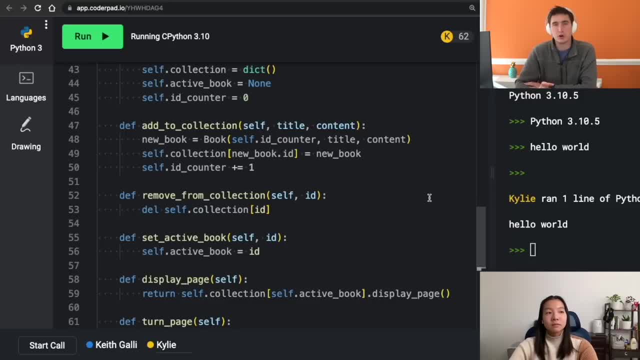 quick follow-up questions before we kind of branch into more of an algorithms, uh type question as the follow-up here. um, one question is: you know, let's say you have an older reader and their vision isn't as great, so they need to make this the size of the font bigger. so kind of keeping 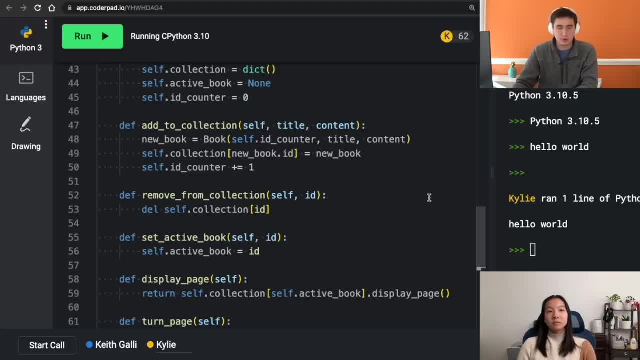 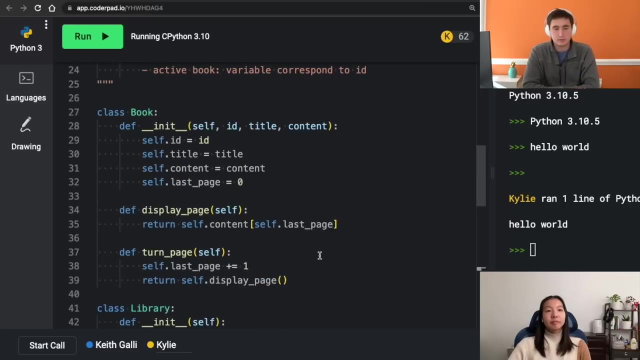 that in mind, that you might have this variable font size, how might you, i guess, refactor or change or modify your current structure- and you don't have to actually write code here, let's just discuss this- to account for, um, that increase in size? yeah, yeah, so i. so when we increase something in size, like i'm just thinking about, intuitively on our 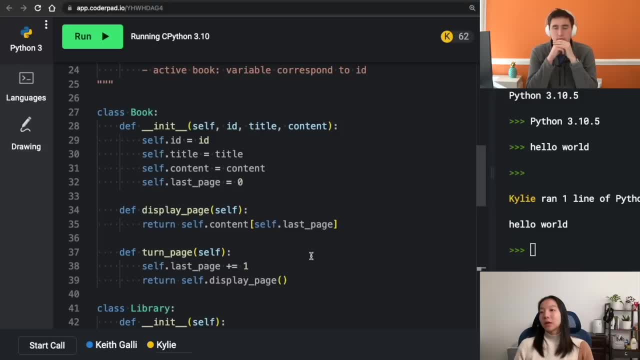 like phone screens or something um that that tends to shift the content right. so, like some page that might hold a hundred words or a hundred characters at you know, um, a small font size might only hold 50 if when we double that font size. so, uh, for the book, instead of having this list. 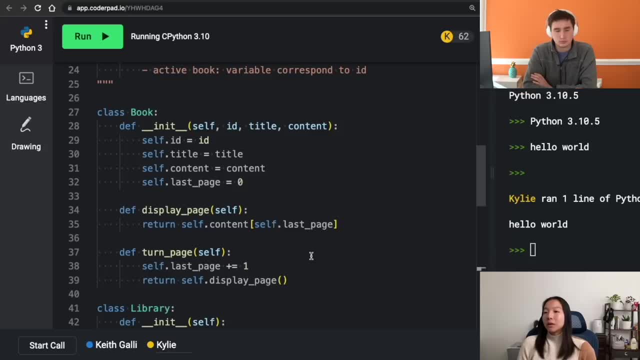 what i might do is i might just save the entire book as a string and um and based. so i would. let me just edit this in here because i think it's easier to visualize what i'm saying. but so i would, might, i might have like a font size equal to um. i guess we could just use like the traditional, like 12. 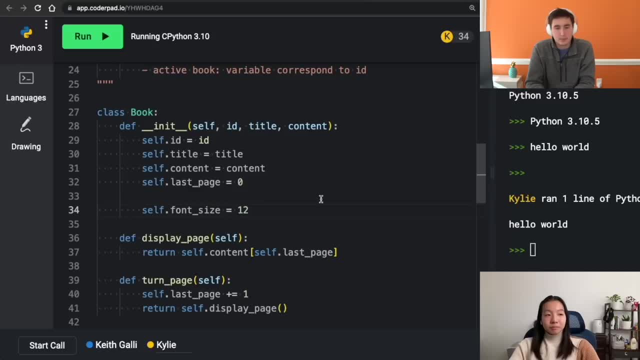 point font or like: yeah, whatever, uh, but when we have this font size, we might have to like we could come up with some sort of um characters per page calculation, right, and so that would be based off the font size, so calculate. so this is going to be pseudocode now, this calculate doesn't. 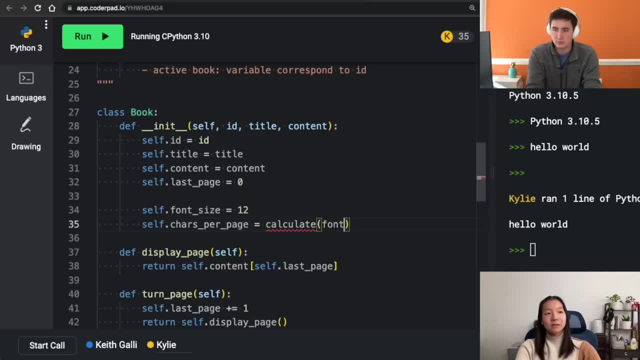 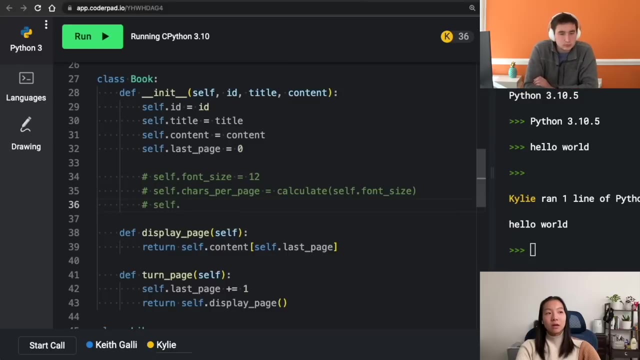 actually exist, but calculate uh based on that font size, um, and i'm commenting it out so it doesn't have any errors. but then, uh, when we do calculate that, then what we can do in order to get our um, in order to get this display page thing, would be, instead of indexing into this content, 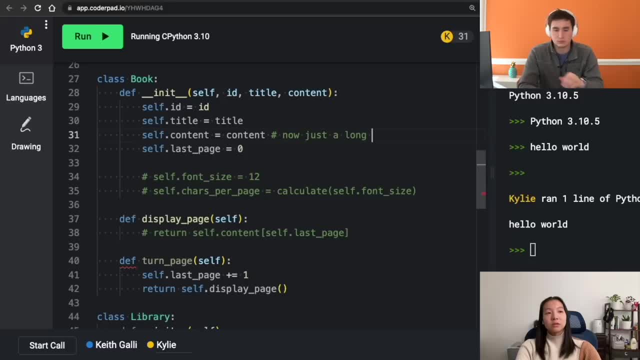 which is now just a long string of characters. what we can do here is we can return: um, we would have to do some sort of calculation, right, so we would need to. we have this characters per page, and we can multiply that by whatever the last page is and um, so this would give us like kind of the starting index of this long string of characters. 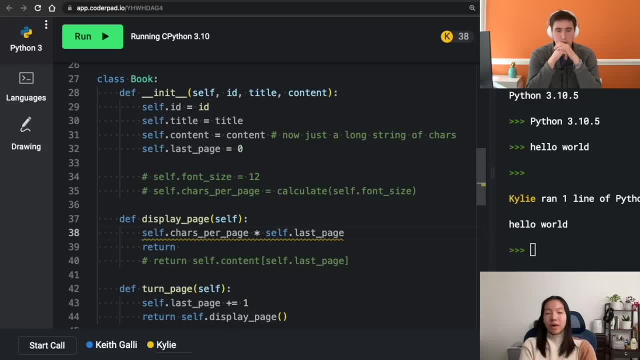 to start. uh, the content of that page start index would be this, and then what we would want to do is: um, what we want to do is then return the selfcontent from that start index until the start index plus the number of characters on that page. so that would be our end index. so actually, let me just write that out. 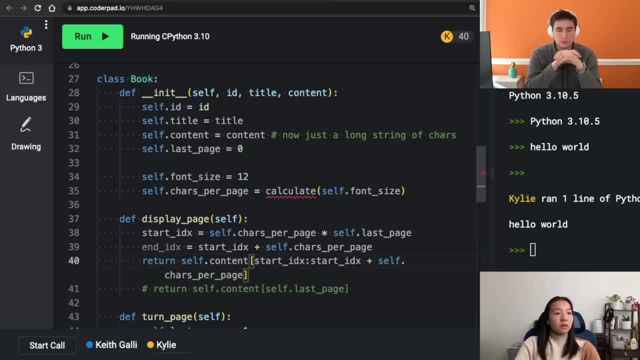 to make things a little bit more clear. so now, essentially what i've done is we have this variable font size which we can calculate characters per page depending on that font size, so that might be more characters or less characters, depending on how big the font size is. and then our content, instead of a list of strings, is now. 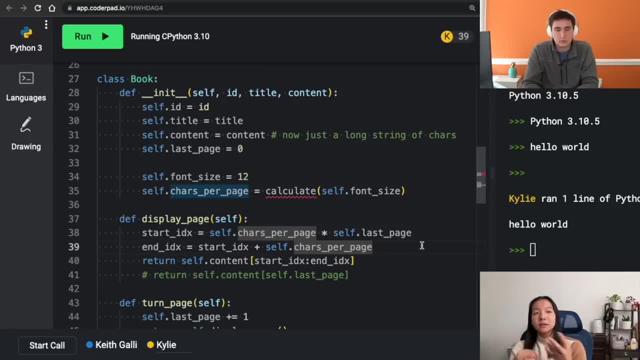 just a really long string of characters, and i guess some assumptions that i'm making here are that, uh, this would just be approximate, um. so, for example, if we had a backslash n which is like a line break, right, um, that might just end up counting as a character or two characters. but 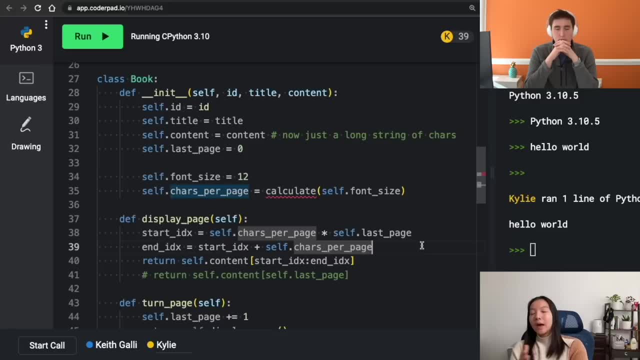 the assumption is that, um, that would be approximate per page, or maybe that we're using some sort of like monospaced font or something like that. um, but essentially, now that we have the characters per page and then just a long string of characters that represents the content we can index into. 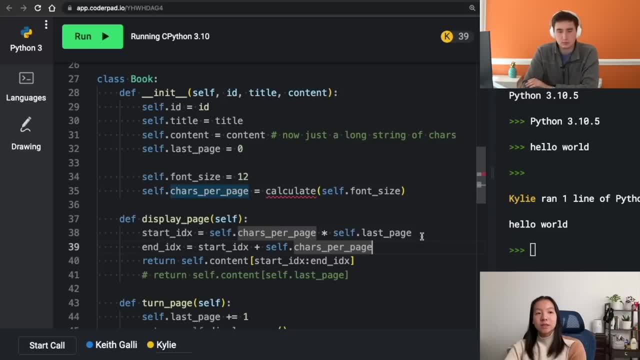 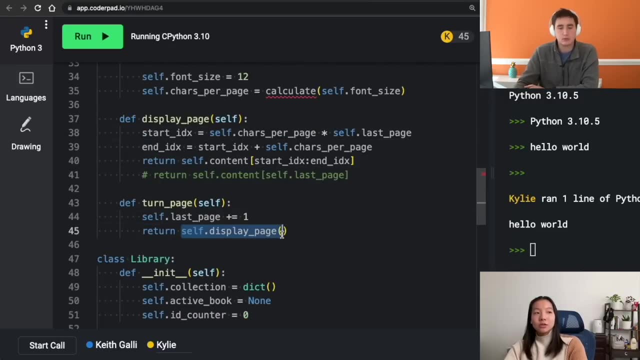 that content, depending on, like, based on the last page that we know, and so what's really cool here is that when we do turn the page, uh, we can just end up calling it. so this is kind of that granularity that i was talking about. yeah, that that makes a lot of sense to me and definitely, you see, the advantage of having, um, that inexplicable monospaced font. 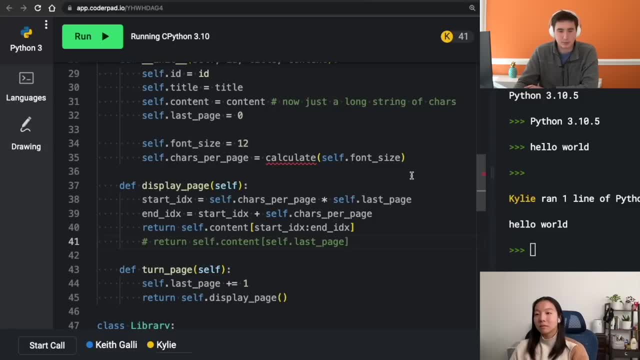 that function that you can change by having to implement something different. One last quick, I guess, follow up and then we'll move on to the algorithms portion of this interview. I'm just trying to think. you know, at a high level, let's say that we wanted, we had. 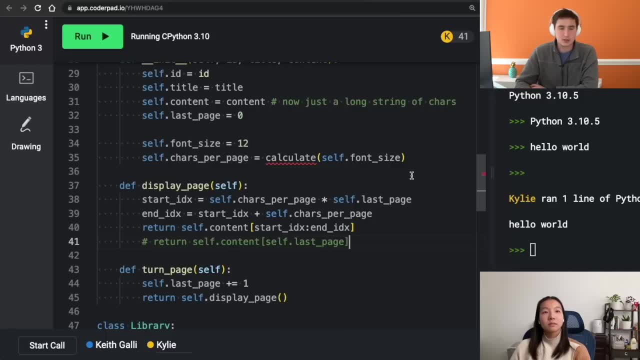 multiple users in this system and they all shared books. So, like you know, they might all share the Harry Potter books or something like that. Like books are common among all of them, How might you modify this, given that you know some of these qualities of a book might be shared between users? 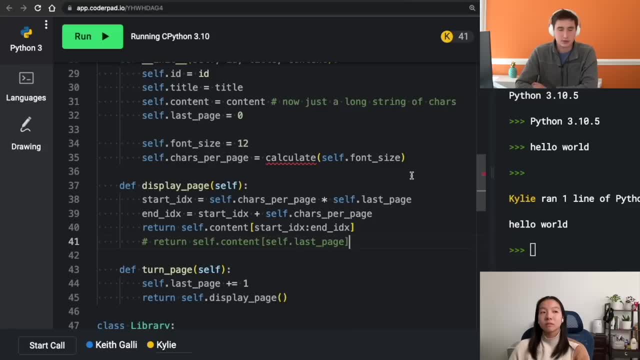 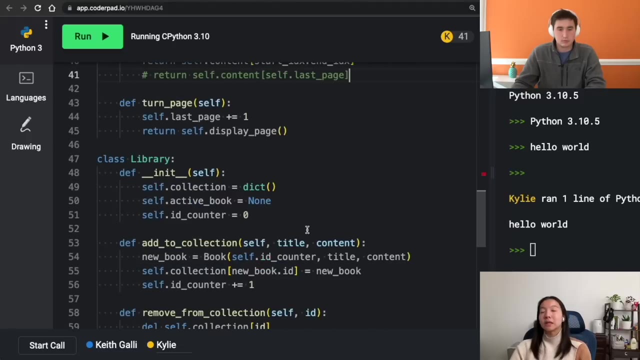 because they're all trying to access that same book. Does that make sense? Yeah, So, yeah, yeah, for sure. So I think that when we start to, you know, have like multiple people involved, like these books might get stored somewhere, for example in like a SQL table, right, And so then 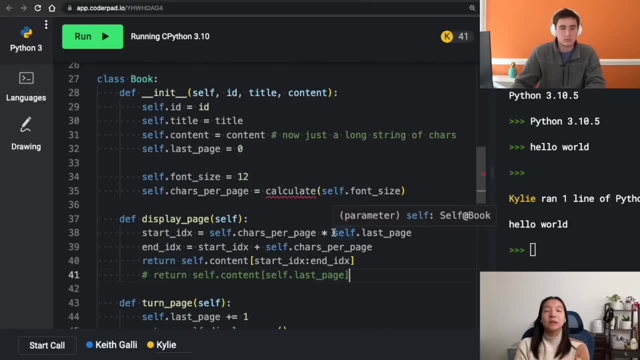 when that happens, we would still want to maybe store, like the ID, the title, the content in that table. Now, the only changes would be that the these sort of customizations are are per user, but the book and the content, those are for this entire group of people, And what we can do, I think is is: 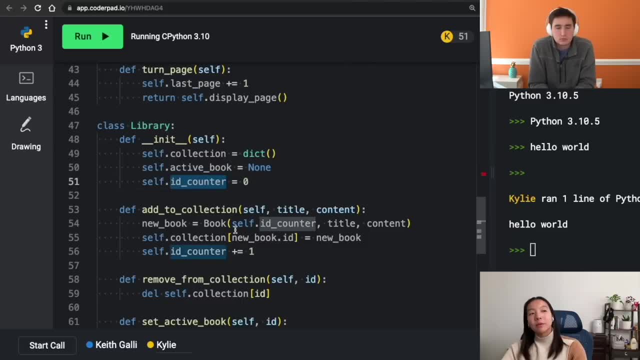 instead of this ID counter being like library specific, we can start identifying books by their ID Right. And so you know, this was kind of just a hack to make this ID thing work and be independent and be like unique. But, for example, when you put something into a SQL table, you can also have an. 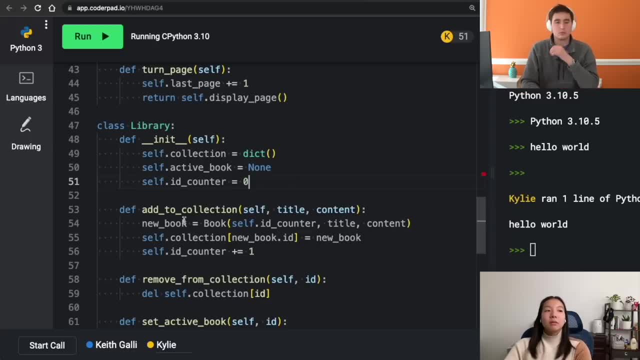 ID associated with those entries. And so maybe when we add to the collection, if we see that the title and the content is already in the table, then we instead just return the book that's already in that table, or something like that. Yeah, Okay, I think that, I think that's. I think that's, I think. 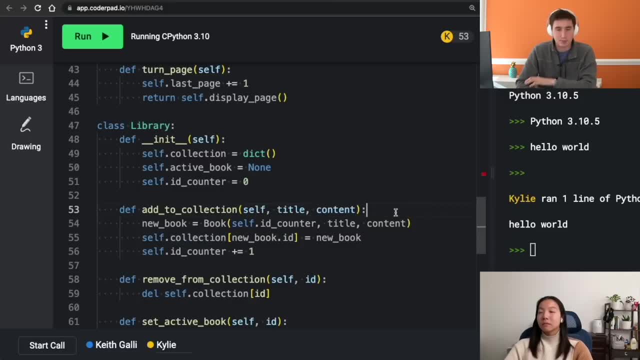 that makes sense to me. Cool, I I'm, yeah, Happy with this discussion. I think that we can move on to the second portion, I guess. do you have any, I guess, last questions on this before I move on, or last things? you want to say: Yeah, So no last questions. I think that the last thing I want to 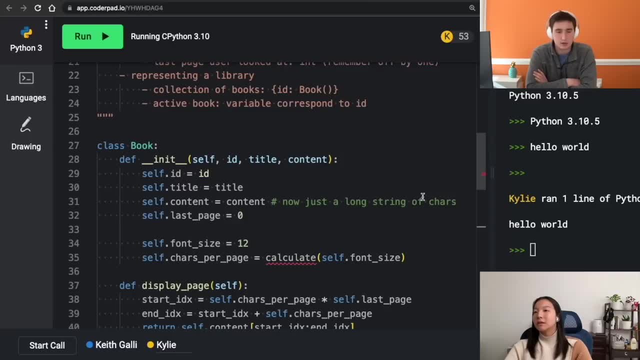 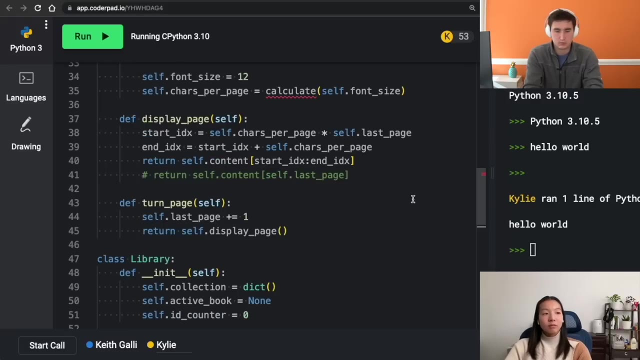 say, is also like it would really depend on, like, how you implement this like group of people, right, Like so my immediate thought was like a SQL table, but that doesn't have to be that's the only way. Um, so, yeah, I think okay, cool, I think it would depend on that. 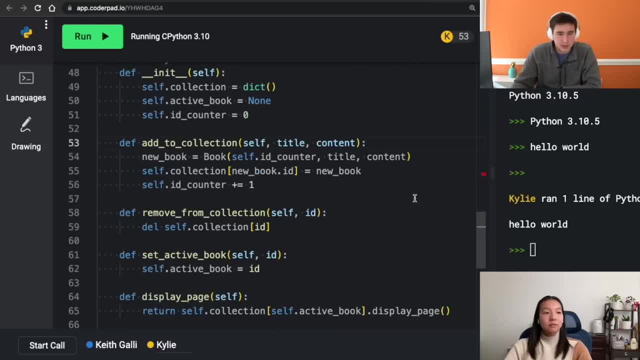 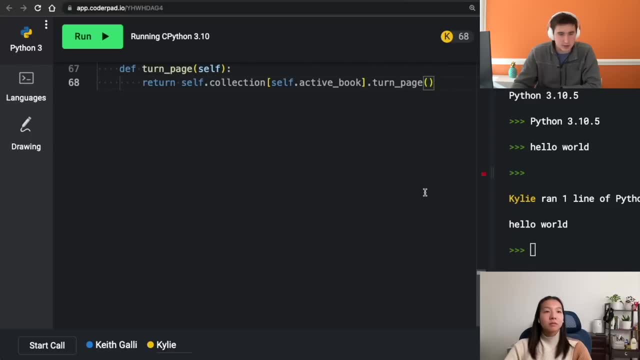 Um, all right, Awesome. Uh, let's, yeah, Switch gears, and I'm probably going to just comment this out: um, in case you do want to run some code and there's any errors or issues in this, So I'm just. 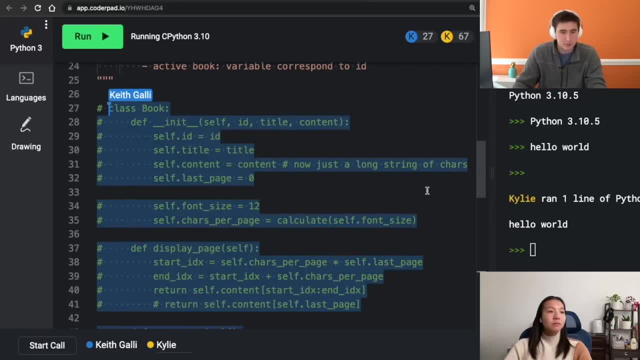 going to comment this out, but I'm going to leave it here just so we have it, um to look back at, and I'm going to just indent this a bunch and we're going to just start at the top of the screen. 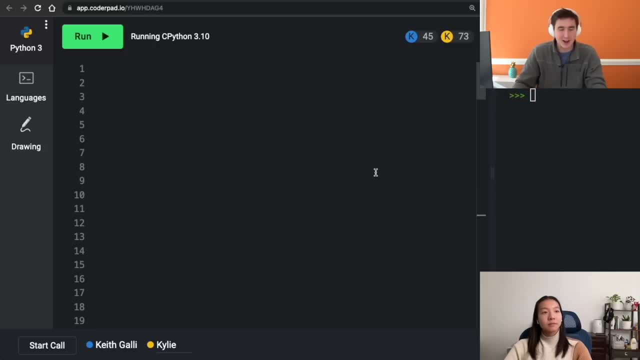 So don't mind all the stuff at the bottom, All right. So another important component of our book reading system- and this is completely independent, You don't have to reference any of your past um code is I mentioned. this is for short stories and you could have independent indie. 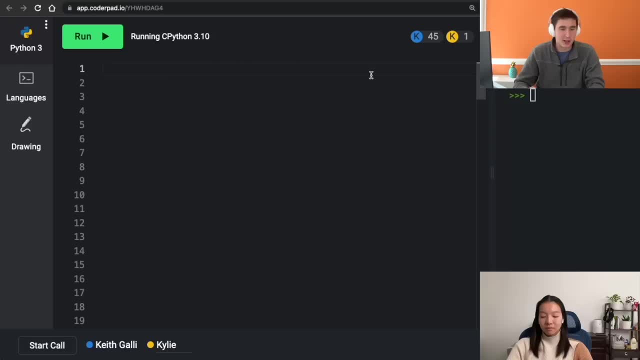 authors, you know, adding these short stories, So they're not going to be, you know, the classics, not going to be those types of titles. They're probably gonna be smaller authors. So one thing that we want to avoid in this system is: 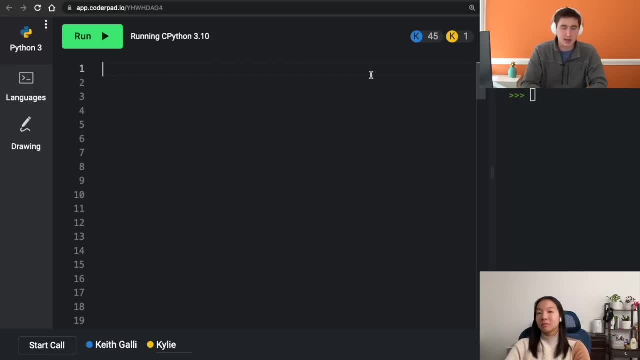 Okay, Plagiarism. So my task for you is to design an algorithm that would be able to detect the two most likely books that would have plagiarism in them. It's like the, the, the two most likely books that pop up as a match for potential plagiarism. uh, in this, in a library, And 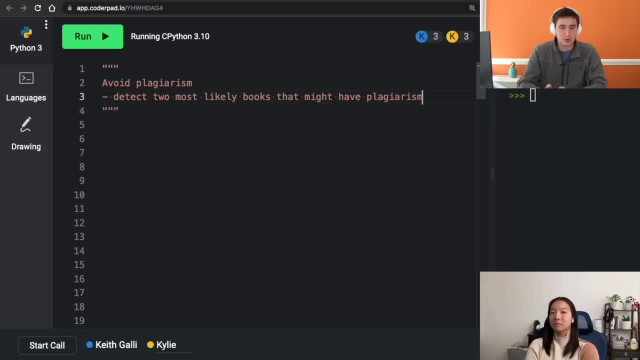 we can define as we can define most likely as meaning they have the longest shared, uh, common section of text. So we're looking, we have a library of books and we're looking for the two that have the longest shared common section of text And we specifically might want to know how. 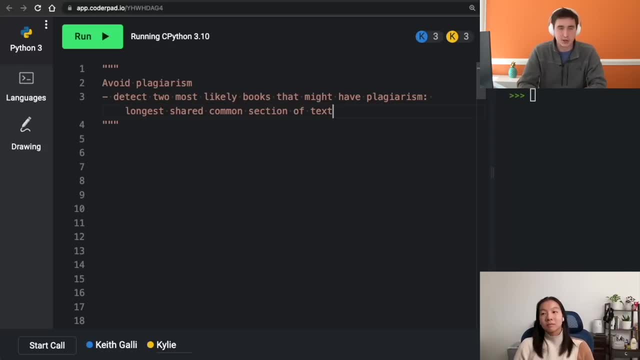 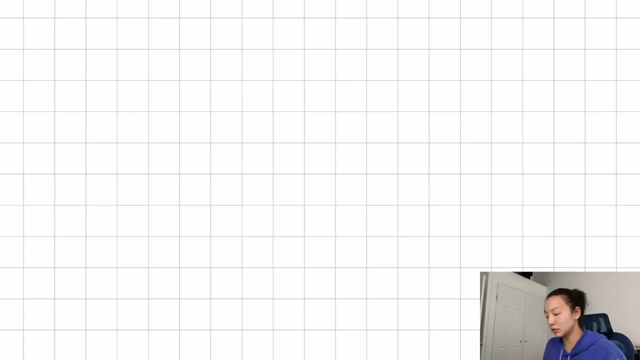 many characters that um section of text is. So you can imagine: if it's sharing a single word, obviously not an issue, but if it's sharing six paragraphs, that's going to be a problem. So does that make sense, Right? So just to clarify some things: what Keith really means here by substring. 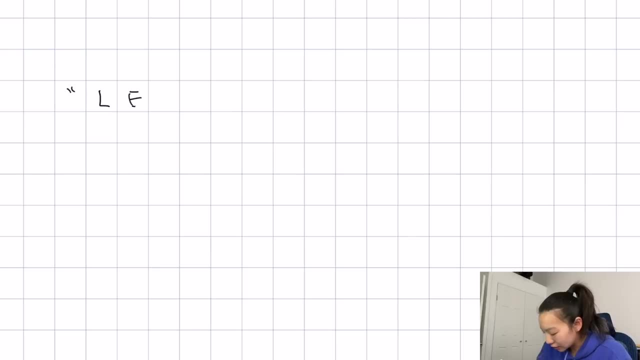 is that, for example, if you have a single word, you're going to have to divide it into two parts. So, for example, if I have a string such as learning, what are substrings of this? Well, one possible substring is learn. 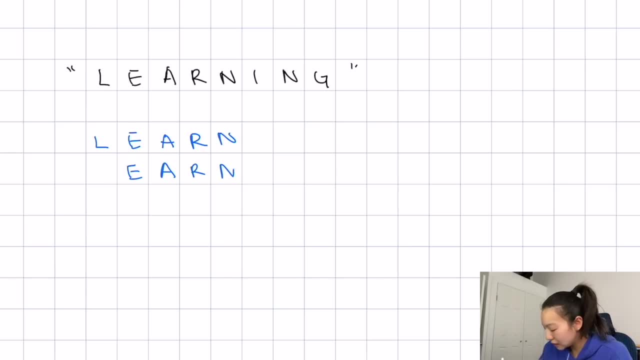 Another possible is earn, because these are strings that are using characters that belong to this string learning. Another possible one is earning. Oops, Now you might say, okay, Kylie, all of these are consecutive in terms of the characters. So here all of these correspond as characters that are next to each other. But in this specific example, 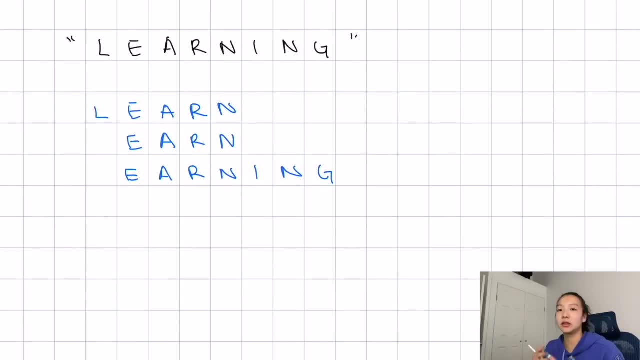 Keith is not actually asking: okay, it has to be a consecutive substring Instead. What Keith is asking is just any substring, which means that as long as the letters are in the correct sequence, you can skip characters if you want to. So, for example, here leg would actually also be a substring, or? 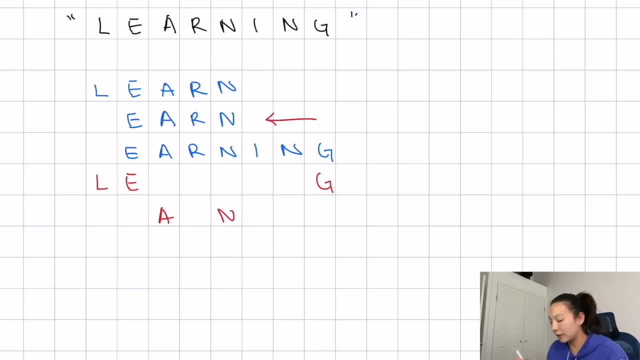 an. So, for example, right here we have earn as a substring of consecutive characters, But down here I could rewrite it as a substring where there's actually a gap of two characters in the middle. But this would still be a valid substring, So it doesn't have to be consecutive. 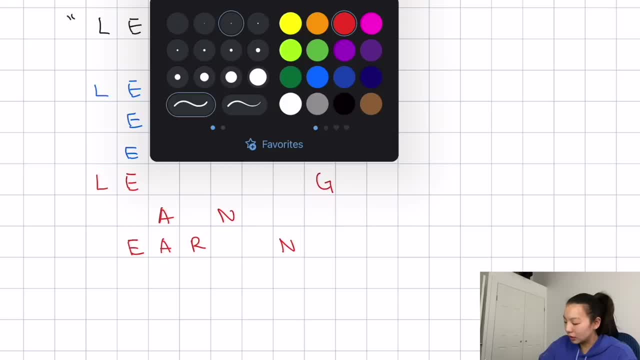 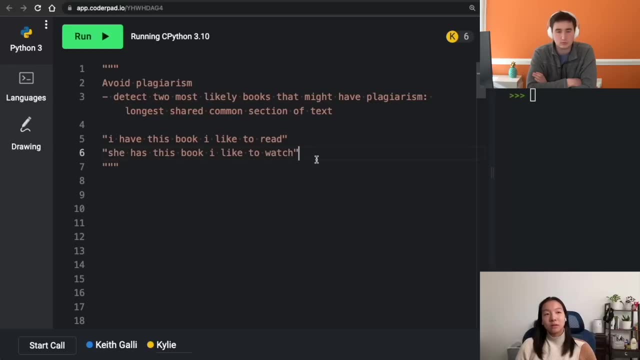 we just need all the characters to be in order from left to right. Let's see. let's start off with kind of a naive solution for that. Well, one thing that you could do is literally come up with every single combination of like substrings for both of these And then compare those and see. 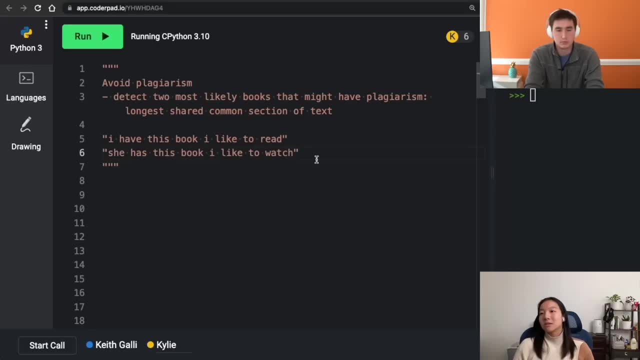 which two substrings are correct And then compare those and see which two substrings are the longest right. But there's a lot of different combinations for substrings, And so I think that we should come up with a more elegant solution. Let's see. So one thing that I'm thinking is: 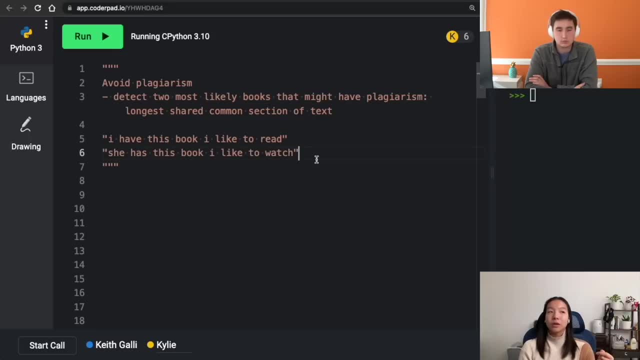 we should have pointers that start at the beginning of both strings. And we should have pointers that start at the beginning of both strings And kind of move along until one of them detects a shared character. So, or like when, until one of them detects like the first shared character. So here actually, 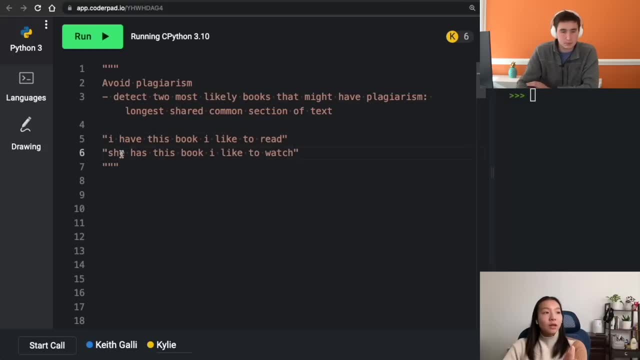 like I would say, the first shared character is H, right, And so here we would have like like the two pointers kind of be this: Maybe I'll go from the bottom, but here and here right, And so we look at the next character. 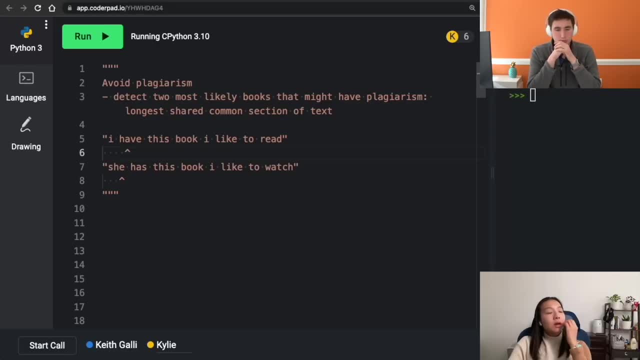 and we realize, okay, they're not the same, So then we want to keep going. But one downside of this is that, well, okay, What if I want to start comparing from here and here? right, Yeah, Okay. And then I move it over and these two have two shared characters. So I think that 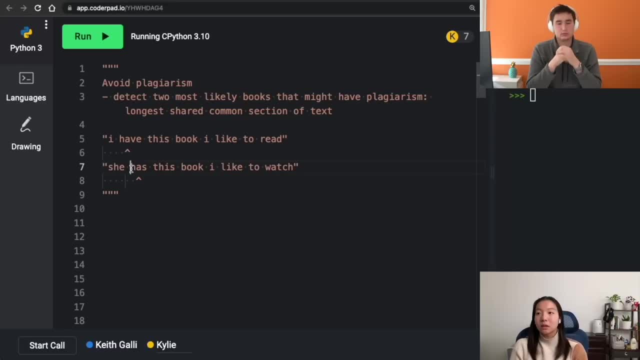 there's still this question of there's a lot of different combinations here. I think you're on the right track, though I like, I like these thoughts so far, And then okay, Yeah, Okay Yeah. So I know that here I want. all of these individual patterns. so here I can just try to go from here to here. I want the two. So I think you're on the right track there. I like, I like these thoughts so far. Yeah, Okay, Yeah, So I know that here I want kind of these. 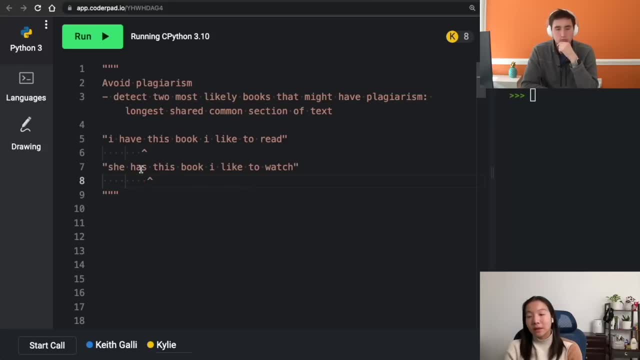 Okay. So I know that here I want kind of these, kind of these pointers that are moving, and then i just want to be able to align them right. i think that's the that's the key here is this alignment, and so now i think we just have to figure out how to make that alignment work. um, 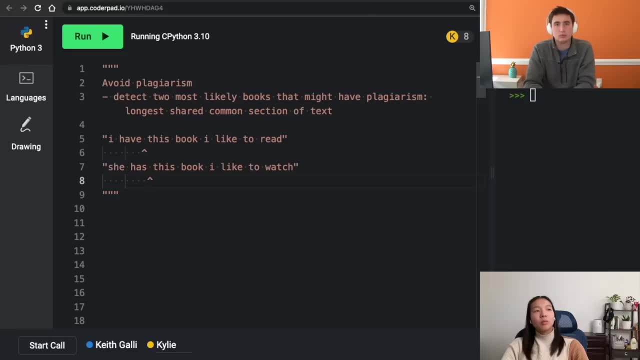 i'm kind of thinking like like one thing that we could do is kind of have more of a base sentence and then one where, when we have like, so, for example, if i, if i made this my base sentence, then in the other sentence i would want to search this sentence. 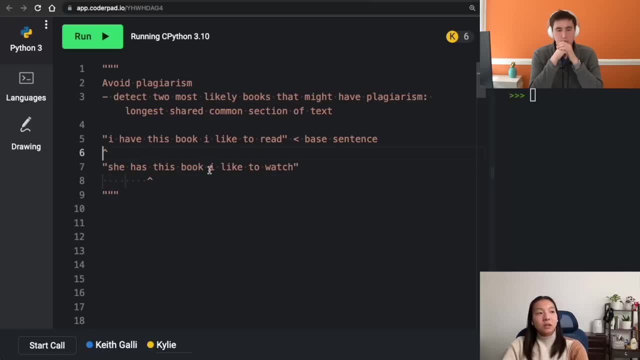 uh, for each character. so if i have the eye here, then, like my first, i would start looking from here, and, And then maybe I would start to look from here, Right, But I think that that would end up also being kind of long, because for every single character in here. 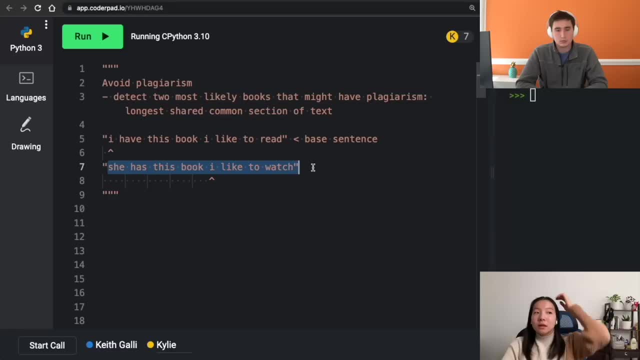 you would have to iterate through this entire thing and do the whole matching process, And so does that make sense. why that's like maybe not the most optimal solution. Yeah, that makes sense, And I guess what would be the runtime of that? It would be O of N squared, because well, I guess, if we have one sentence, O of N. 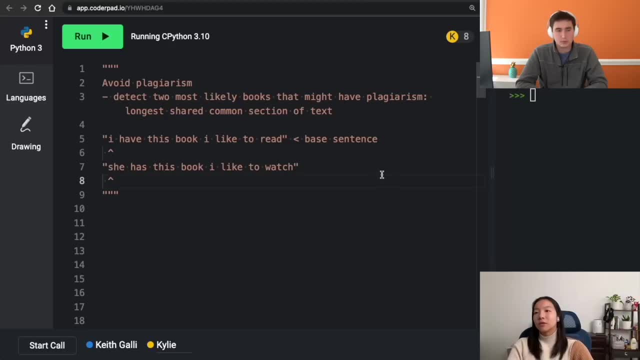 and one sentence O of M. it would be O of NM, because for every single character we'd have to run through the other string M times And actually okay. so like, if my base sentence is like: like, what is the worst thing that can happen is like a base sentence like this right. 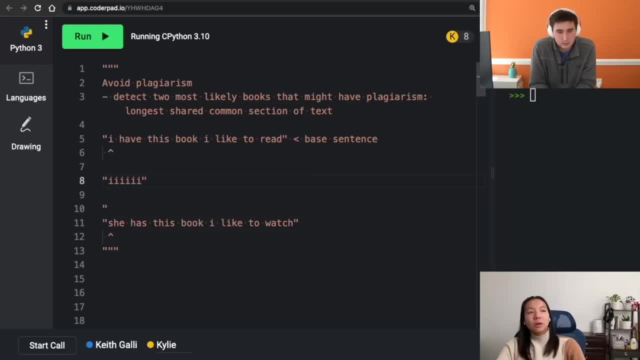 And then, And then you're searching. The worst case example would be like something like this right, Where, like, if I have an, I okay, well, I have to go through each of these And so, yeah, I guess we would have to go through until, like, they don't match anymore. 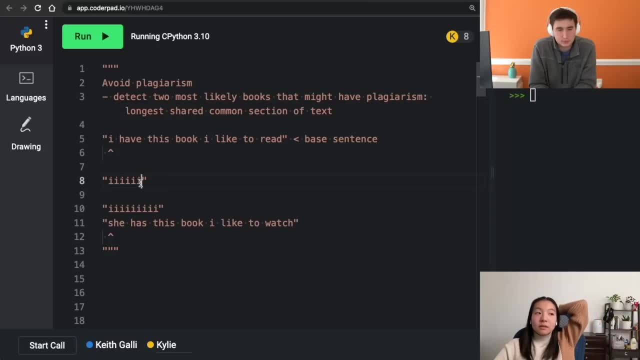 But then that would just be the very end of this, So like maybe I can add like an A at the end of that. So then I would actually Okay. So then Then I would say it would, it might be O of N squared M, where N is the shorter sentence. 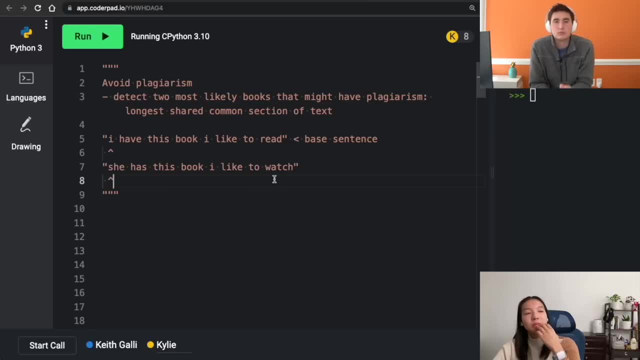 Yeah, I think that that makes sense to me. I think that we should come up with a different solution. I'm trying to think of how dynamic programming would work, because I do think that this, this might be a dynamic programming problem. I'm not sure of how to formulate it. 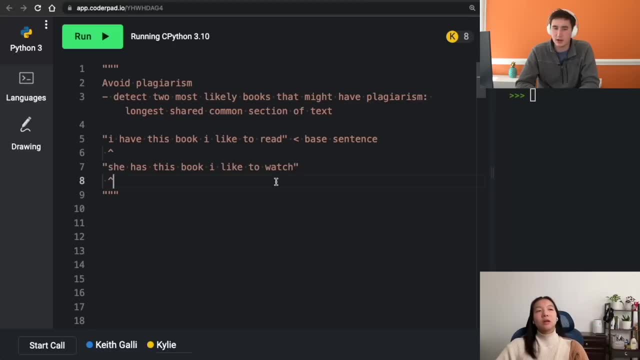 Yeah, let's. I think that you're on to something here. I think I'm trying to think of a good ways to kind of kick you off here. I mean, I would say let's just lay out, Let's assume that this is dynamic programming. 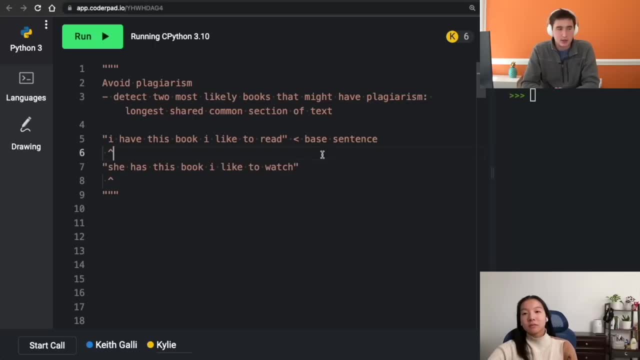 I think, as a good starting point, maybe we can talk about sub problems here and try to define that, And maybe that will help us get to our solution. or also maybe just to find a base case, And maybe that will help us get to the solution. 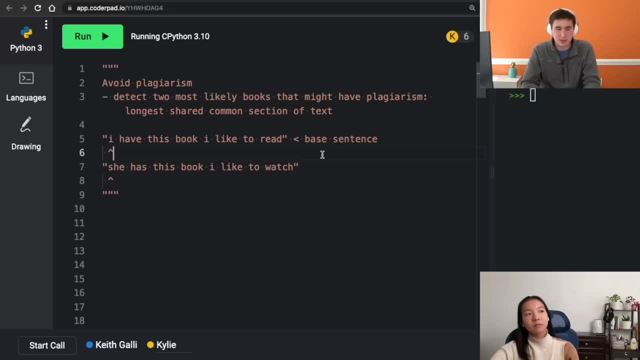 So I think let's assume that dynamic programming can be used here. Let's maybe just start trying to figure out sub problems and maybe a base case, Yeah Yeah. So I definitely think that the base case would be pretty simple and it would just be if there is a match right between the two. 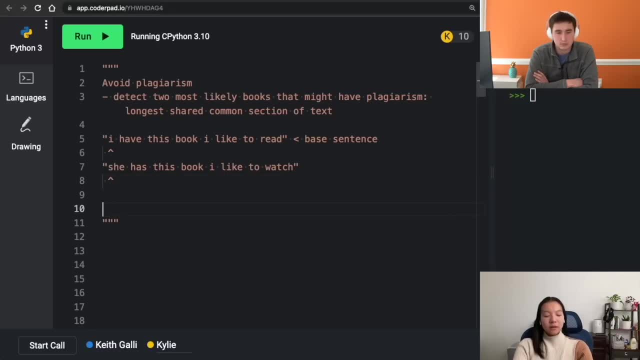 Like if the two sentences equal another. that would be, or let's think about all the possible base cases. So it would be if there's a match, or maybe we've iterated through Everything that we can and we're comparing, like an empty string to non-empty, or even empty to empty, which is when we would know that we're at the very end. 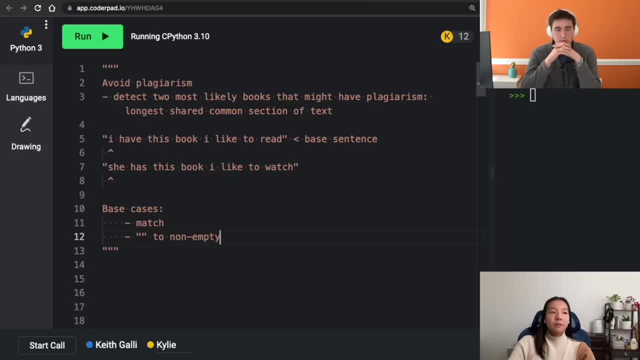 Right Yeah. So for example, with this match, I mean by like, read to read, like that would be an exact match. So I think the difficulty of this problem is, that is, that we can start anything Anywhere in the texts. 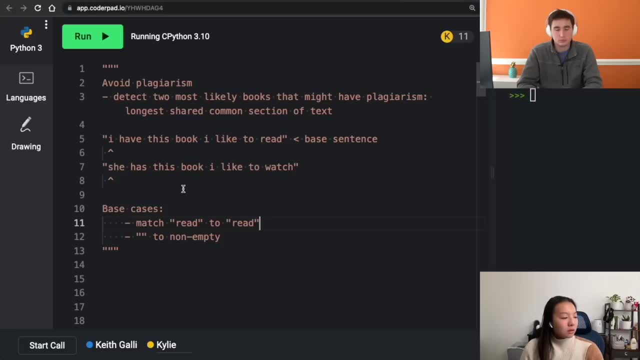 Right, And I guess if we were trying to recurse through this, Or if we, if we were trying to go through this with dynamic programming, What I would kind of want to do is Say, Okay, Either like Like S is the start of some substring in this sentence, or it's not right. 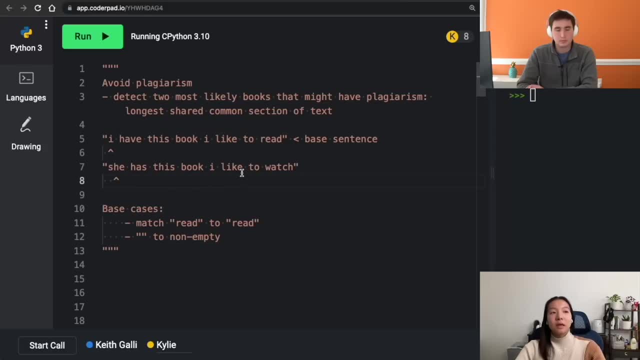 And if it's not, then we want to move over and we want to say, okay, well then is like H is a substring or the start of a substring from this other sentence or it's not, And we want to kind of continue that process. 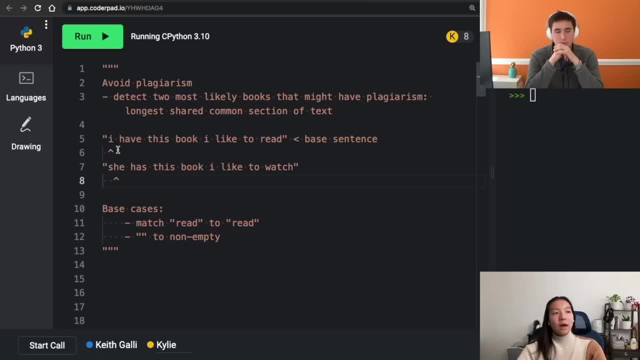 And so if, for example, H is a substring, Then We would want to figure out what the longest substring, longest matching one is. And then that would essentially like: skip us over a few Yep, A few blocks. And so I think another way to kind of formulate this might actually be like how many, how many characters can kind of almost subtract from the two. 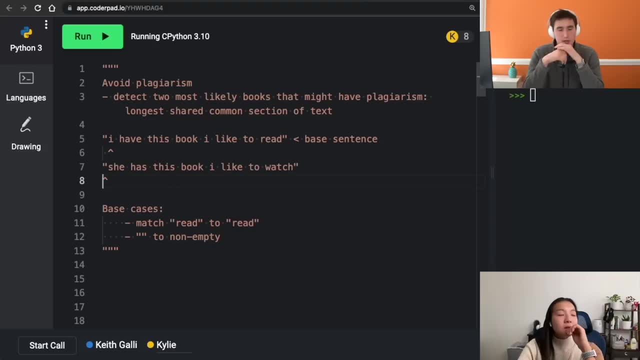 Yeah, yeah, Um, And I might, I might jump in here. just I think you're on the right track, but I might provide a little bit, maybe more, of a launching point, Just because I want to be considerate of our, our time here. 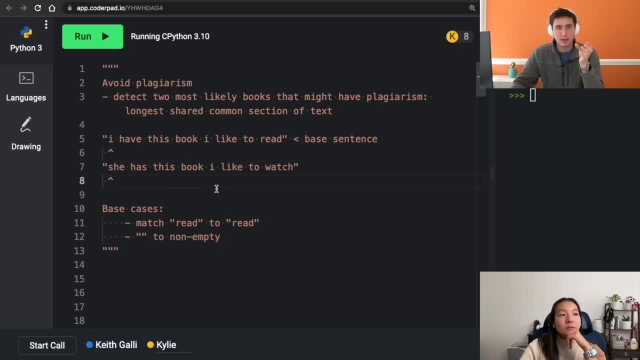 Um, I think you're on the right track. I think that let's maybe try to define this like with a single line expression, like a single line recurrence type expression. Um, because I think that if we can build up the, We can build up the. 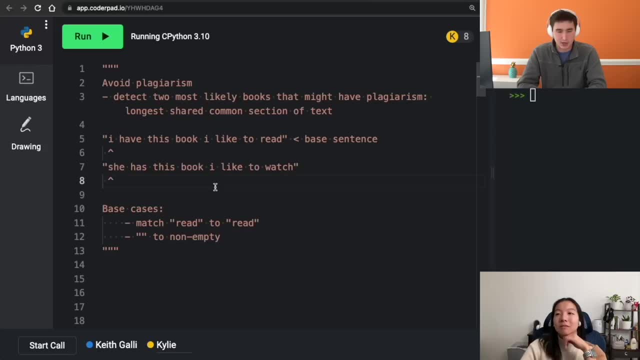 To a. you know build up some problems to that final state. that will help us. So let's say we have sections of text a- And I'll put this in- could see where we have. a is one of our sections of text And B is another one of our sections of text. 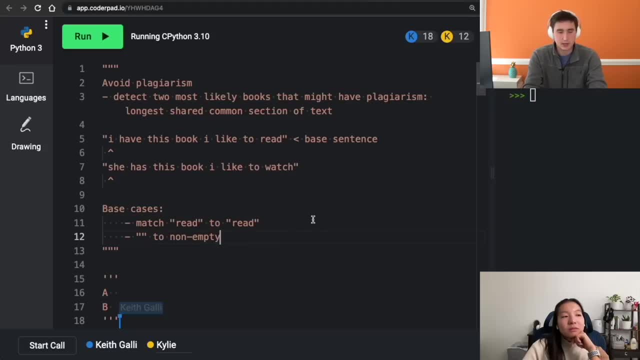 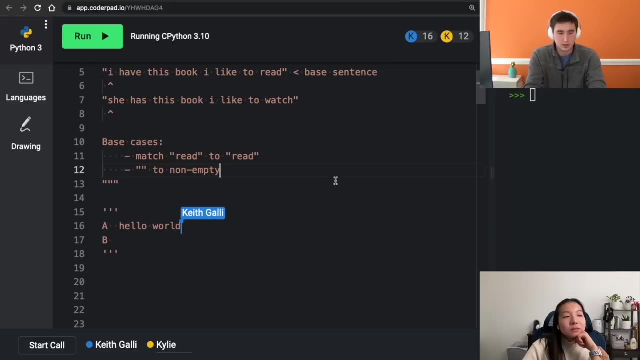 Um, And basically that could be a hello world or something you know, and world, Uh, just world, or something like that. Um, we can assume that. Yeah, basically what we could start doing here is we can imagine that we wanted to find the longest match between A and B. 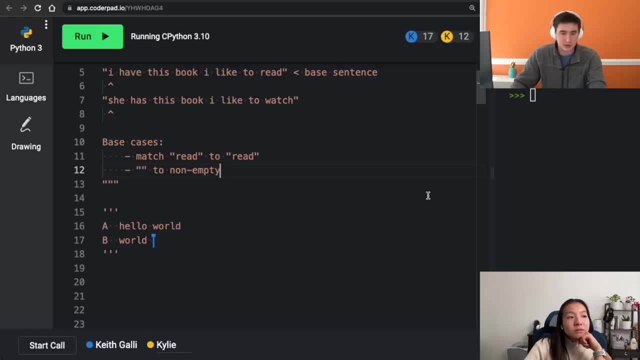 And you could define that as from character index zero to character index zero here. So like the longest common sub sequence here, or substring of A, B, zero, zero would be our kind of goal state, because we would want to find if we're working backwards, let's say we want to find all the way to the beginning. but to help us get there, you know, we could probably see if, uh, you know what is the longest substring at different indexes. 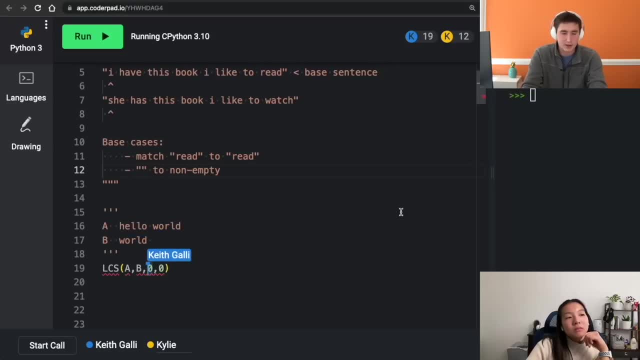 So, if you know, maybe index three, index five, so like this would be the, I guess, last character five would be like the last character of B And I guess, keeping this in mind, can we define this in such a way where we maybe we can uh define an equation that would help us work up to that final goal, which would be the entire sequence. 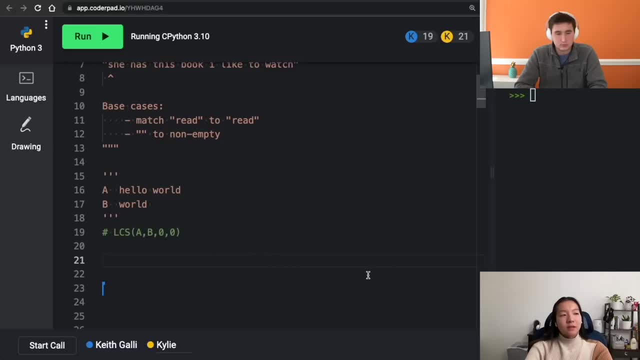 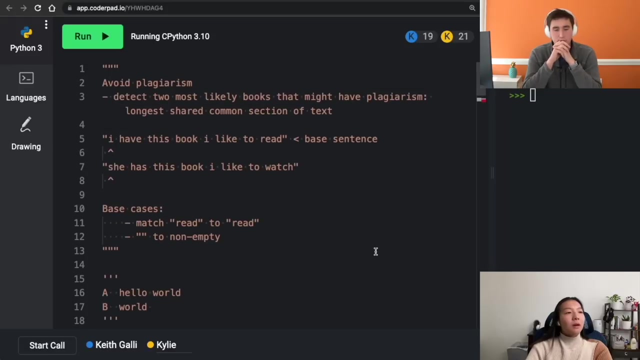 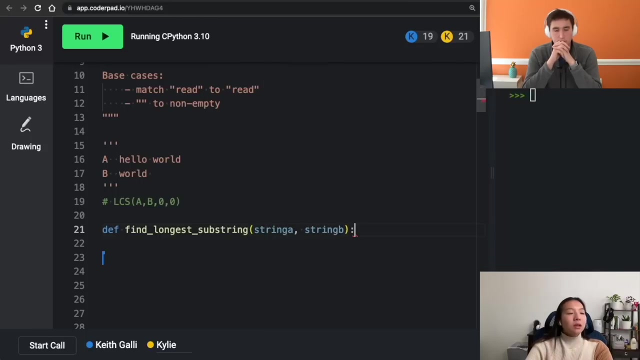 Okay. So if we're using kind of these AB strings as example um, let's define some like like Find uh longest sub string or something, Um, and we might have string a, string B, right. So and you're saying: okay, let's do index a and index B as well and start those off with zero. 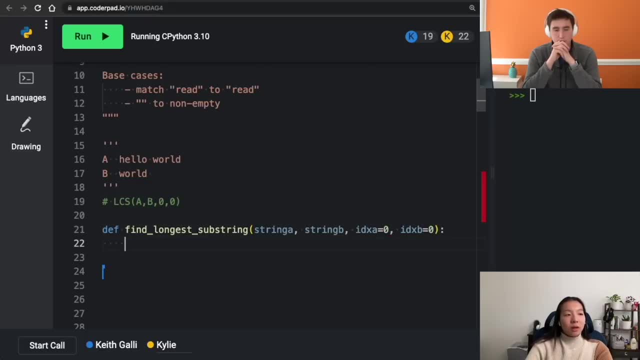 That would be our recurrence relation, And so I guess what we'd want to do is find the longest substring between Um, yep, these um, and we want to increment one or the other Yep. Right, So like that, uh. 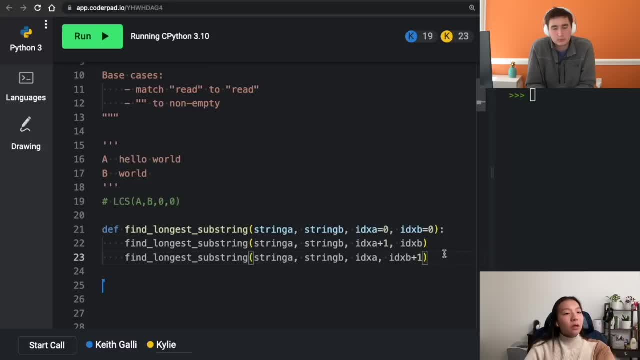 or, or. if string a equals string B, then what we'd want to do is find the longest substring. Um, we want to increment both of these indices apparently. oops, sorry. So I meant string a at index a and string B at index B, like this: 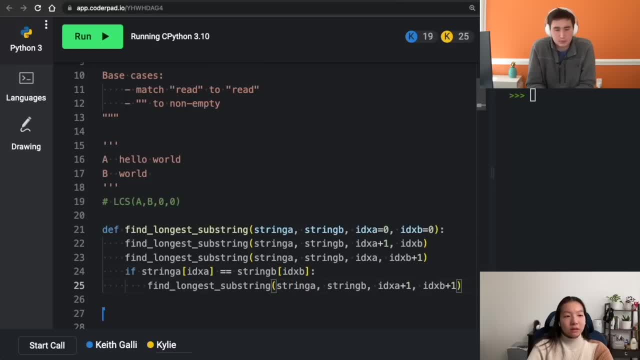 So then, we'd want to increment both of the indices and we want to add one right, Because This means that we've, uh, found a starting match, Um, and what we'd want to do is actually take the so here, um, and if you want to just write pseudocode here, it's fine to for me, uh, possibility. 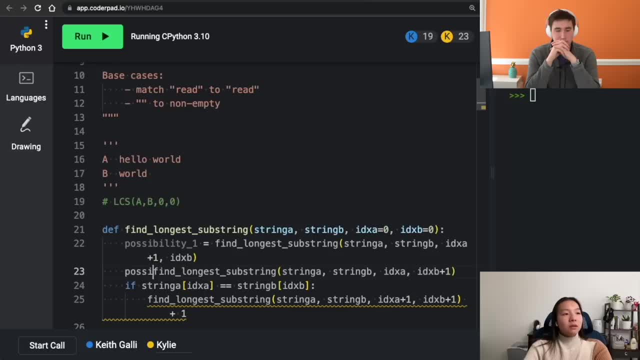 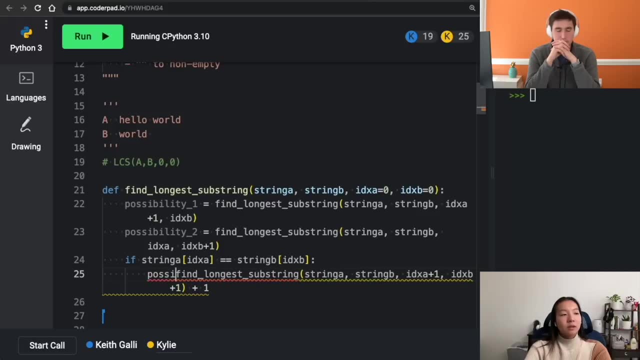 Okay, That, that that makes sense to me, Yeah, So let's just do All these possibilities And so then, if the two, then we have this like third possibility, right, And what I would want to do is, uh, take kind of the minimum. 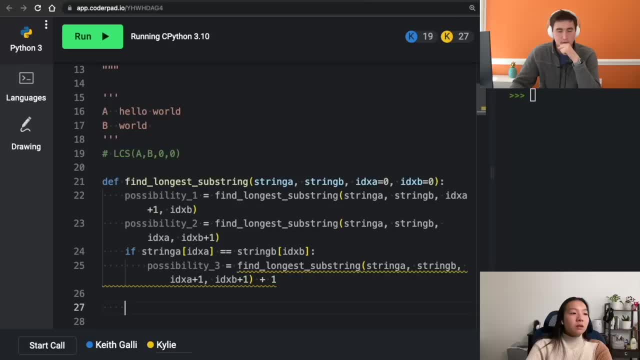 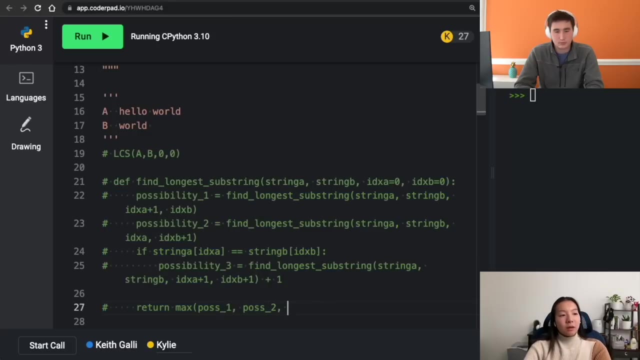 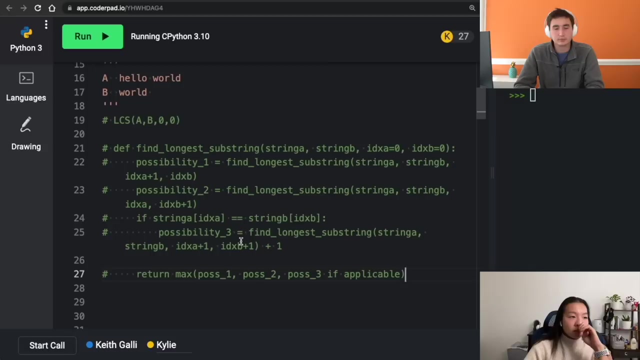 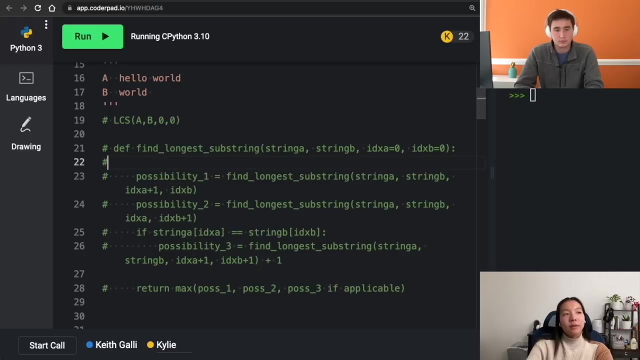 Why is this giving me an error? Oh, so then I would re. I would want to return the max of possibility. One possibility to- okay, let's write pseudocode possibility. One possibility to, and then Possibility three: only if like, if applicable, um, and. and then, with our base case, we said that it would be if one of them is at the end. 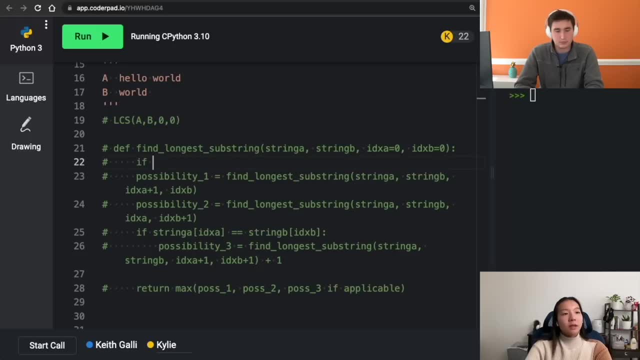 So let me add that in here. So maybe like, if, uh, IDX a is equal to the length of string a, then we want to return zero, or or Hold on More, Okay Here. or IDX B is equal to the length of string B. 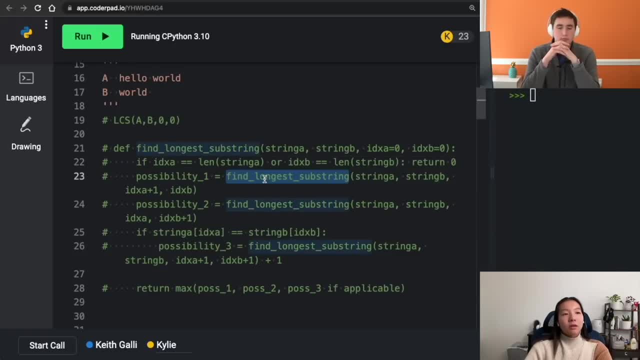 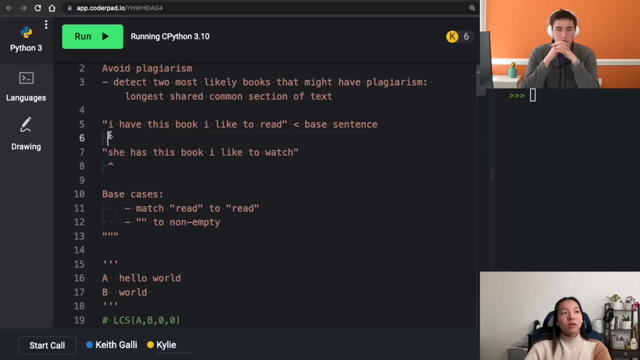 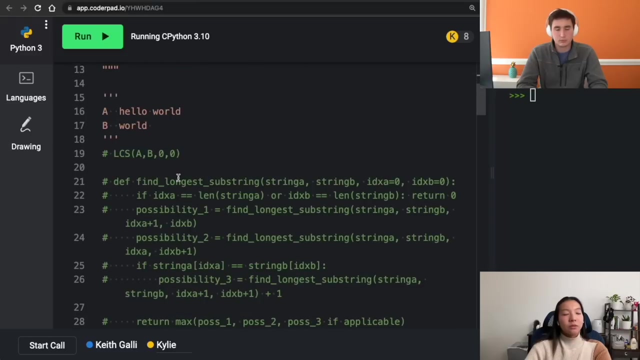 Um, yeah. So then for our longest substring. this makes sense now because with each index, we have the possibility of shifting it over one and trying to compare this sentence with this entire one, uh, or shifting the other one over one, comparing those two. 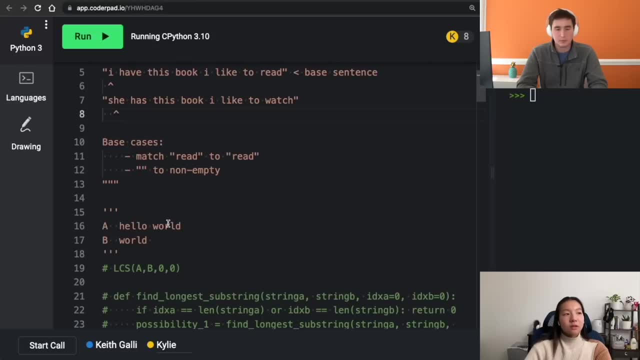 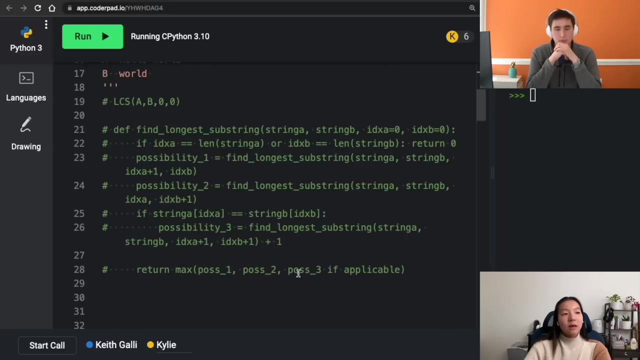 Um, yeah, Indices, or those two substrings from there on, or if they are a match, then we also have the third option of moving both of them over. So actually I should go from here and then, because, uh, this fine longest substring repeats all that on the next character for those two, then we repeat that process again and we add one every single time to that. 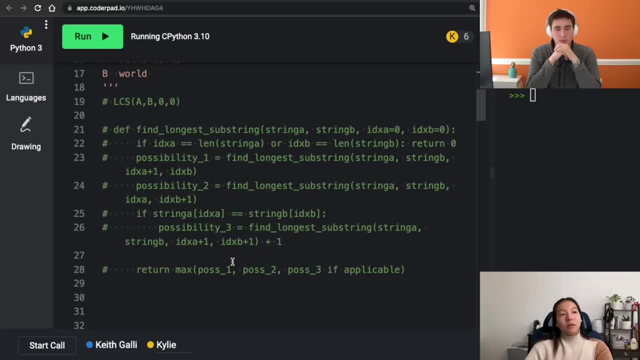 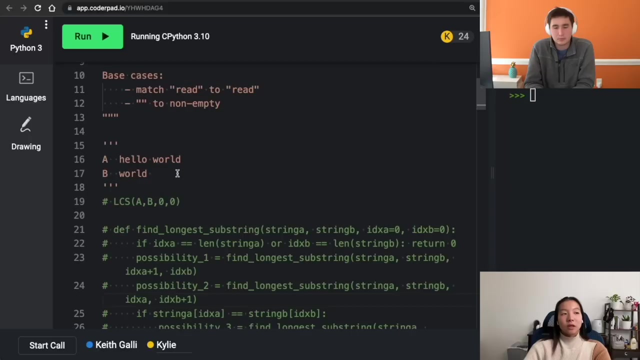 Um, so I think logical, Logically, this makes sense. Now, one thing might also be that we start to kind of recurse a lot on the same indices, right, Because we're trying all these different combinations And if we move them both over by one then we kind of are iterating over through them a lot. 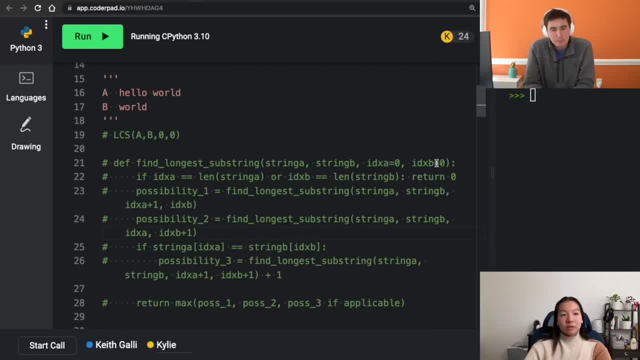 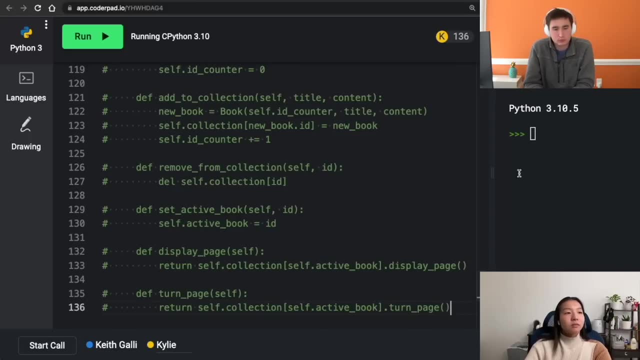 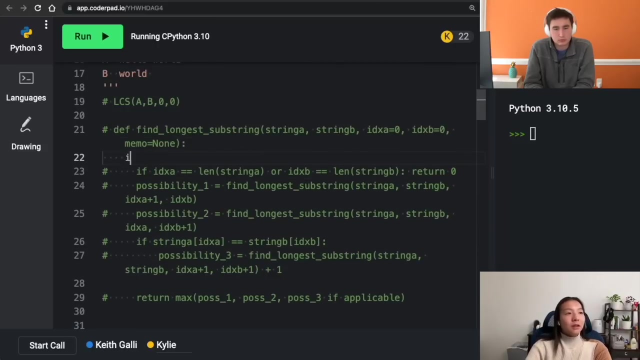 So I think that one thing that we could also do is implement some sort of memoization. So here, like maybe—hold on, I lost the—oh, here we go, Okay. so then, like, if I—so if the memoization is none, then we might want to start this with some sort of—. 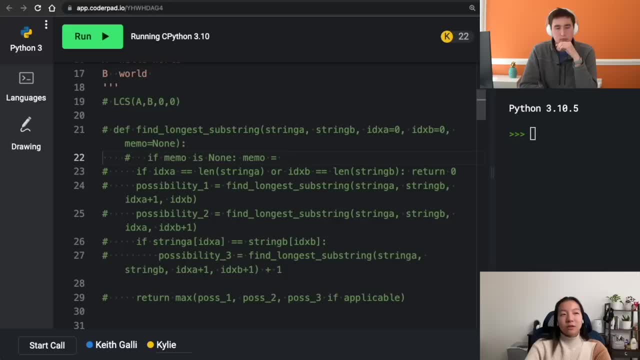 it could be a dictionary—I think that also. what could make sense is like a list of lists, right? So like maybe negative one, because there's no such thing as a negative one-length substring, And I'm going to multiply that by the length of like string A, for example. 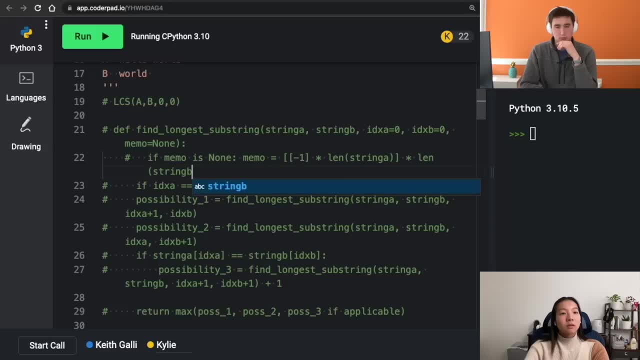 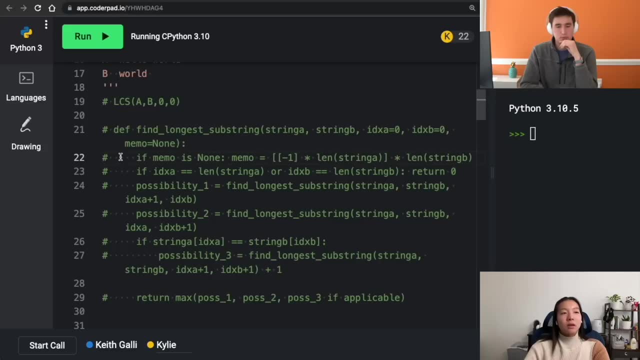 And then this whole thing by the length of string B, And so essentially I have this table of— Oh, it would be string A this way, and then string B down. Yeah, I always get confused with the direction of these things, But I understand the goal of this: length string A and length string B. 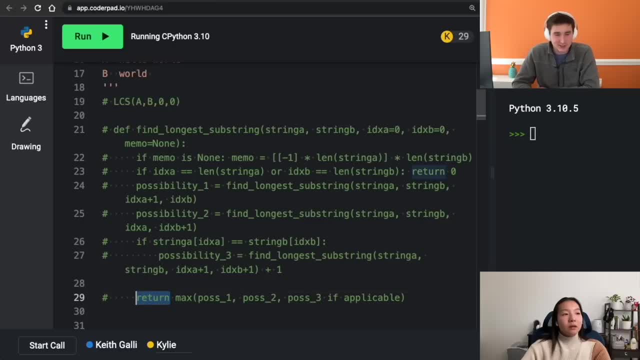 Basically create a table that stores some of these values. Yeah, exactly, Yeah, Yeah. and then, in order to store that here, then we would want to create, like the index A, index B- I might be—these might be- backwards. 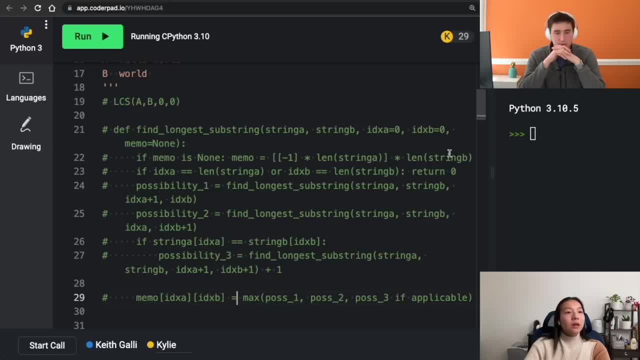 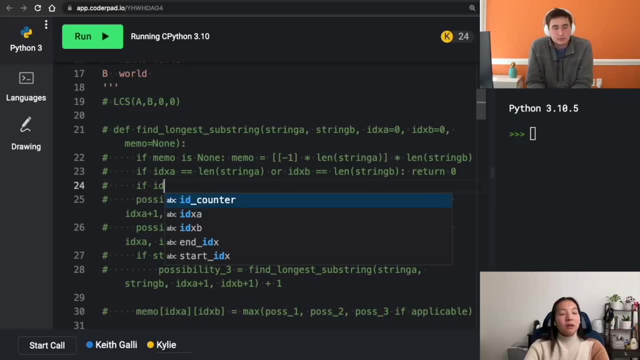 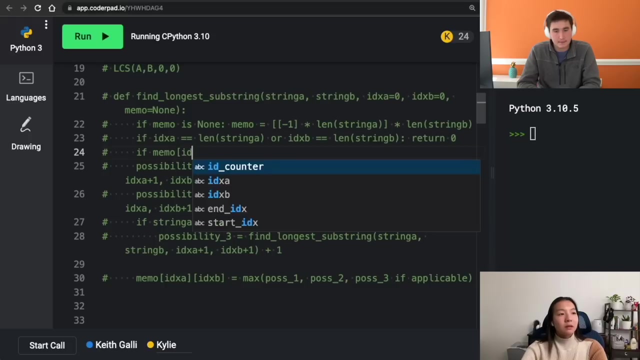 But we would want to store that essentially. And so then we'd want to add a case of like: if, like this memo at index A, index B— these might be backwards again. If that's negative one, then we want to return—or sorry, if that's not negative one. 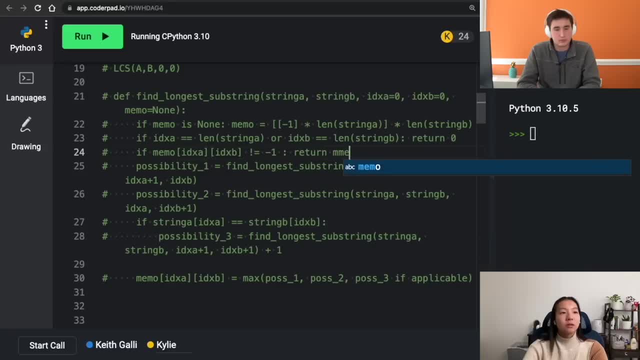 then that means that we— we've already found the answer. So then we just want to return whatever we've memorized there, And so at the very end we'd want to just return memo like that. And let me just think about these indices quickly. 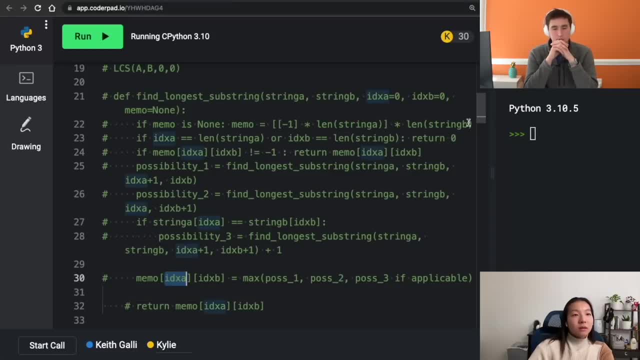 So the first one is string B. So actually, if I just swap these two, that should make it work. Okay, Because first we'd index into A and then we'd index into B, Yep, So yeah, Yeah, if I just swap those two, that would work. 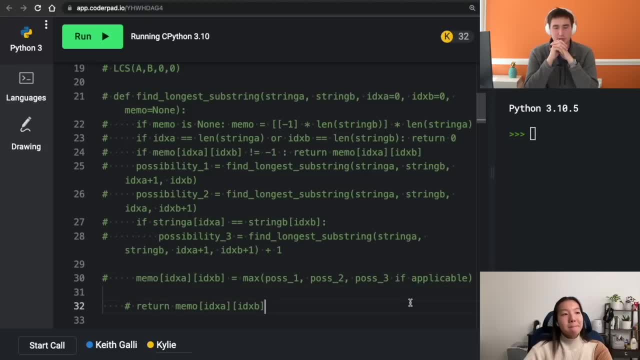 Cool, Yeah, this makes sense to me. I guess my last question—I think that this is the approach that I was kind of thinking about as far as dynamic programming goes- My last question is: what would be the runtime of this, you know? 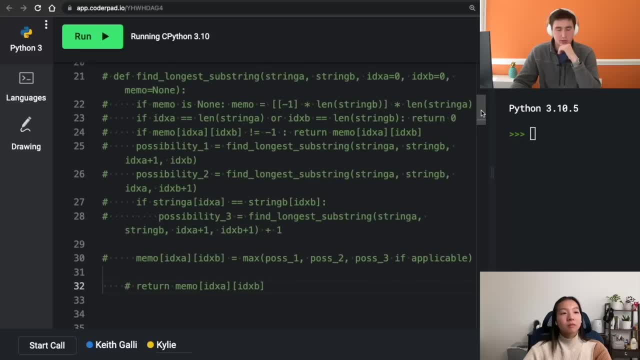 memoized dynamic programming solution. Okay, so here we are going through all of index A—or all of string A and all of string B- right by incrementing these indices until we hit a base case. So there's no way to avoid going through both of them and incrementing one, but not the other. 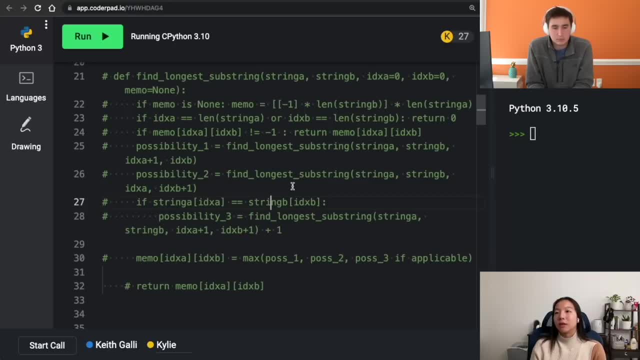 And so we essentially have to fill out this entire memoization table in order to figure out our answer, right? Yep, that makes sense to me, Which means that it would be O of n of n. And then my last question—I know we're running right up on time—is, I guess. 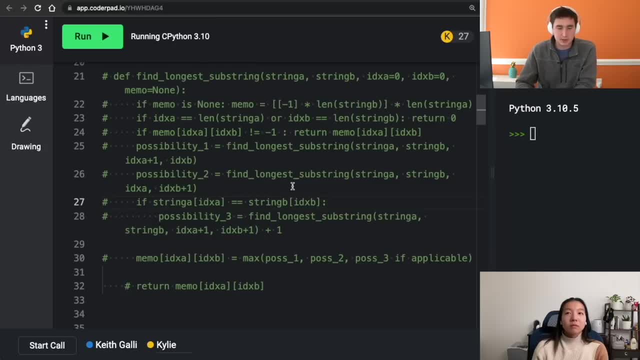 given. the context of the original problem was: you might have a library of books. how would you leverage this find longest substring to, I guess, find the two most like the highest probability matches in the entire library of books? I think that—so here, now that we have—. 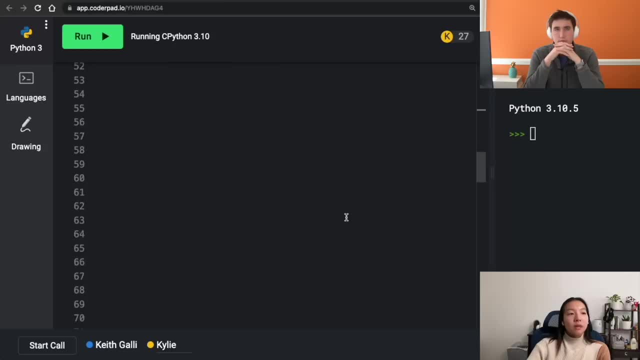 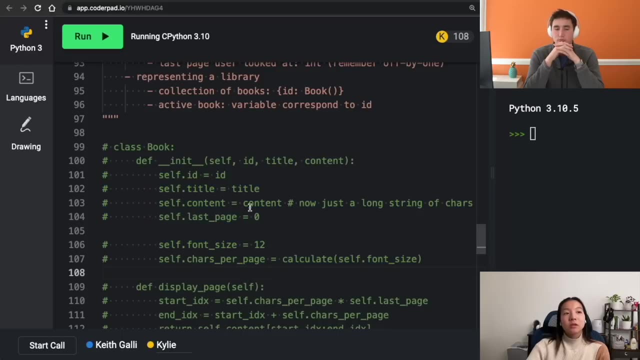 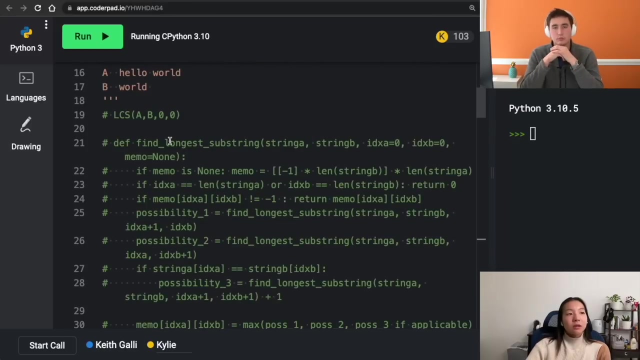 we have this find the longest substring with string A, string B, and we have all— we have—so we—let's suppose that we changed the implementation of this book to be this like long string of characters. for the content, then that means that what we can do for this find longest substring 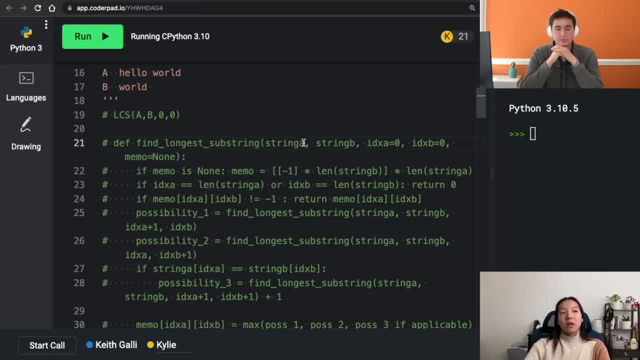 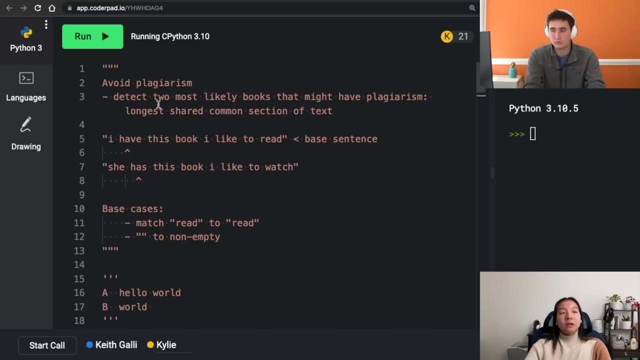 is just pass in, like book A dot content and book B dot content, and figure out the longest substring between the two of them. and we can do that for all the combinations of books- Unique combinations of books and if we find, for example—okay well, so the prompt is to detect the two. 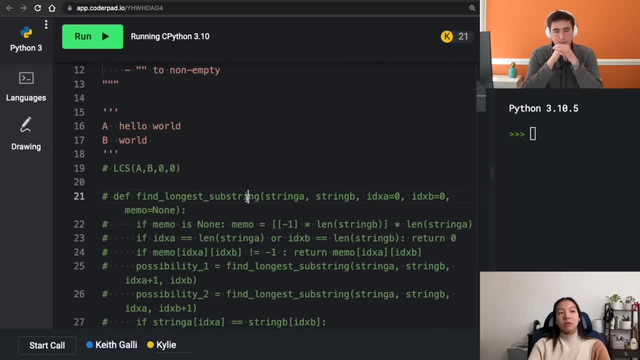 most likely books that have plagiarism. so we would just return the two books with the longest substring. but, you know, maybe we want to say like any—any books where more than 30 percent of the character—you know, more than 30 percent of the book is—or maybe even like 10 percent. 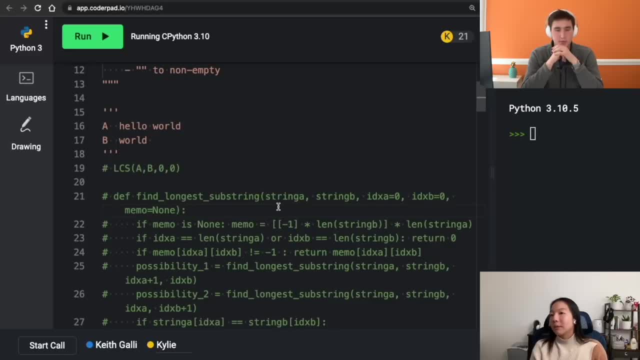 shares the substring. Yeah, Yeah, So it's the same substring than like we might call the plagiarism or something like that. Cool, That makes sense to me. All right, That's all I have. Thank you for your time. 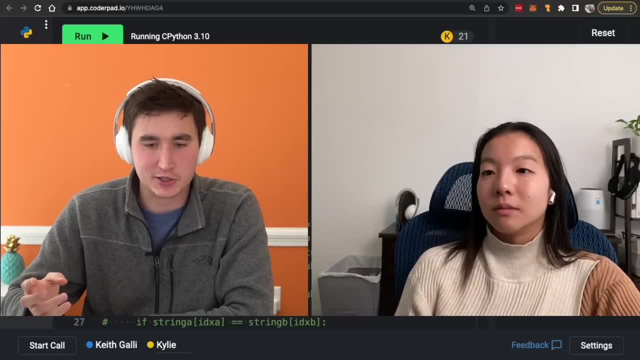 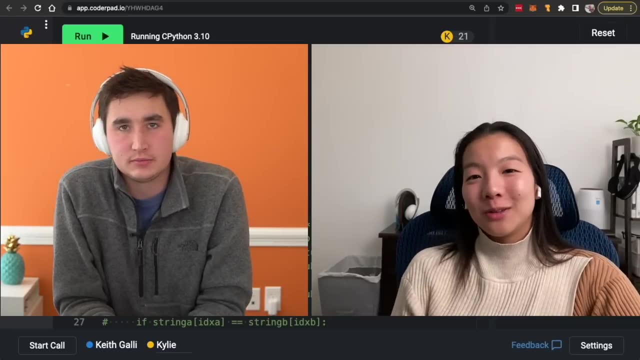 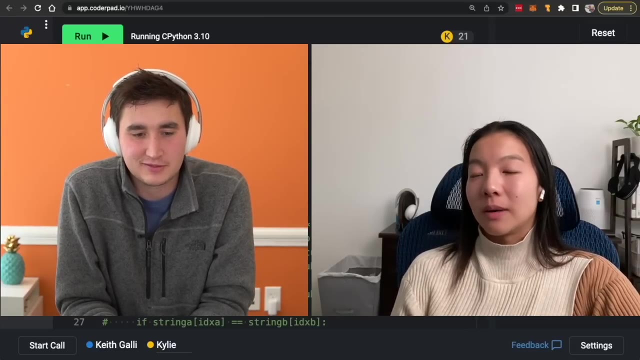 I guess quickly. do you have any questions, I guess, for me, or any questions about these prompts before I head off? Awesome, Okay, so note to the audience that in a normal interview this would be a time when I would dive deeper and ask questions about you know Keith's work or what you know he enjoys. 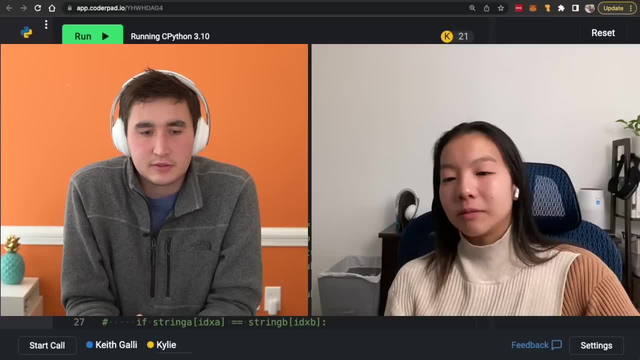 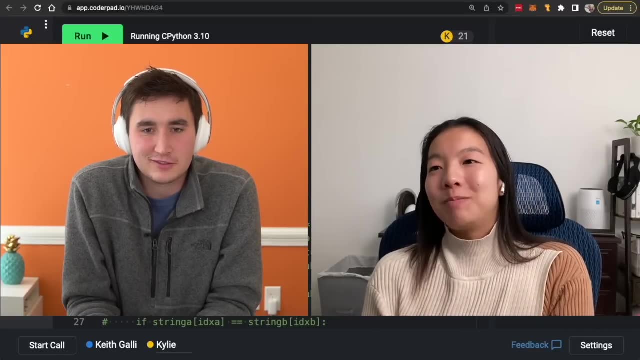 about the company And if I, you know, find something in one of his answers that I'm really interested in, I'll dive into that a little bit more. But because this is just a fake interview and I don't really have any questions about Keith's company because the company doesn't exist—. 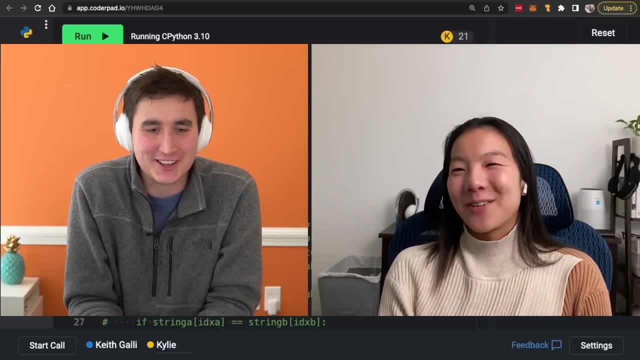 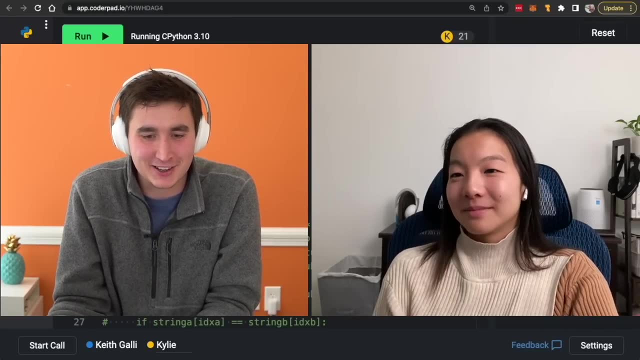 Yep, That makes sense to me, And I did not give you any context really to work with here, so we don't have to repeat what we did with the video that I posted on my channel. But cool, That's where we can end the interview. Switch to the next one. 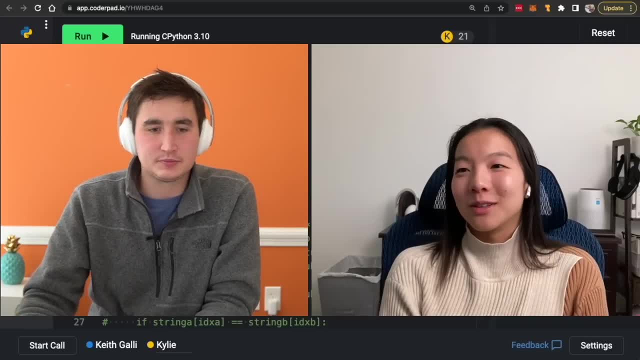 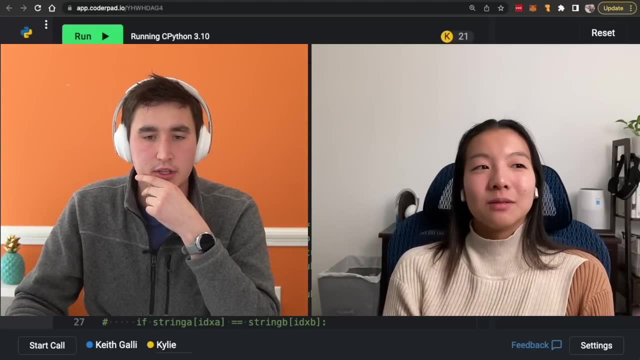 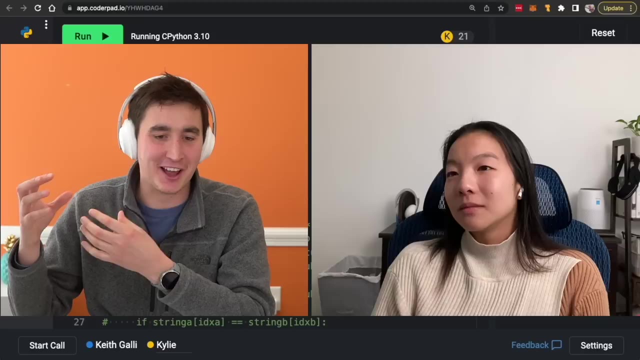 Switch gears. Yeah, All right. So now let's switch over to the feedback section— session. Do you want to go through your notes and kind of just share what was good, what was bad, your overall impression of the session? Yeah, And I think this was an interesting session because I like wanted to squeeze as much as possible into this, Like oftentimes you might see like a smaller fully object-oriented design or a smaller only algorithms. 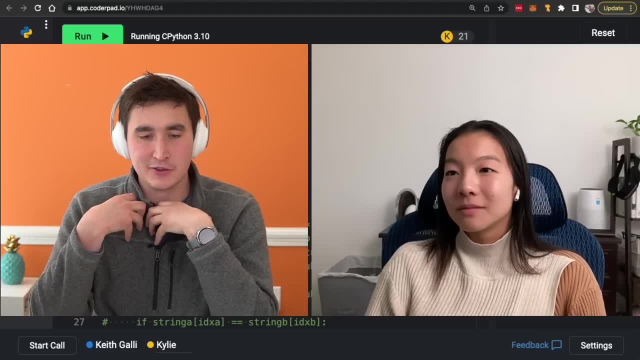 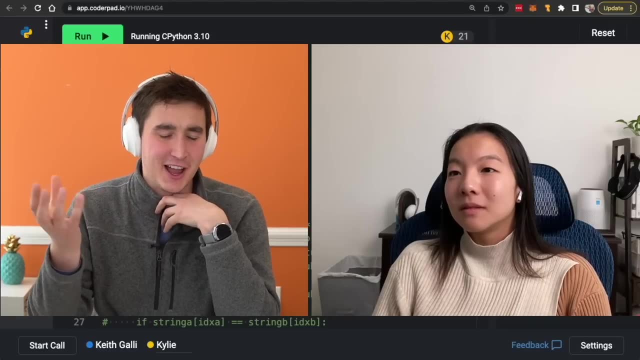 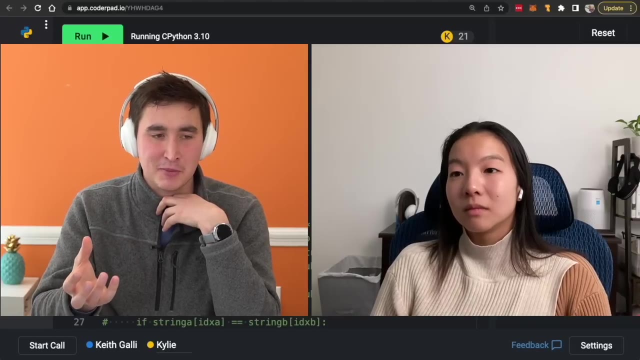 But I kind of wanted to get both because ultimately, from my perspective as an interviewer, like I feel like having— Yeah, both concepts is how I actually evaluate your programming skills, because a single algorithm doesn't tell me that much as far as your actual talents and like if you'd be a productive member of our team. And also the object-oriented design might not say everything either. 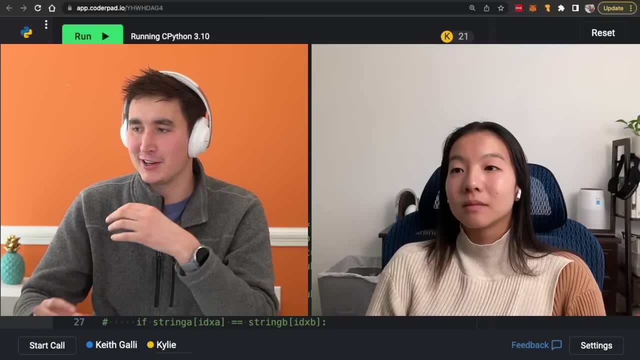 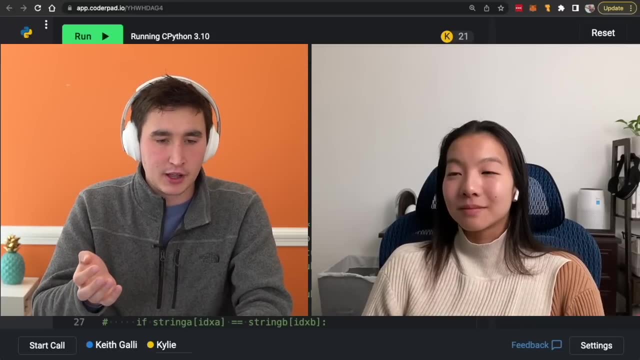 So I liked the combination but it was a bit like it is a lot of information. So, feedback-wise, let's start with object-oriented design, I think. solid overall, I think that you hit like the key points Yeah. 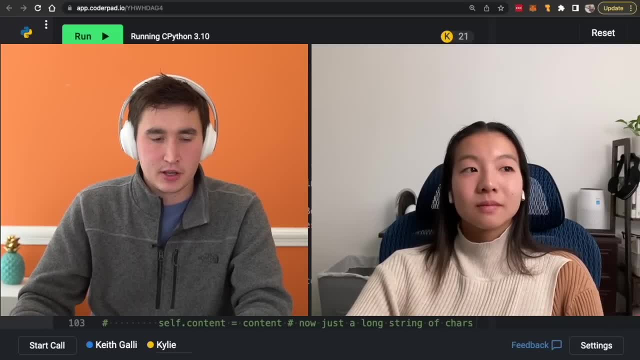 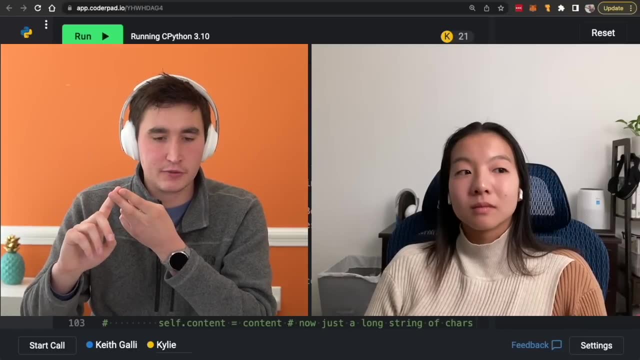 I think some of the things that I'm thinking about with regards to your solution is you hit all of like the key things that I was looking for. So, like all books in library, remember active book, remember last page in all books, display page in active book. 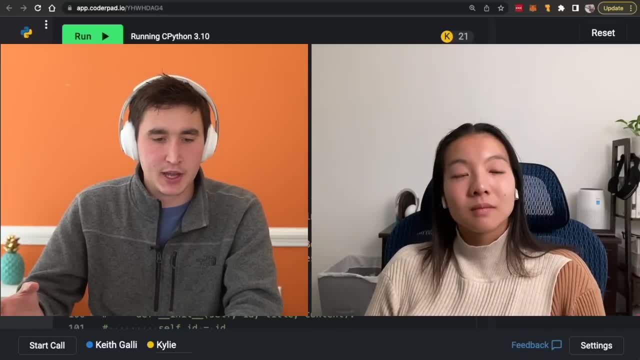 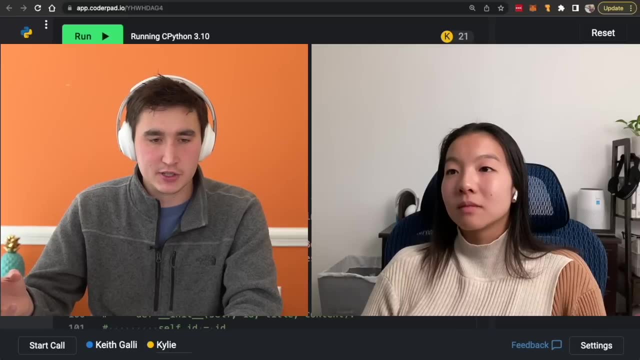 I think you did a good job with, like the basic class structure to capture all of that. I think what I would have liked to see- if I was to be like nitpicky and looking for even better solutions- is I might look for even further. 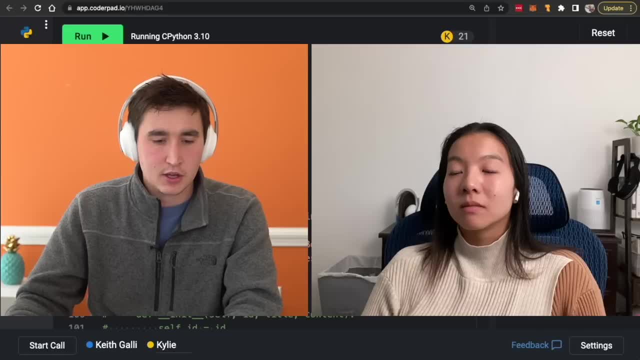 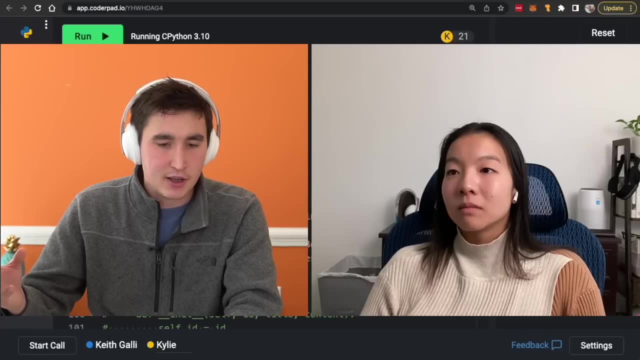 I think you did a good job with, like the basic breakdown of classes. So like I think there was some things that could have been broken down further, where I think maybe you could have a display class, even that could kind of separate the details. 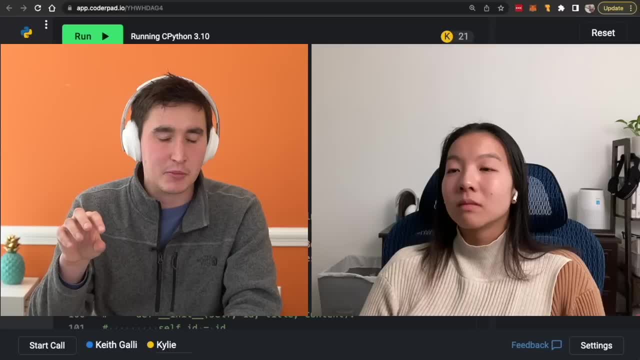 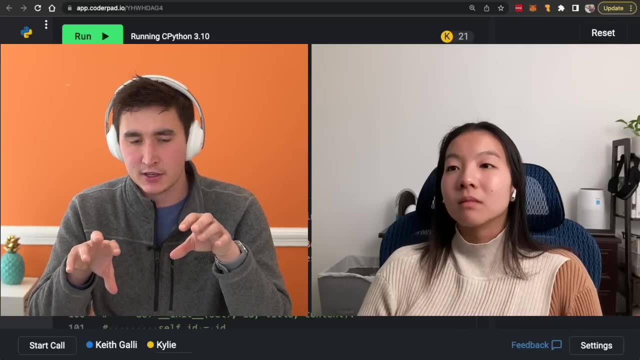 Like you have the book class that has the title, the content, but then the display class can handle like the font sizes, the characters per page, all of that, and just isolate that functionality. Yeah, Yeah, So that was like one thing that I picked up on is just, I think that it's tricky in an interview. 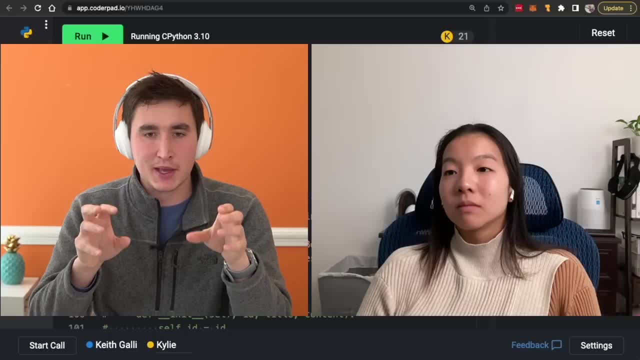 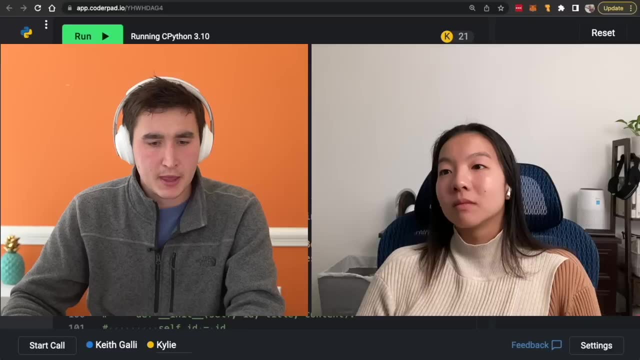 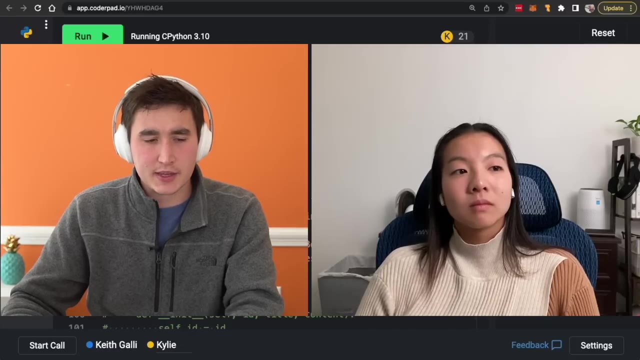 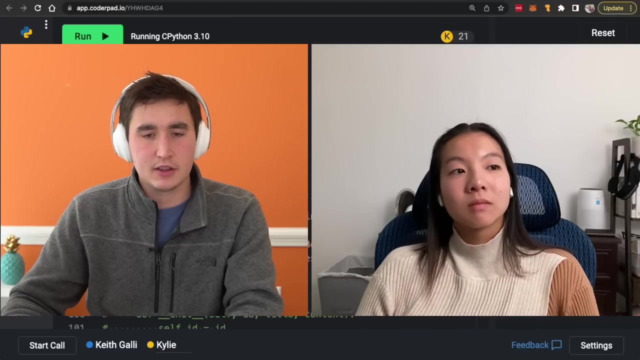 But I think that to isolate different components and make it easier to fit all together, I think further breakdown of these classes could have been beneficial. And then my other kind of like nitpicky comment in criticism would be like: I think the way that the IDs were structured wasn't necessarily like the most easy to understand. 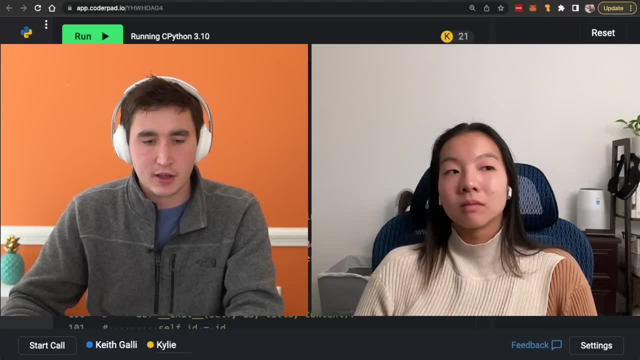 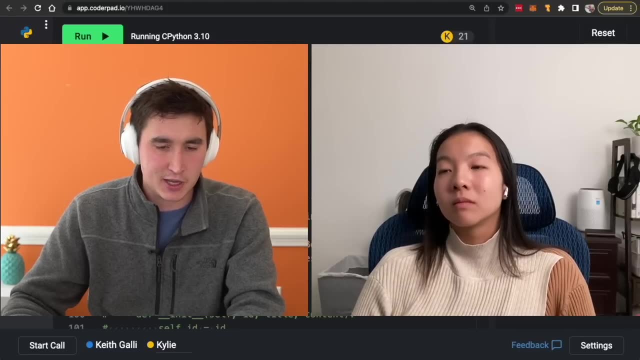 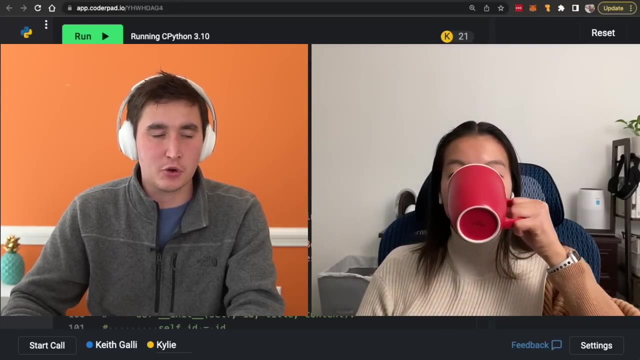 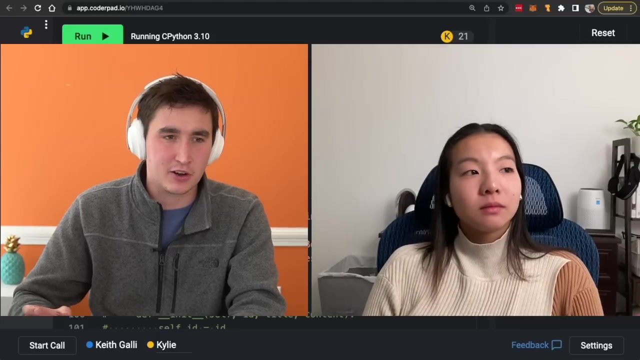 So I guess, providing some more details on, I guess, adding robustness to these IDs, I think like one thing that would have been interesting. I guess I didn't ask about this specifically, but the concept of like: okay, how could you then maybe if you only had a title in the book contents, how could you maybe grab that ID retroactively, or like: would you want to do that? 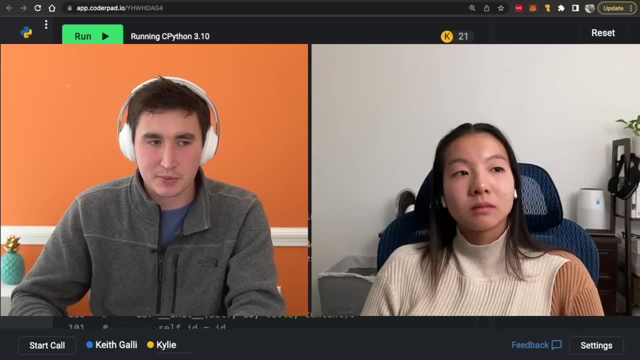 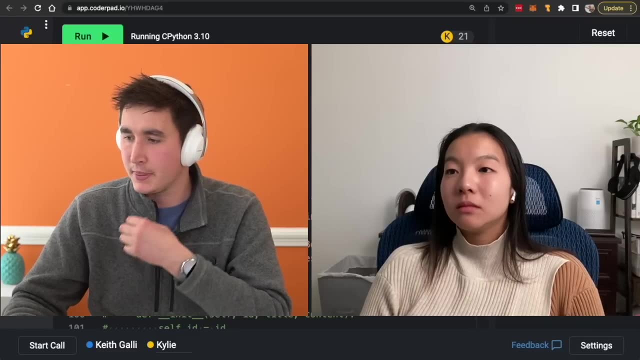 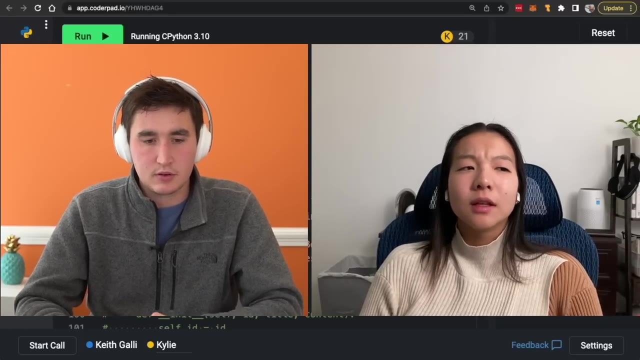 So like maybe some more robustness in how the IDs were set up so that you didn't have to have Yeah, Yeah, So the system to necessarily get an ID. Does that make sense? Yeah, Yeah, for sure. I definitely think that the ID part was one thing where it was. 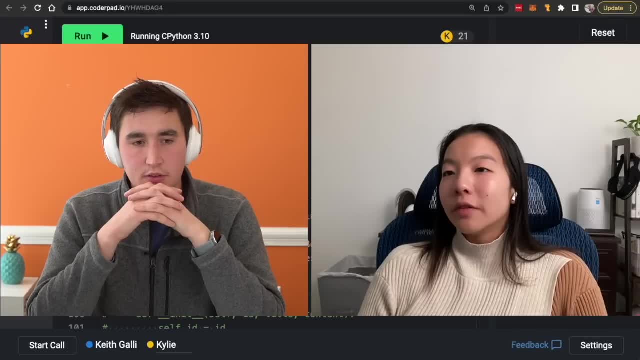 Yeah, Like I would have rather just used the title of the book or like some combination of like the title and author And I think like, for example, at like an actual library. they have like their code or whatever, and they have their system. 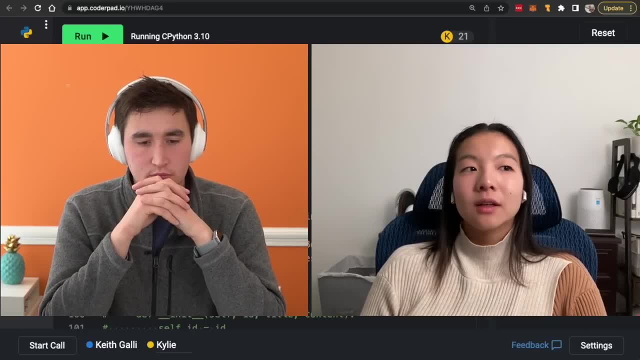 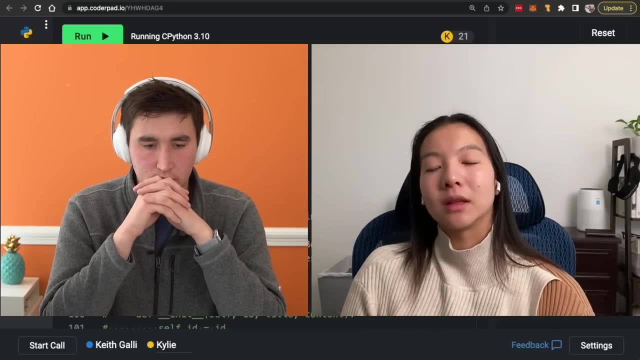 And for you know if it's fiction or whatever genre it is, and then like some combination of, I think, author that I don't really remember that they use to ID books And I think that that probably would have been like. a better solution is if we had like the title and author and genre. 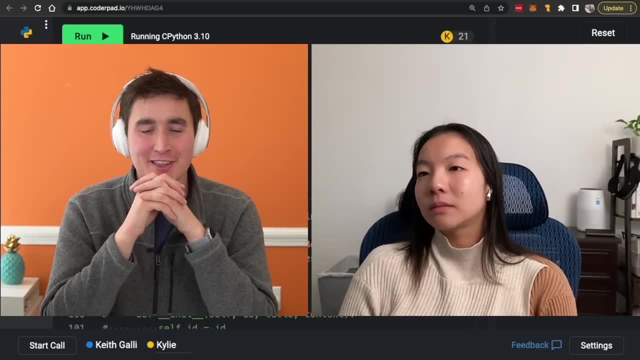 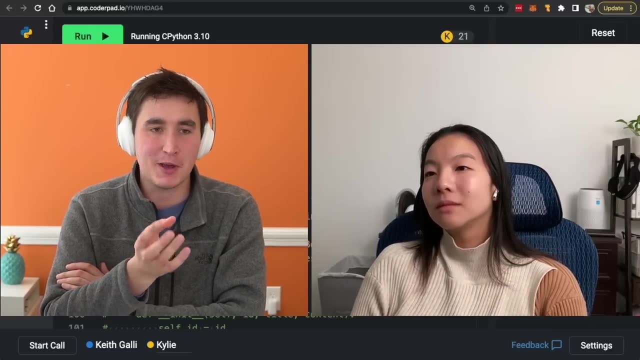 Yeah, it is tricky because you don't have access to that nice library. I think the key thing that you did well with the IDs is that you knew that had to be unique. You didn't want to have collisions And by mentioning like titles might have collisions, that's super important. 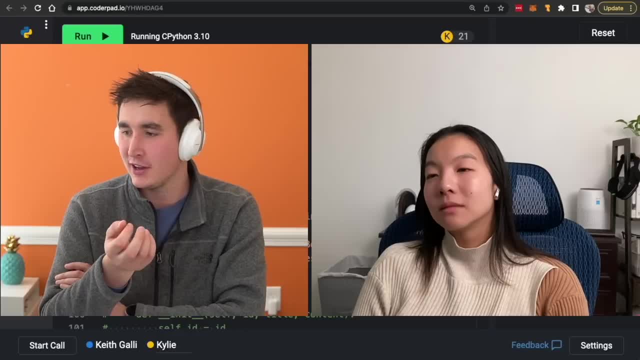 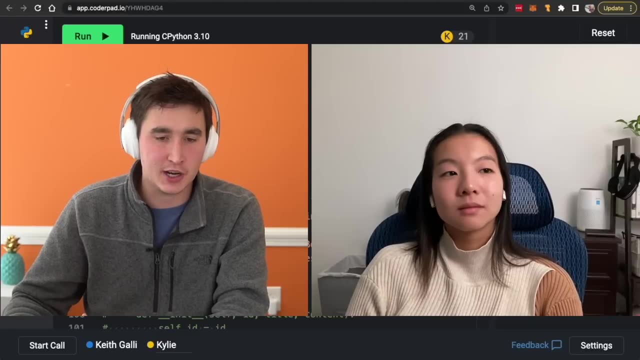 Because that would cause all sorts of headaches for us. Let me see what else I wrote down. I mean again, like I'll reiterate, like this was a good solution, This was a solid solution. This would be like something I'm looking for. 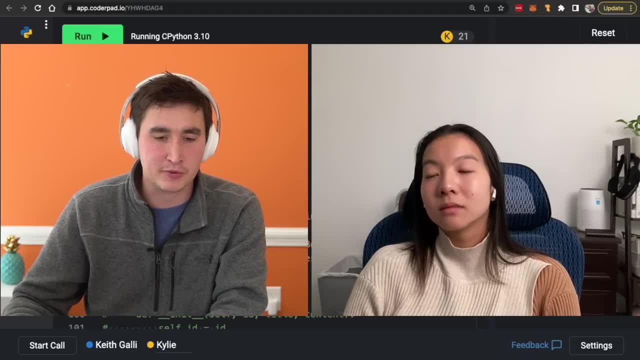 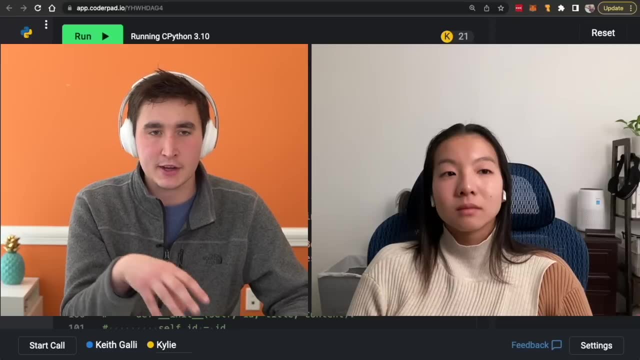 So, like my feedback is more nitpicky and like how could things be improved further? I think another way- and this is kind of similar to breaking things out from, you know, a book class and then a display class- to actually put that onto our Kindle Cloud Reader. 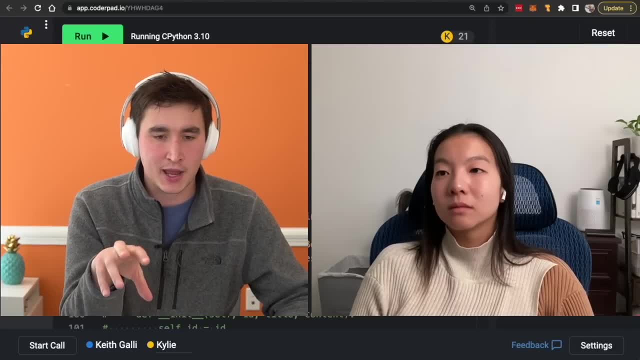 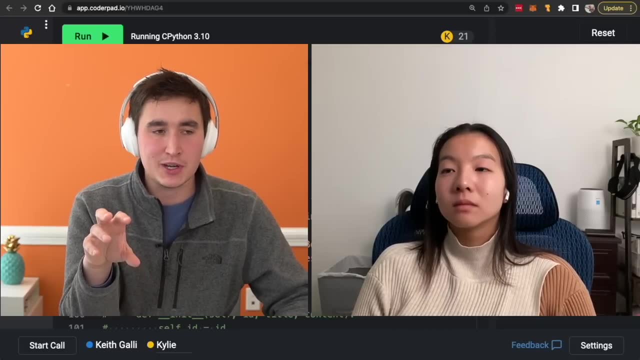 But I think another way you could have. maybe We broke this down in a logical manner. It was when I asked that last follow-up question, which was basically: you know you might have many users in this And now we need to be able to. 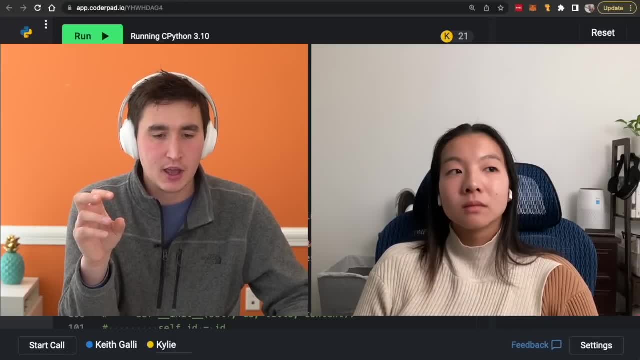 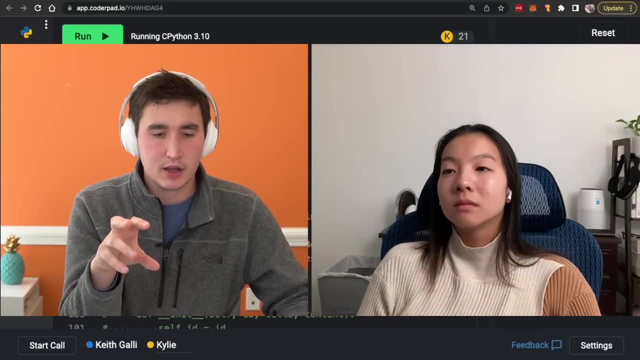 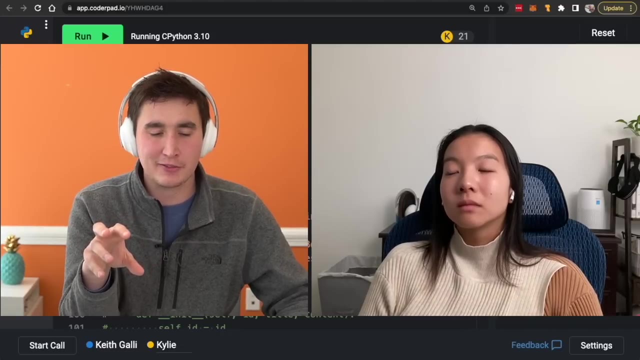 Each user needs to have their own like last page for each book and all that. I think that your answer could have been a bit more nuanced there. I think one thing that you could have maybe mentioned is we could have potentially used, like superclassing, subclassing to maybe have, like you know, 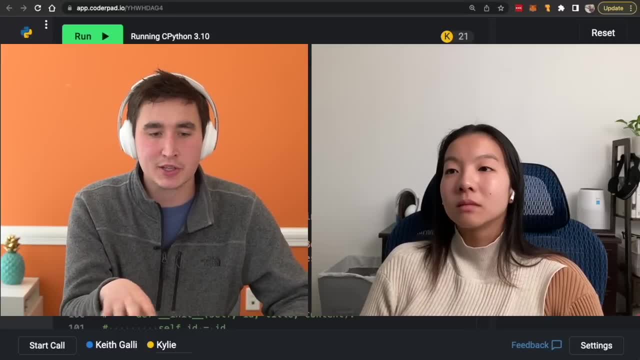 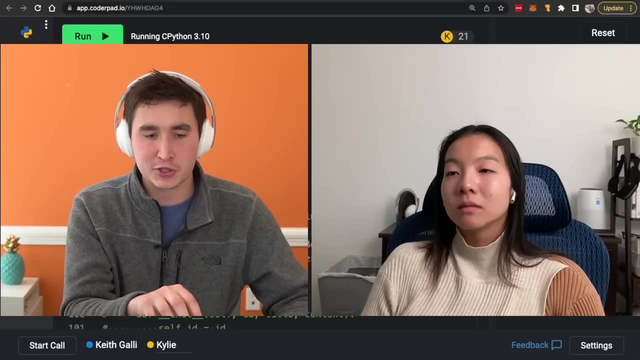 a base book class but maybe there was like a user book class that built off of that class book that you know, everyone shared ID, everyone shared title, everyone shared content, But all of those user-specific things could have reused some of that previous code, but built off of it. 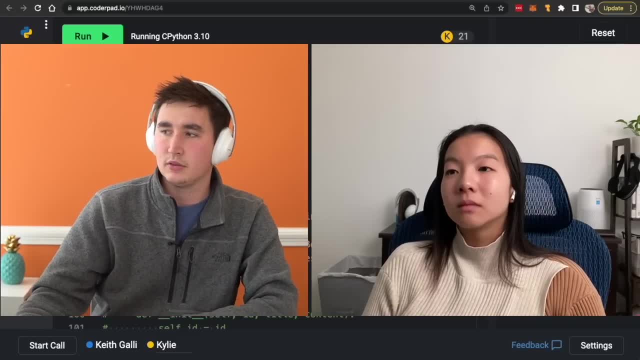 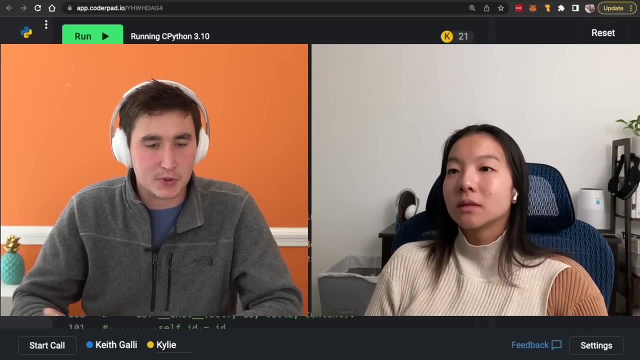 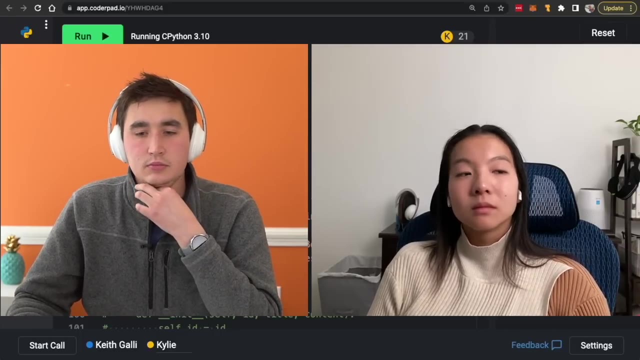 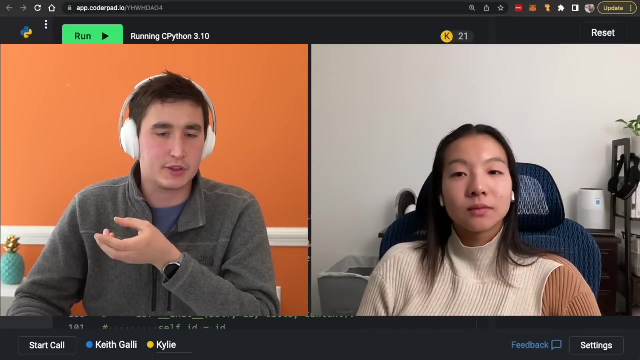 So that would have been an interesting idea too. Yeah, yeah, That's all I have for the object-oriented portion. Any, I guess, other comments on that section Cool, And then, I think, for algorithm solution. I think throughout the interview you did a good job of explaining your thoughts. 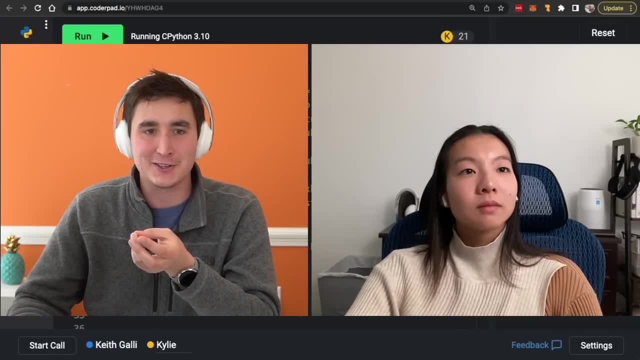 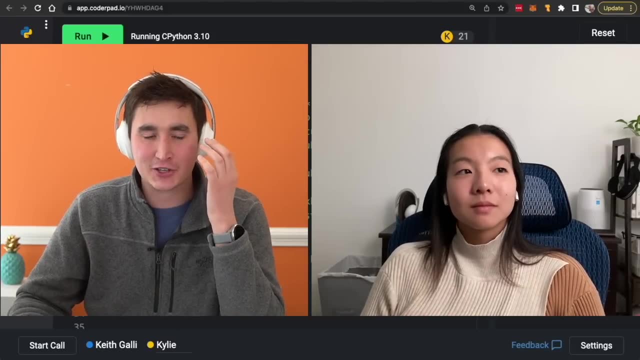 Super, super important to anyone listening to this: Don't just write something down. Talk through what you're writing down as you're writing it. That helps me make sure that I know what you're talking about. That makes sure that I know that you're on the right track or off track. 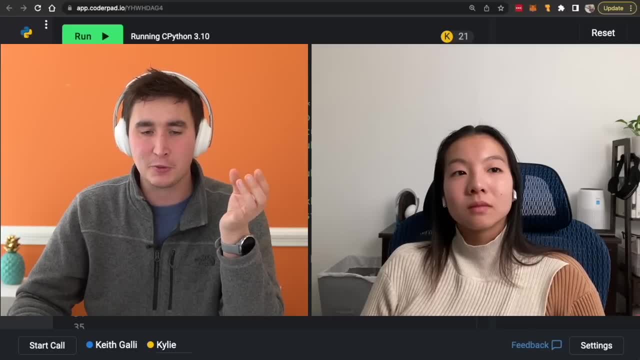 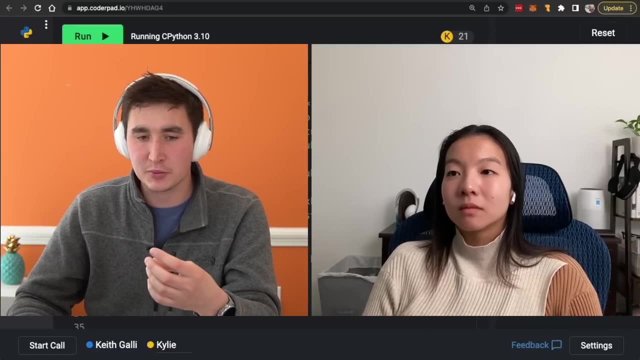 So you did a good job both in the object-oriented design As well as the algorithm, just explaining what you are thinking and the pros and cons. So, like one thing I liked in the algorithm section is, you know, coming up with a very naive solution to start. 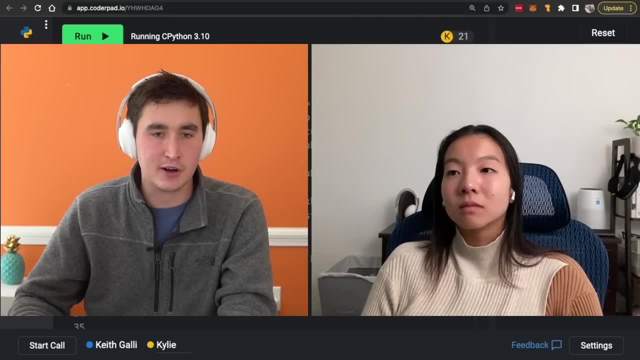 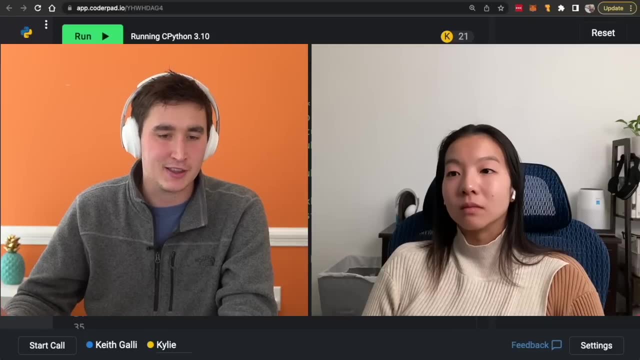 I like seeing that kind of iterative approach, See that you're kind of working towards more optimal solutions. So I liked the idea of using like every single substring in these two but then realizing this is not optimal. I liked then you kind of building and taking that and being like, okay, maybe that's not the best approach. 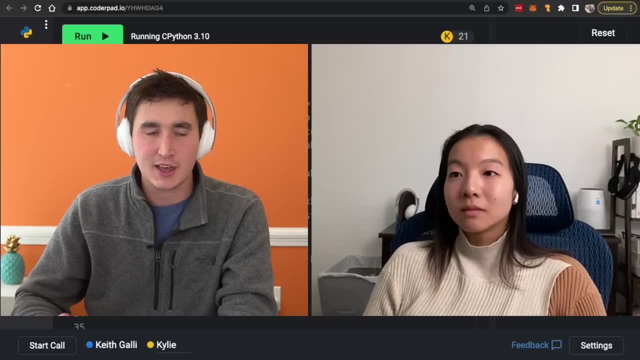 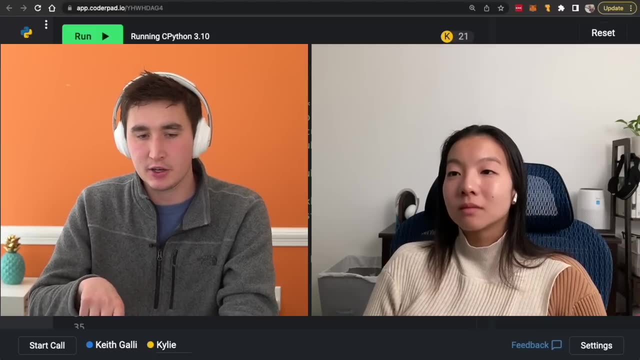 But let's take a base sentence and you know a new sentence and you know, start going character by character in the base sentence and compare it to the you know comparison sentence. I think that that was you know a you know you're working towards a better solution. 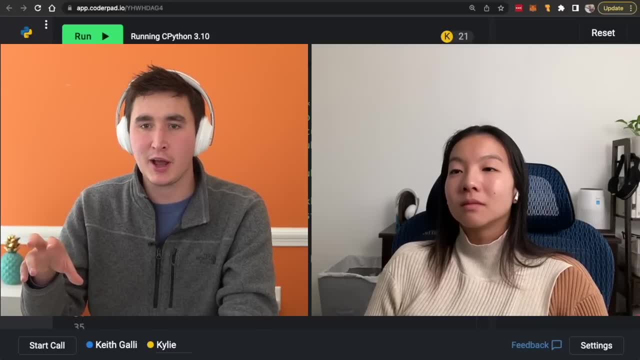 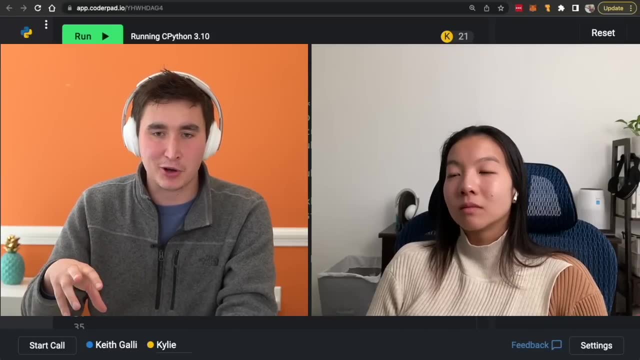 It's going to be better than that. every substring approach, but still not quite optimal, And kind of realizing that there was more improvements that could be made. There was a challenge in how to get to the dynamic programming solution. I think we maybe lost some of those details you wouldn't normally have in class. 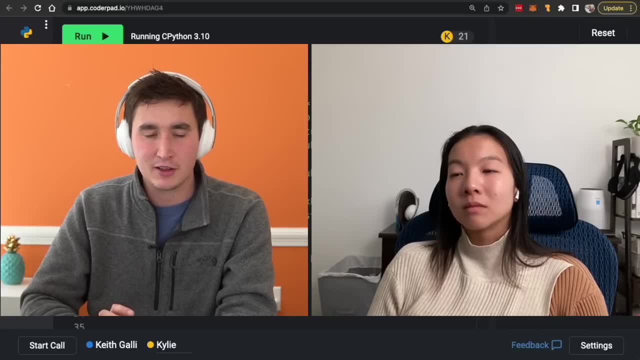 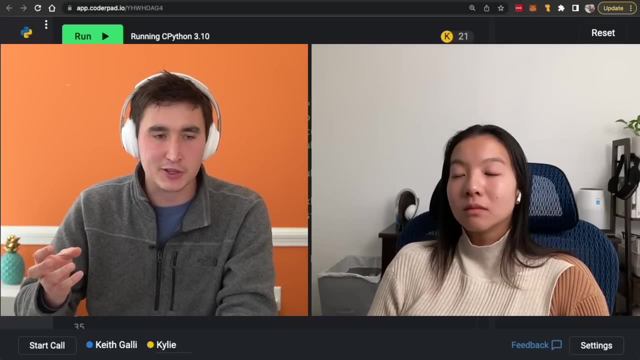 And I think that that would have been really helpful if we had included on like the nuance of this and how you might improve it So like I would have also liked to hear mention not only of verb tense, but also like punctuation, if we have to, you know, keep that in mind. 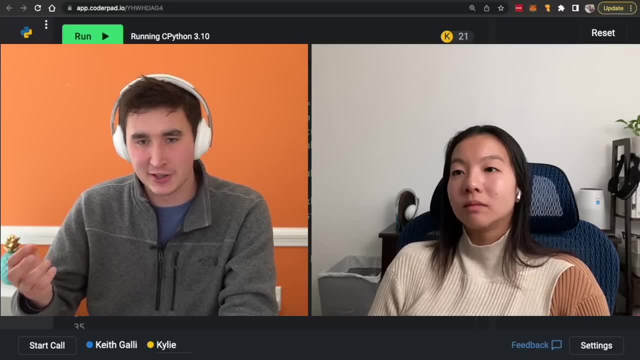 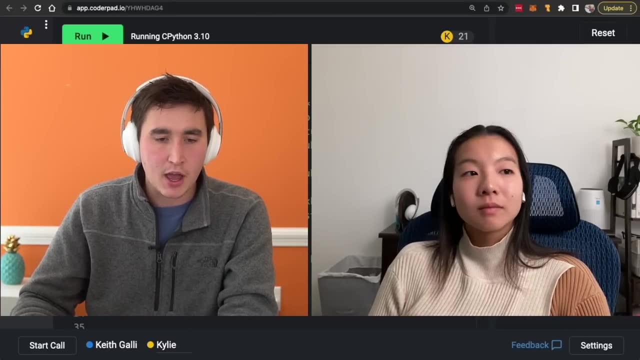 So if someone changed periods, exclamation points, should those still match or should they not match? All of that And then just kind of getting to the dynamic programming. I think this was definitely like a challenge, trying to figure out how to formulate this. 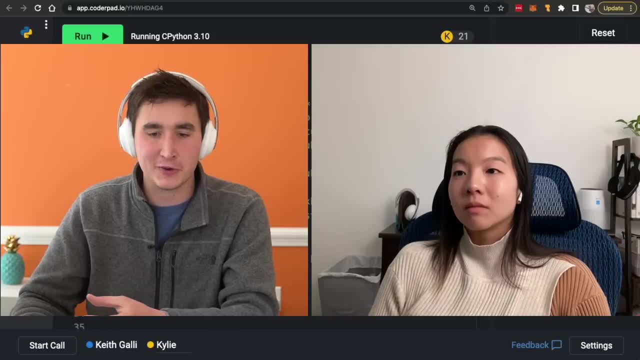 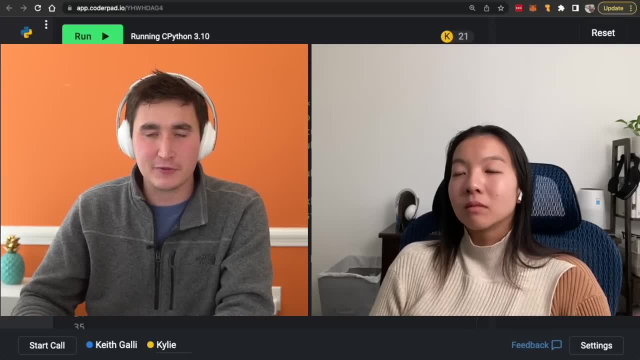 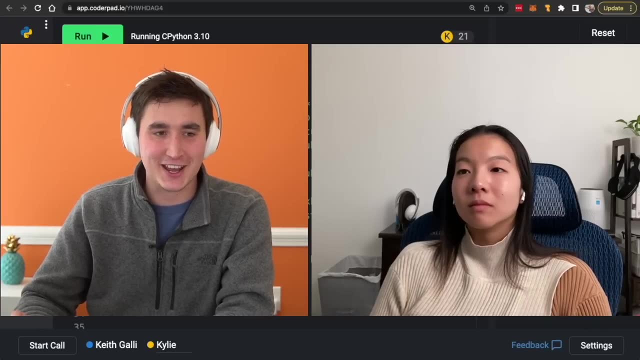 Yeah, Yeah, Yeah, Yeah, Yeah Yeah. You would have had gotten a little bit further without me having to prod, But I think the nature of dynamic programming is, unless you're reviewing it and like, really like studying it and staying on top of it. 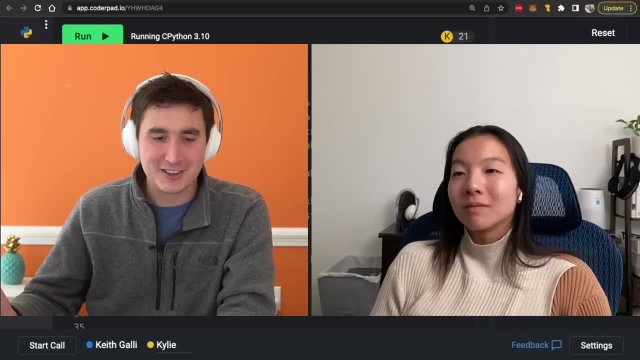 Like in the real world. you don't have to know this type of stuff. You're not coming up and like designing from scratch dynamic programming. You're usually looking at notes and all that. So, like I was, you know I'm okay in an interview setting having to prod a bit. 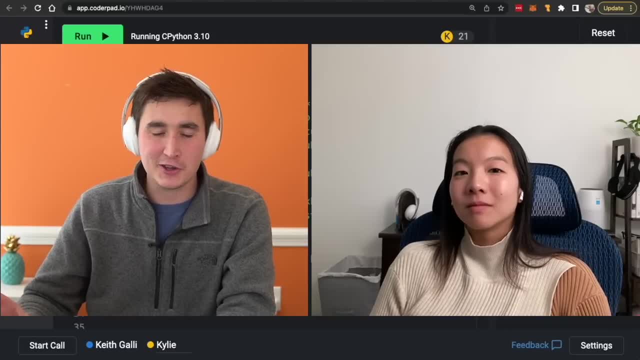 But you know, that's, I guess, the difference between a good interview and a perfect interview. A perfect interview is like the nature is. I had to provide a decent amount of details and kind of help you get to a recurrence. 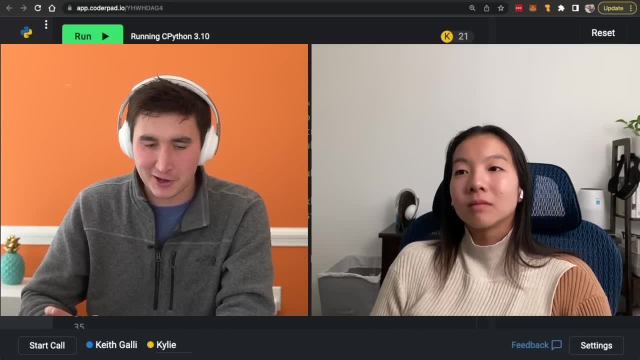 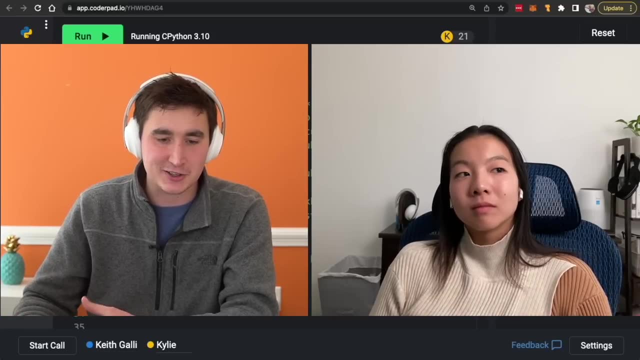 And then once I gave you that starting point, the launching point of the recurrence, you did a great job running with it. That was definitely like the optimal longest common subsequence or substring type solution, with recursion and memorization to help get us to the optimal. 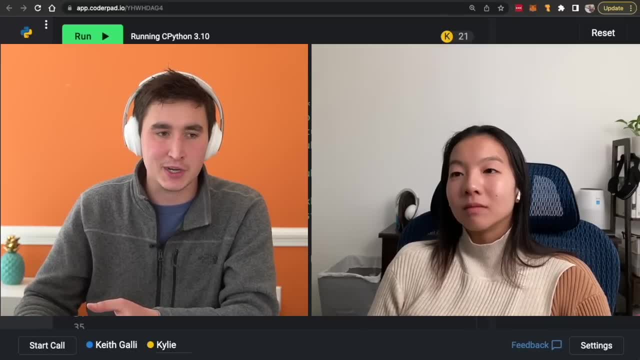 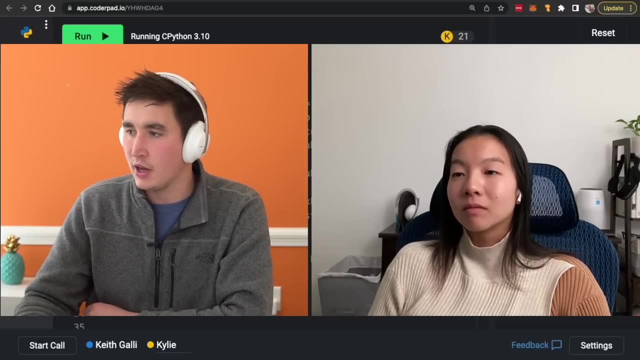 So it was nice to see that, once you had an idea of what we needed to do, that you were able to run with it and knew exactly. you know where you could implement an optimal solution. I think that's all I have. I'm rambling on a bit. 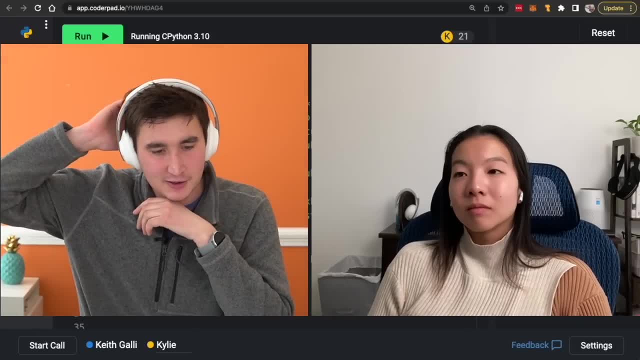 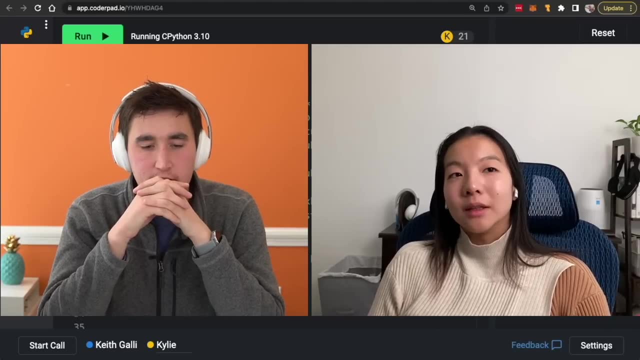 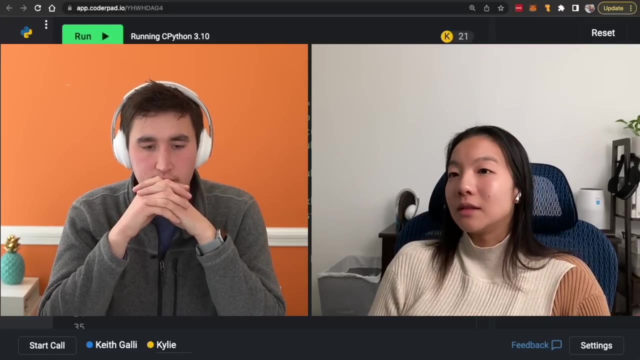 But hopefully those notes make sense and I think we can further discuss. Yeah, I definitely think that this longest substring was a slightly more challenging problem based on, like you know, the problems I've done on LeetCode or like the ones that I faced in, like actual coding interviews. 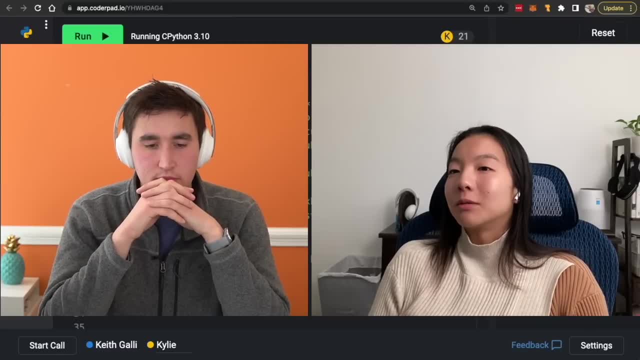 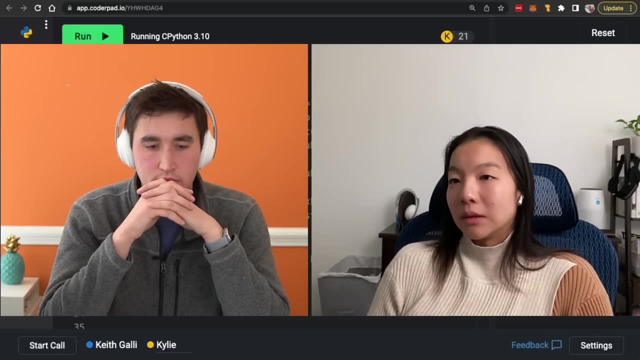 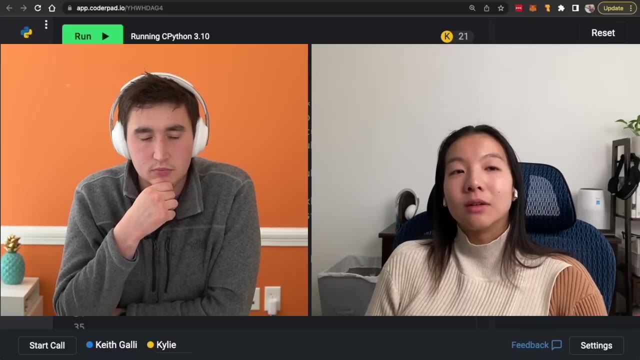 But that's not to say that it's not like a good problem, right? I think it's a really good problem to ask and to kind of figure out you know what are my strengths and weaknesses, And I think that one thing that you know you probably learned from this, is that, okay, you know. 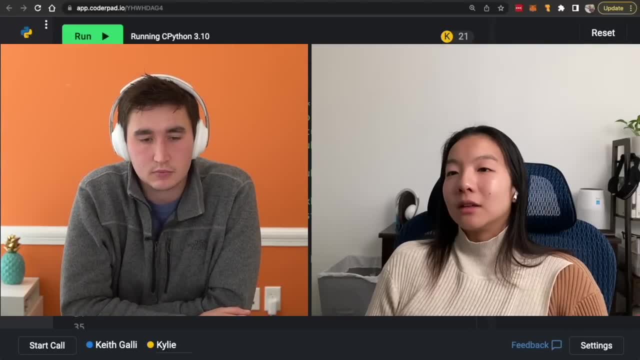 maybe I have certain ideas that are there and I like needed a little push in trying to formulate it properly, But then once you gave me just like a structure to formulate it, then I was able to take that and be able to run with it right. 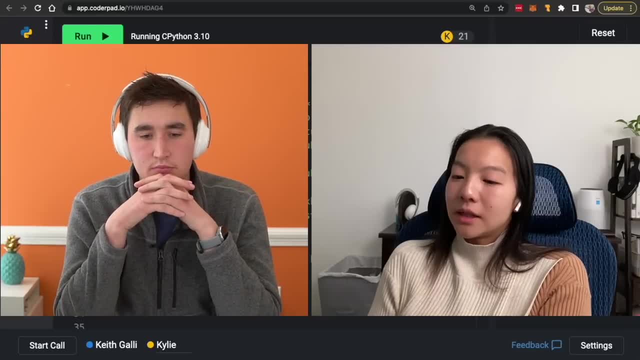 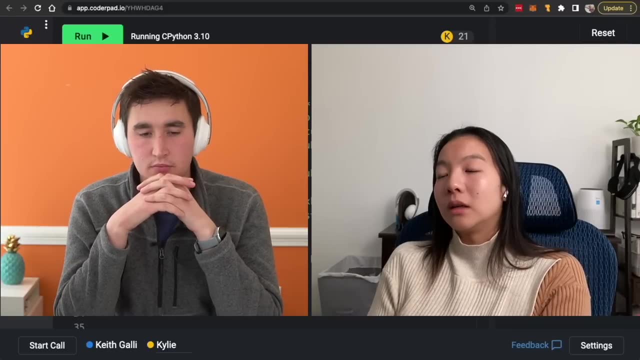 Which I think that you know from an interviewer's standpoint, like when you're interviewing. it's not just about can they do it or not. It's also about how would they, you know, how would What would an interaction with this person look like? right? 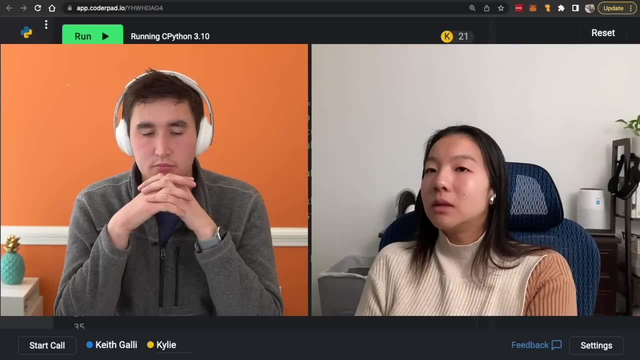 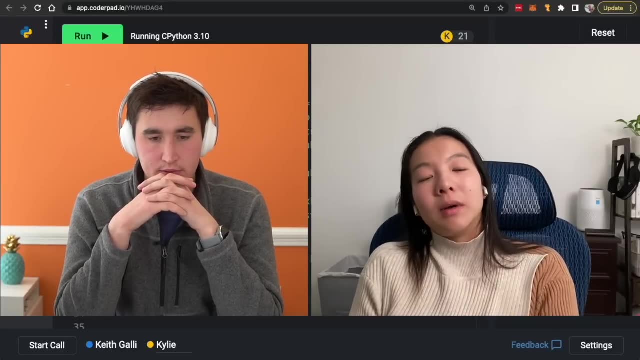 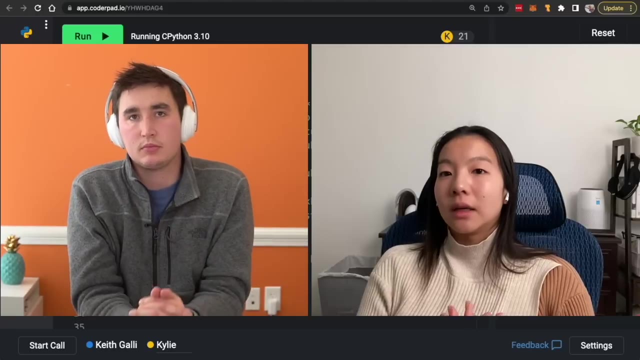 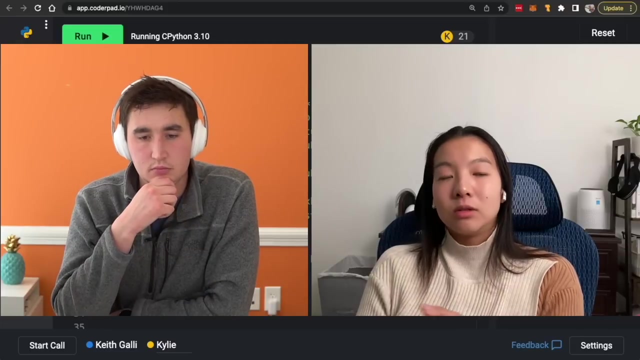 And so, actually, one thing that I really liked about this was that it seemed to be pretty collaborative and it seemed to be very casual, rather than like me taking a test, And so you know What that tells me as somebody interviewing is, oh yeah, like, if I do get stuck, like this person would be able to give me a hint and then I would be able to take that hint and do the rest of the problem. 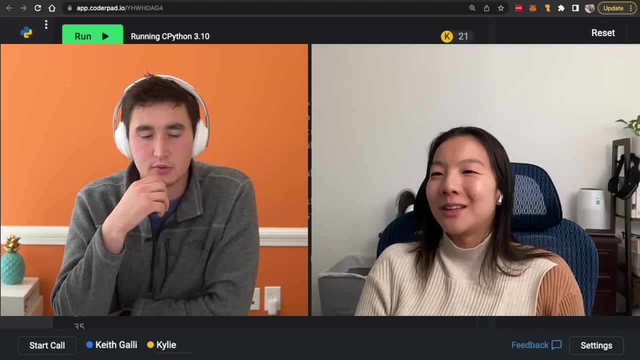 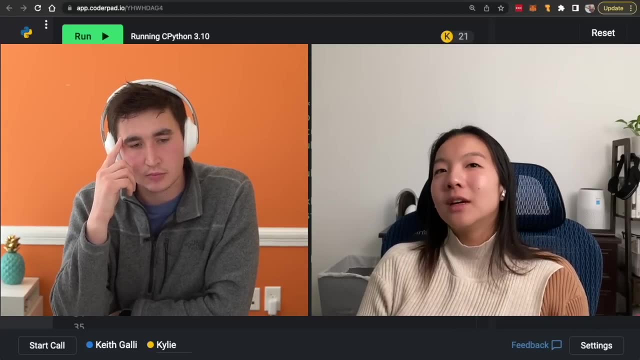 So yeah, I mean I do wish that I was able to just get that and formulate it, But I think that also dynamic programming is typically tricky like that And it takes a lot of It just takes practice kind of, to kind of drill that in. 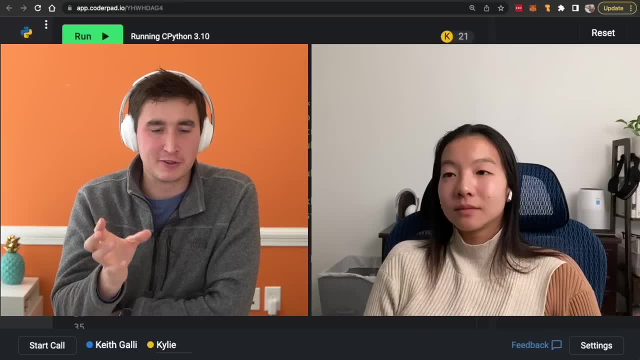 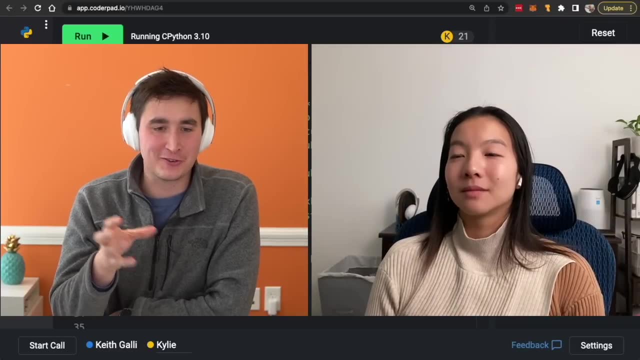 And I think that you make a good point Where it's like this was definitely. the dynamic programming question was a hard question And I think sometimes, once you feel like you're off track in an interview or like, oh shoot, I don't know the answer to this. 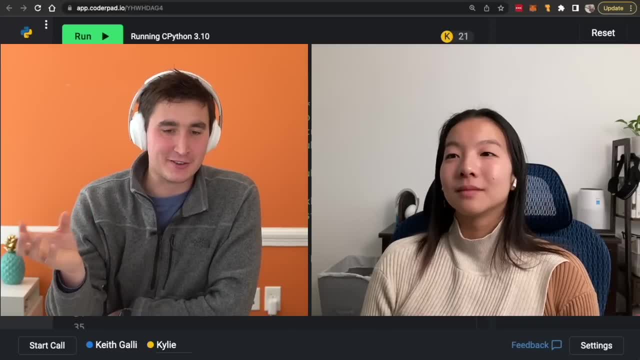 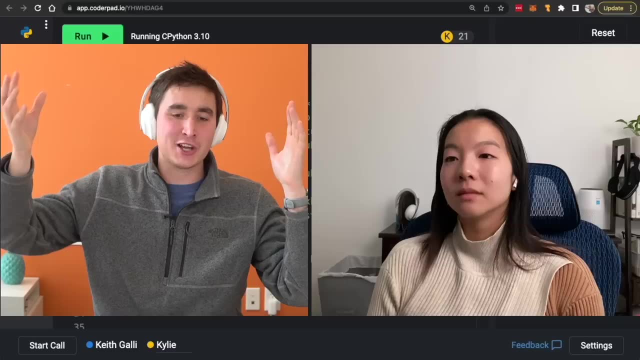 Like I'm screwed, I think, realize that you might be purposely given a hard question because then you can identify a larger range of candidates. So, like you know, maybe the tippy top is like it's instinctual for them to like realize how to solve this with dynamic programming. 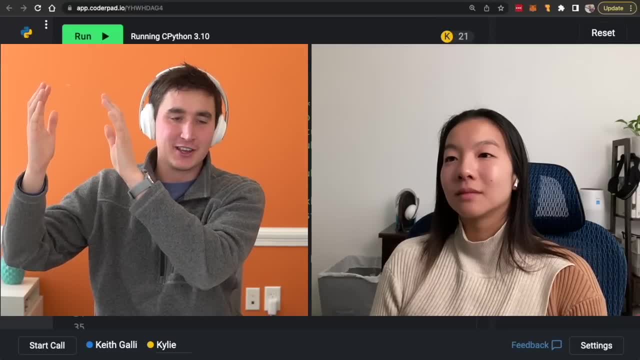 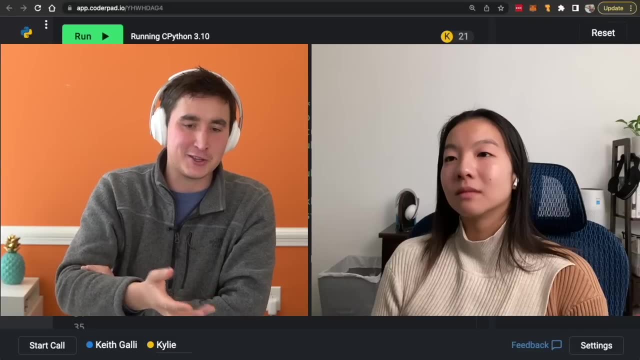 But I'd say, like The strong half of this, they won't know it right away, But they'll be able to work themselves to it. So like, don't get too flustered. This is not to you, This is to a general comment to anyone listening. 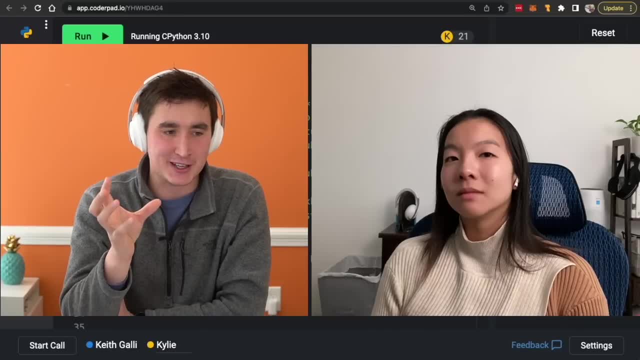 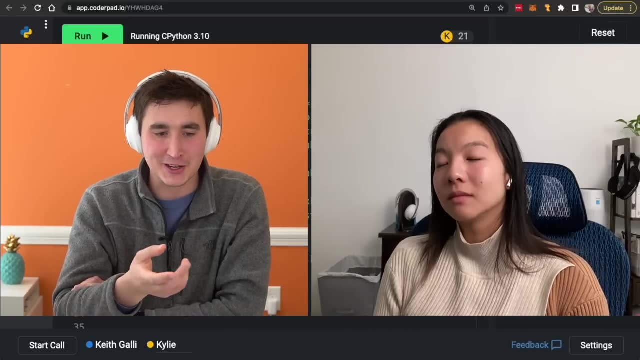 Don't get too flustered by, like, getting stuck. You're oftentimes expected to get stuck. You're human, So you're going to get stuck. It's how you rebound And I think you did a good job mentioning you know you rebounded well. 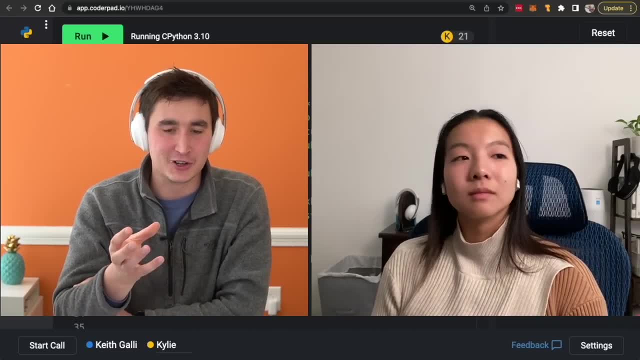 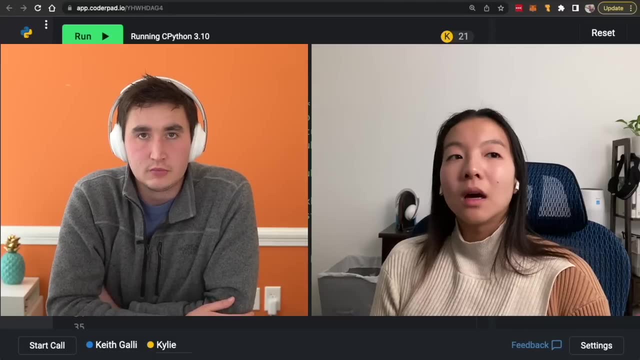 And that's what's important- still like a very strong interview, Mm-hmm, Because you were able to work to the solution and it was a hard problem. Yeah, I will also mention, I think, one other thing that a lot of interviewers do tend to look for is probably testing. 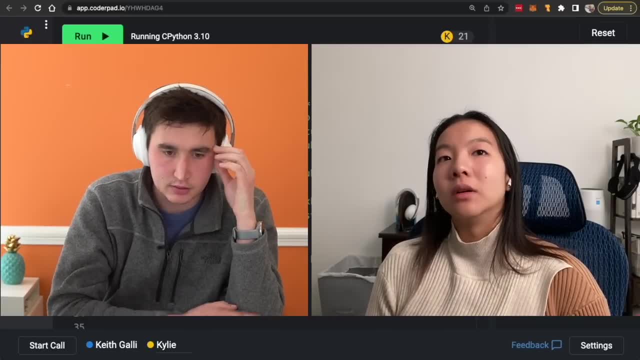 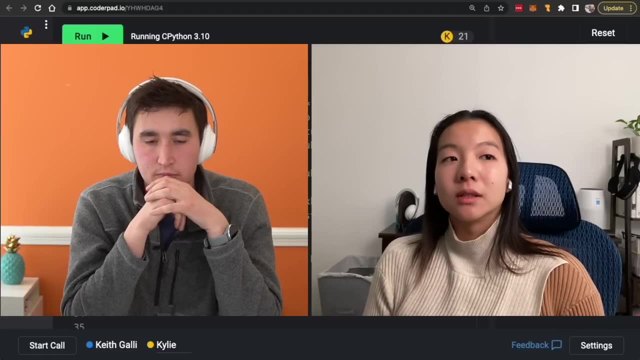 So I do think that, Yeah, You know it's a good signal. You know we were running out of time, But I think for the interviewer it's a good signal if the interviewee brings up testing and says, oh, like you know, I like the solution. 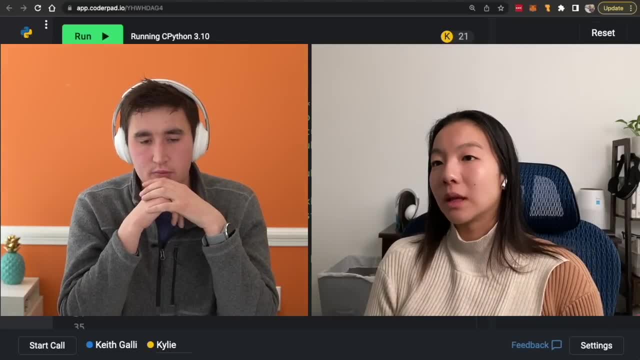 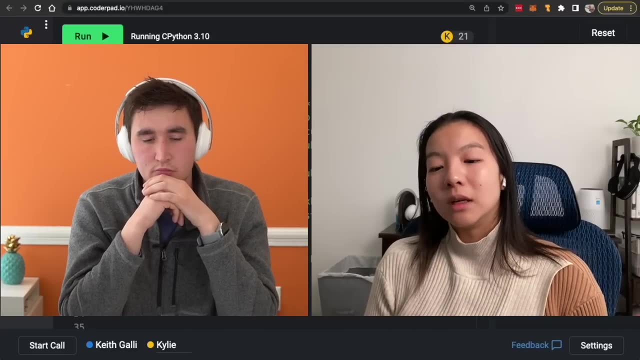 But, in order to verify my answer, I would like to test it Right, I'd like to run it or something like that, And I think, in terms of what the interviewer is looking for, is that they want to see that you're going to be a good software engineer. 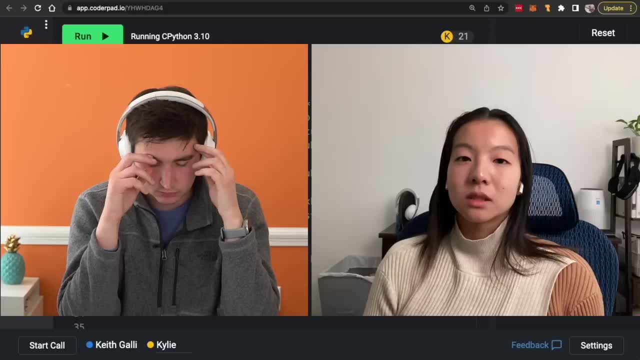 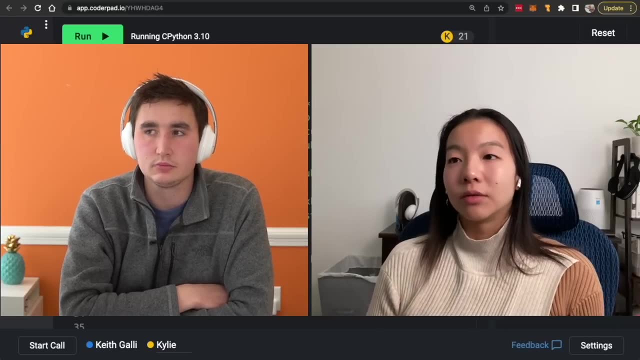 Right, And I think testing is a big part of that equation, And so I think that just mentioning maybe, hey, like these are a few cases that I would have ran through if I had extra time, Or you know, here are some of the edge cases. 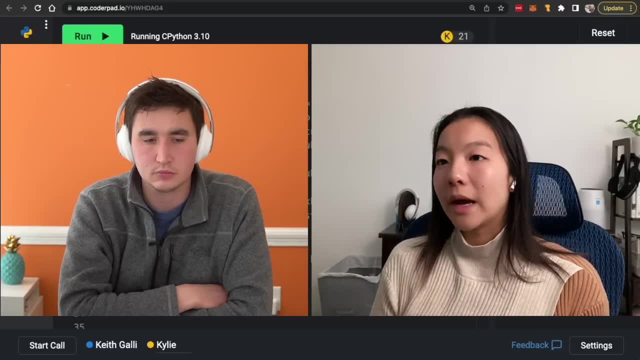 Like I think this might work. I think this might work for most cases, But there might be some sort of edge case here and there that I should have like gone through. I think those would be No, that's a great point. 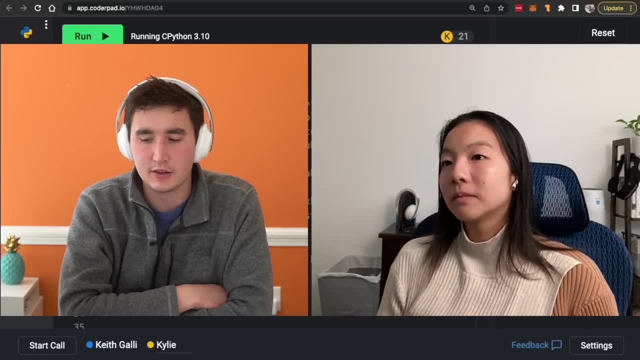 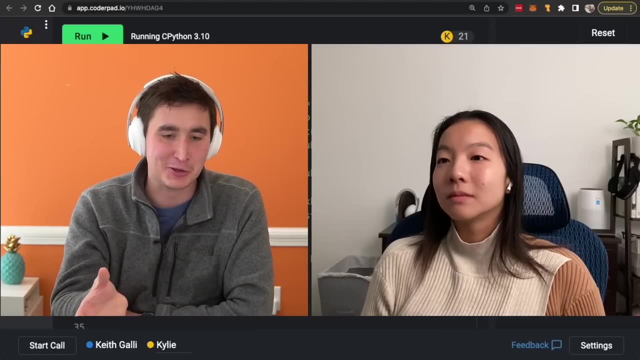 That should also be a component that you mentioned. The testing is super important. So seeing that- And it is challenging because we did kind of run out of time- So like I feel like you didn't hit some of those things that you probably would have hit if we had all the time in the world. 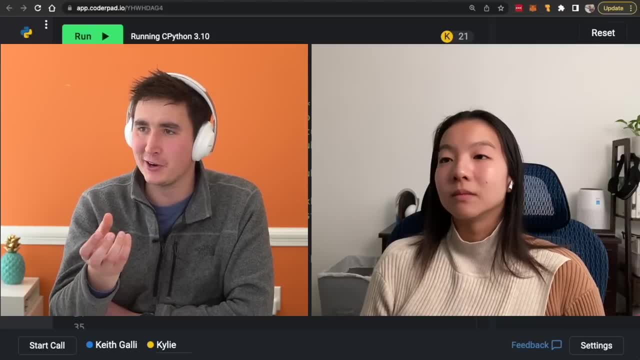 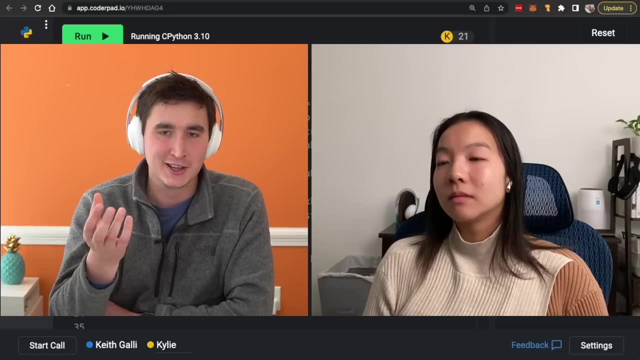 One thing that's interesting. I saw this on Twitter or LinkedIn as an idea. I don't know what your thoughts are on it. I think that it is pretty solid. I would kind of be impressed if a candidate did this, But I could see it going either way. 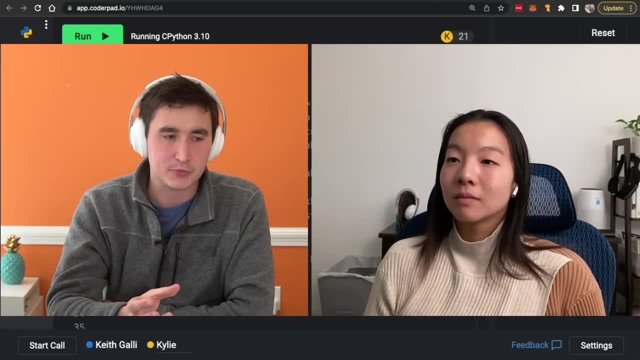 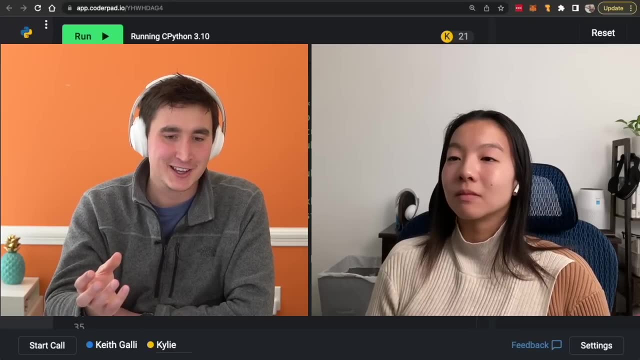 Someone mentioned they were like a data analyst at Google And in the interview process like they screwed up, I think, a couple queries, a SQL queries, And after the interview they, like you know, calmed down. 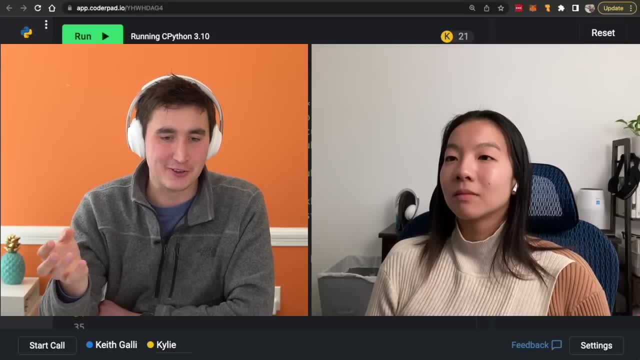 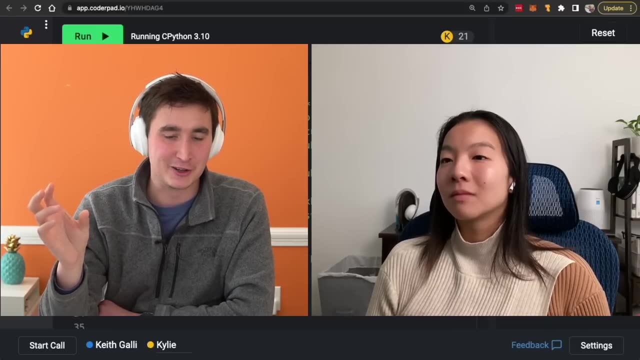 Like they collected their thoughts And they like emailed the interviewer, like the solutions, Like, oh, like I goofed up there, This is how I would have solved it. I, you know, had a little bit more time. 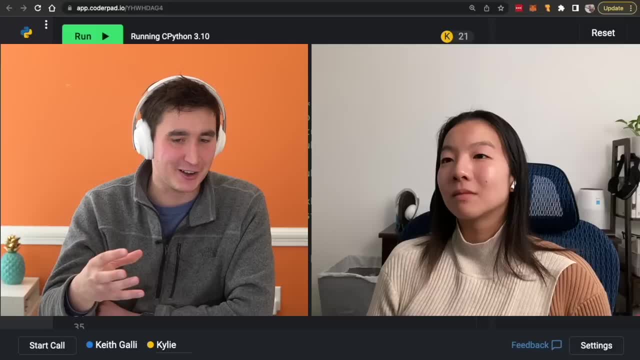 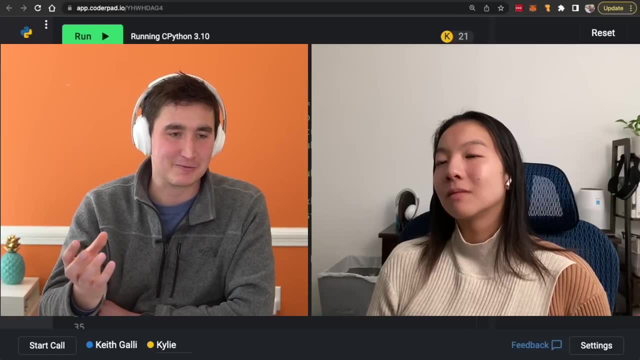 They followed up with, like, some solutions. So it would be interesting. I don't know if you think it would be a good idea or a bad idea. I could see it going over either way. But to like follow up and be like, oh, I didn't get to mention these testing cases. 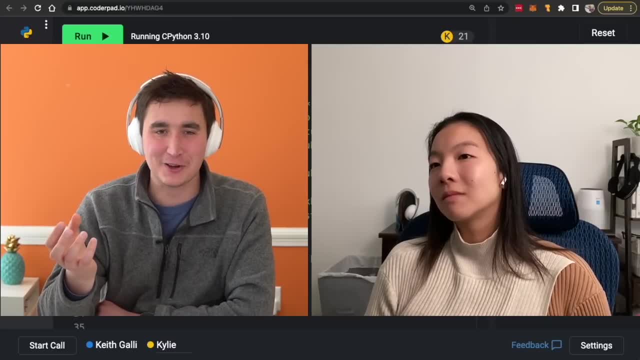 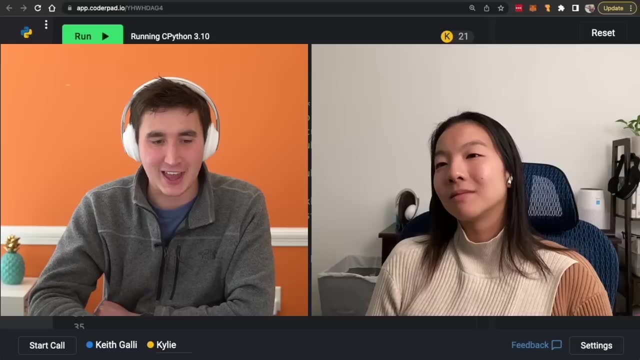 This is what I would have done. I think it's probably situation specific, because it could be kind of weird too. I don't know. I'm just throwing that out there as an interesting avenue, if you feel like you wanted to redeem a bad interview. 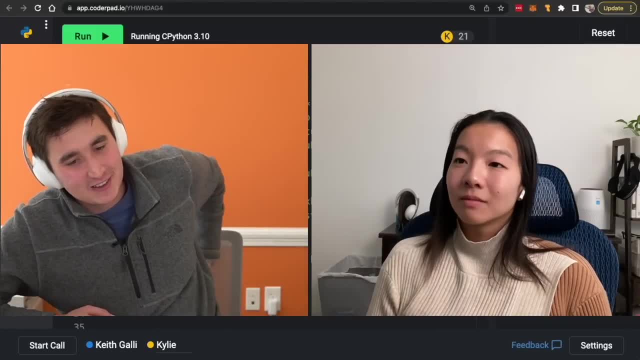 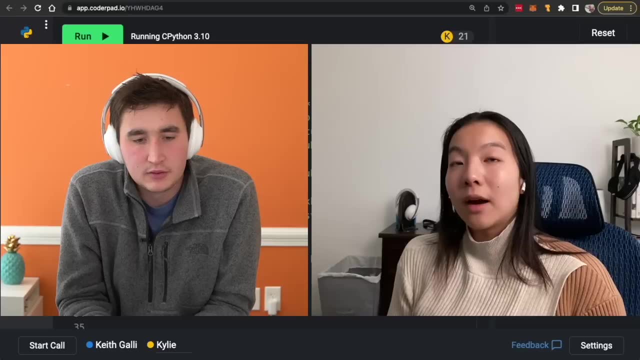 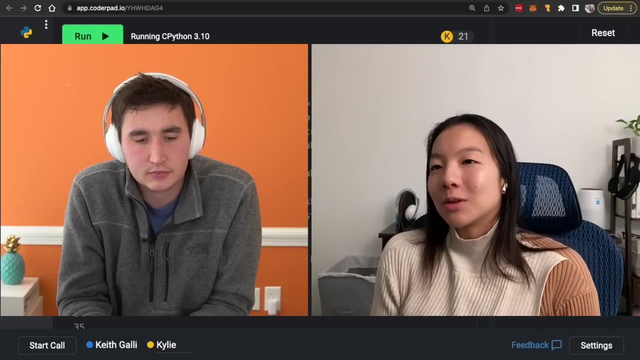 Or something like that, And like have some saving grace, Yeah Well, I definitely do think that that is like. I don't think it's necessarily, I don't think it would be a bad idea under any circumstance. I think that, okay, maybe your interviewer would never see that. 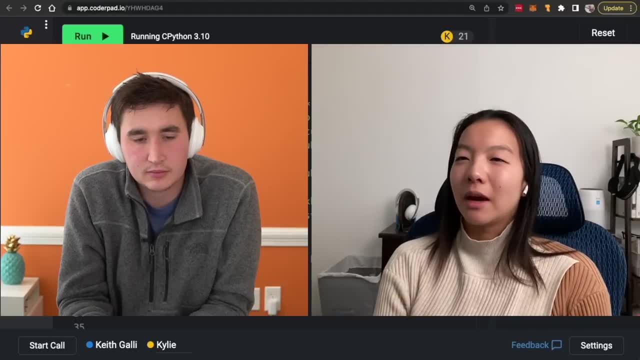 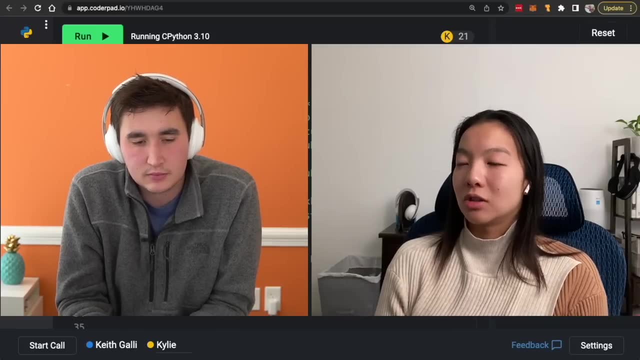 And they find it a little bit strange. Or maybe they've already submitted their, whatever. But I don't think it can hurt And, if anything, I think it shows dedication And it shows That you know you couldn't solve this problem. 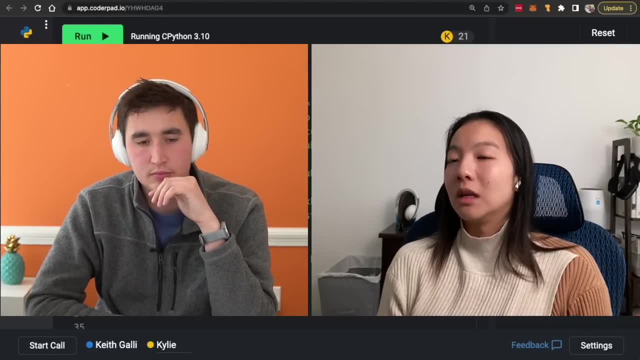 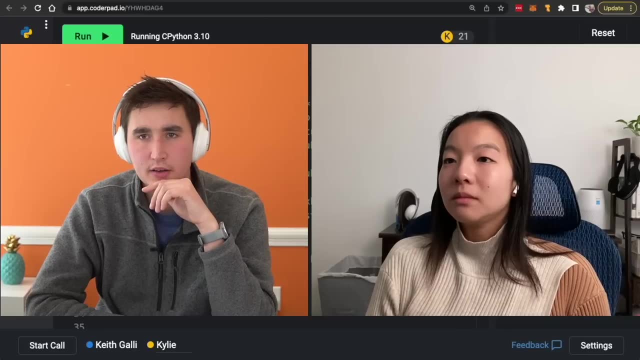 But you took time And you thought about it some more And you didn't give up And then you did come up with the right solution And you followed up and communicated that. Yeah, I think. yeah, it's situation dependent. 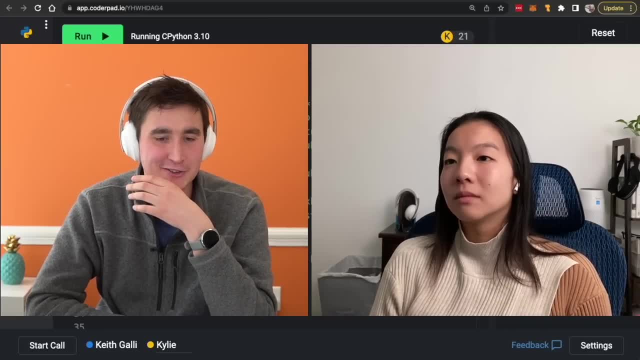 If I felt like my interview went great, I probably wouldn't feel like the need to do that. But if I feel like, oh shoot, I'm so much better than that, At that point it can't hurt to do something like that. 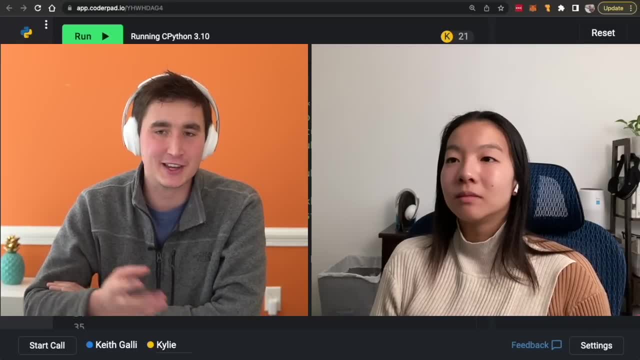 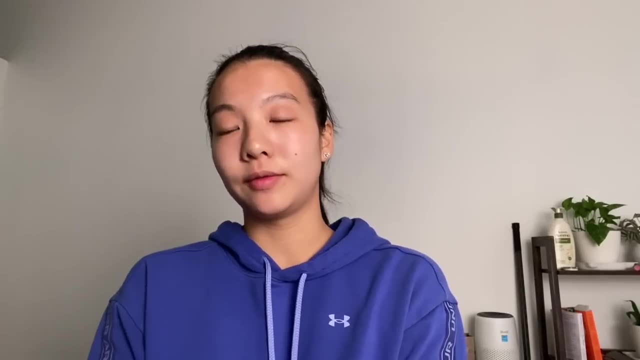 And just keep it casual, Keep it like: hey, Yeah, Yeah, Yeah, I thought of this. Thanks again for your time. Yeah, Take care, Like Okay. So now after the interview, I just wanted to follow up with you guys. 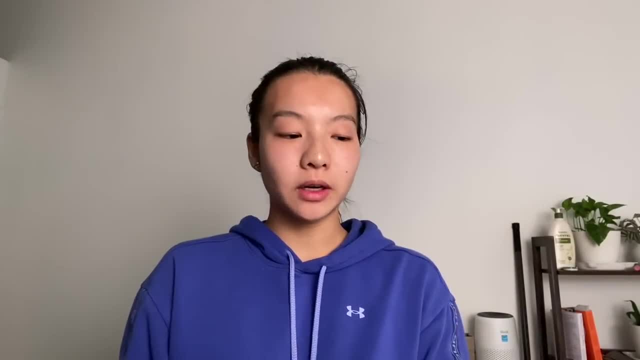 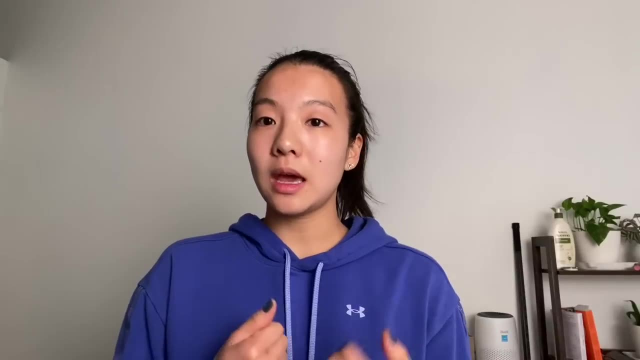 That interview. if I walked away from it I would have been like all right. Well, there are certain aspects that you know, just like Keith said, there are certain aspects that signaled, you know, I was probably a strong candidate. 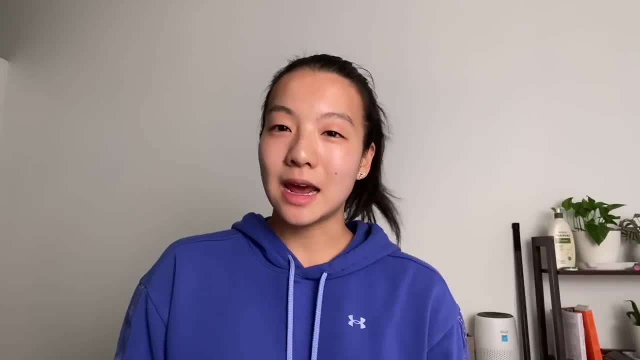 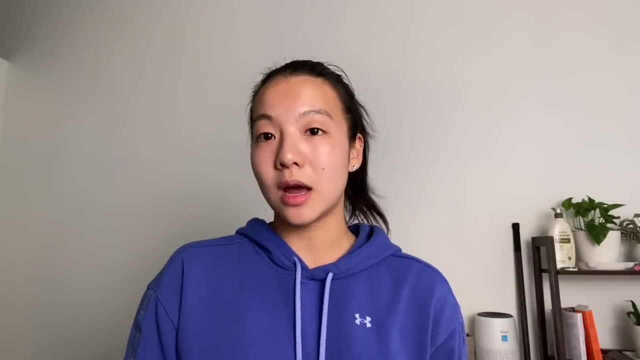 But I personally would have walked away from that being like dang. there are some parts that I probably could have done better on, Like I needed his help a little bit. I probably could have, you know, eventually gotten it if I just had a bit more time to think. 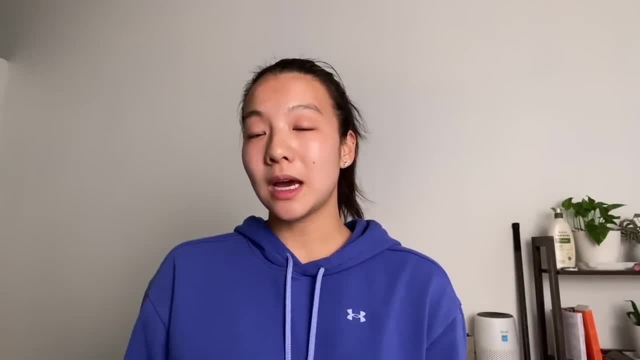 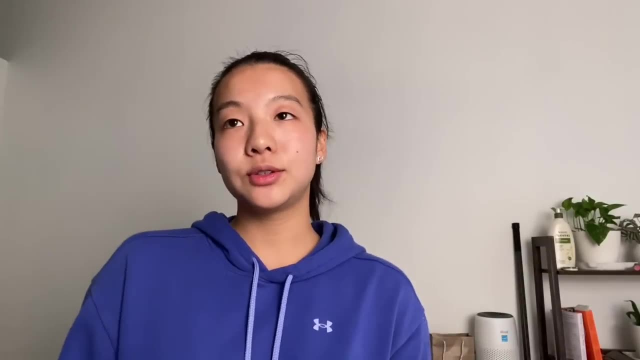 Or maybe today was just not my day And that's just sometimes how these interviews go. You can't do perfectly on all of them. Now a few notes about my implementation specifically, I use pseudocode because Keith, the interviewer, specifically said it was okay to. 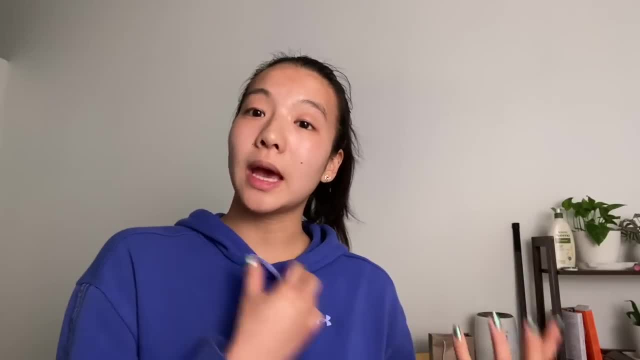 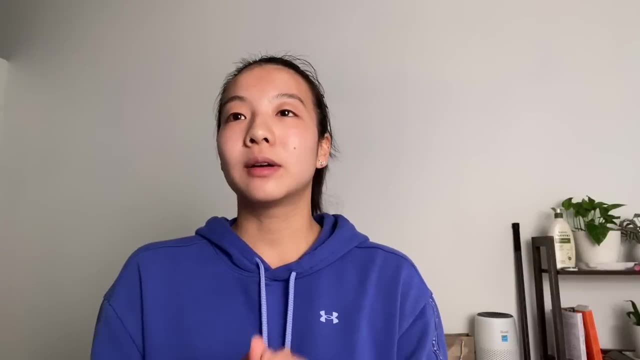 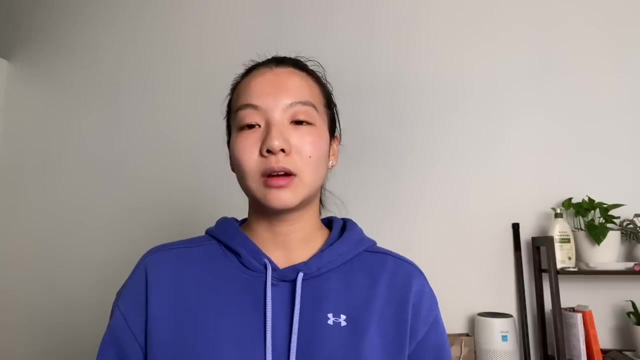 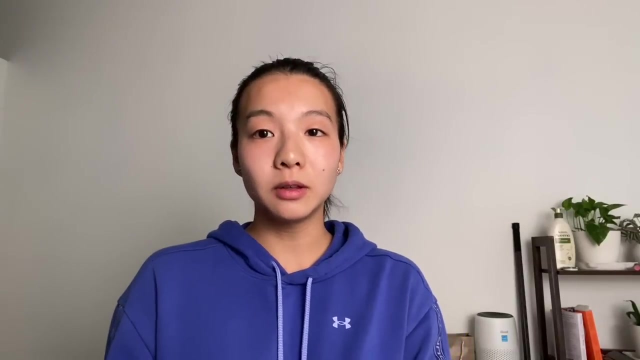 And in this specific problem I really wanted to focus on the algorithm and not really kind of get you know, get into the syntax of things, And so for me Python is almost basically pseudocode. so most of it was very Pythonic, but I commented all out because I was too lazy to get that max part working, because I wrote like possibility three if applicable, and I was just a little bit too lazy to like actually, yeah, implement that. 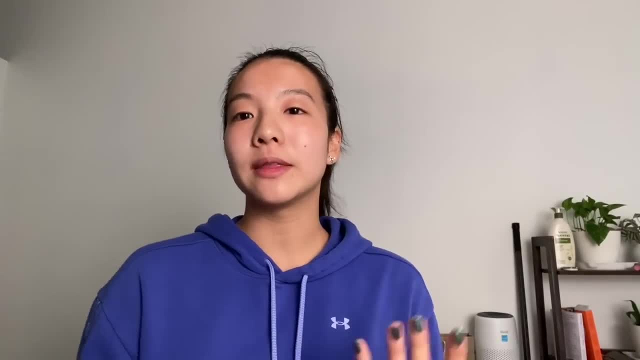 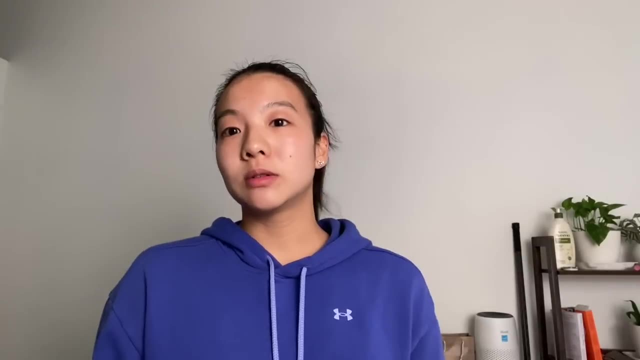 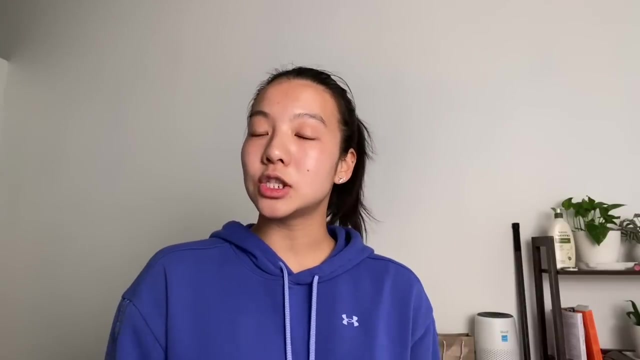 And then also there was some underlining that just wouldn't go away and that was really bothering me, so that's why I also just turned it to an entire comment. Now, some things to remember. There are some things to remember about interviewing in general. so don't be scared to ask questions. turn the interview more into a conversation, because that also gives the interviewer a signal of this is what I'm like as a teammate. 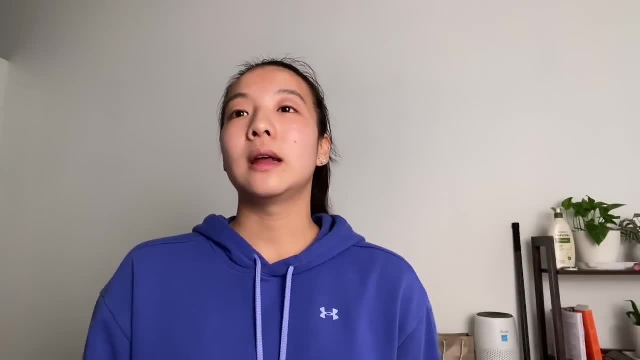 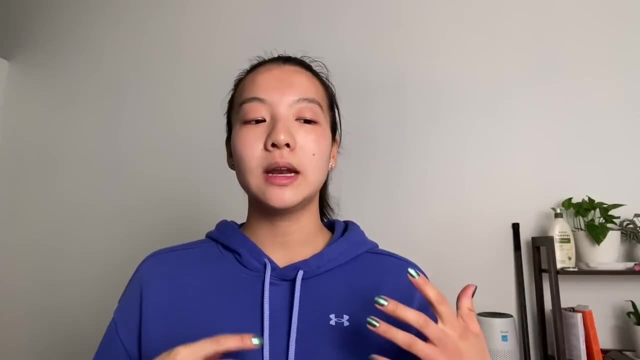 This is what it's going to feel like when you're working with me Now. during the interview, I would always recommend repeating the question to the interviewer, just so that you can check if you actually understood the question and then, from there, maybe even ask clarifying questions. 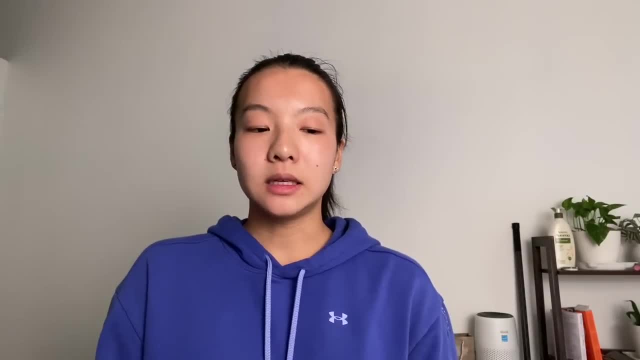 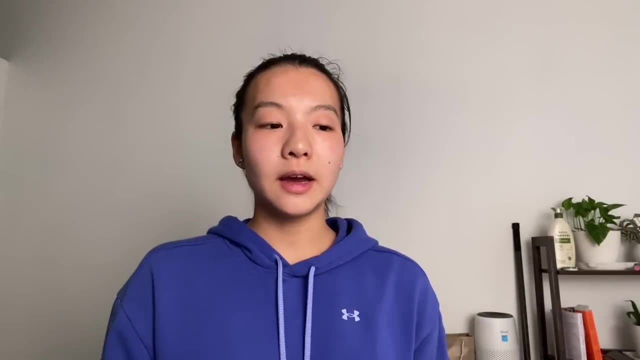 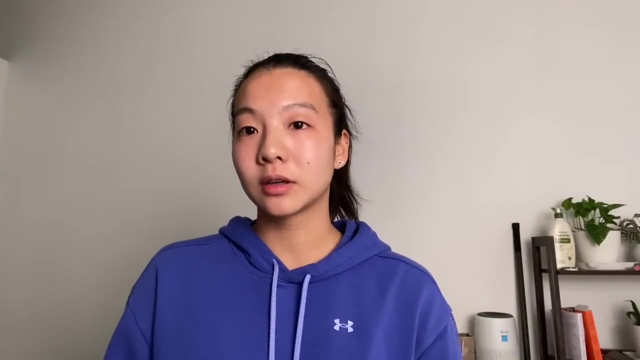 And I typically start with something known as the naive solution, which is: this is the first thing that I thought of and this solution would work, but it's kind of this very brute force solution where it might take a lot of time and it might not work.